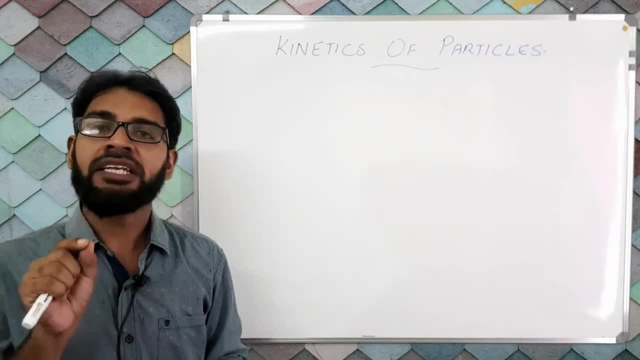 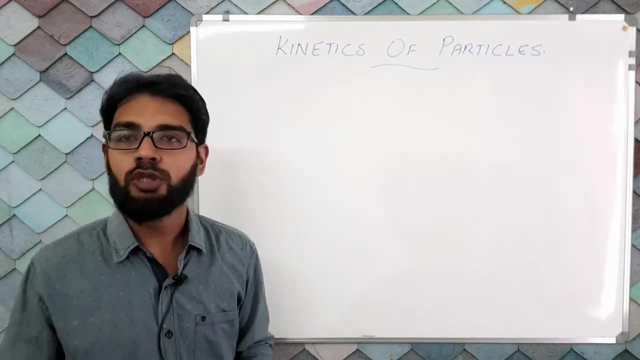 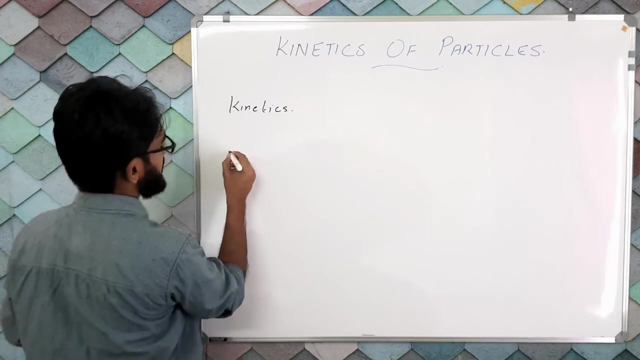 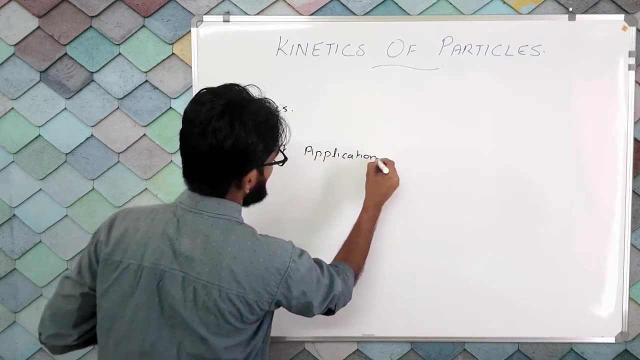 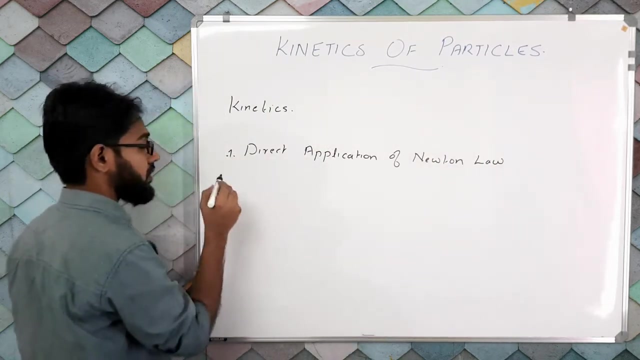 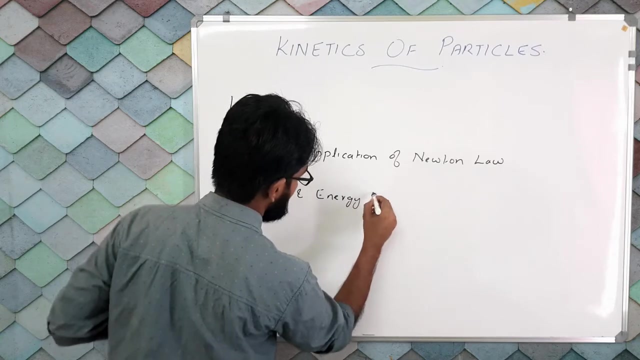 we identify the unbalanced forces acting on a particle and relate them to the motion. Now there are three methods or three approaches to study kinetics. First, the direct application of Newton's law, which you must be familiar with. The second one is work and energy principles. 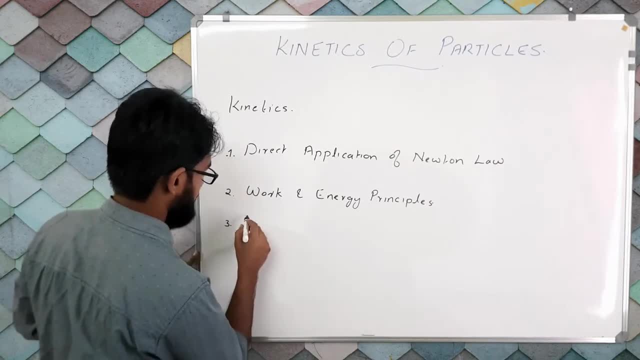 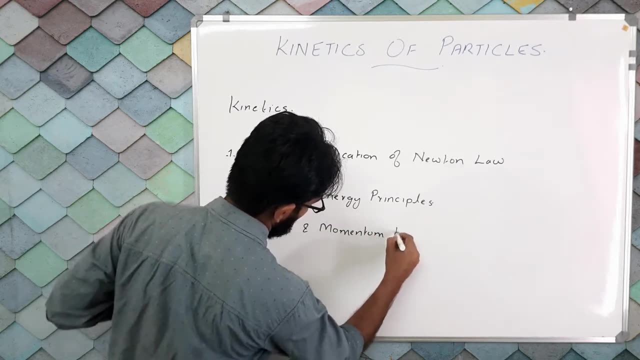 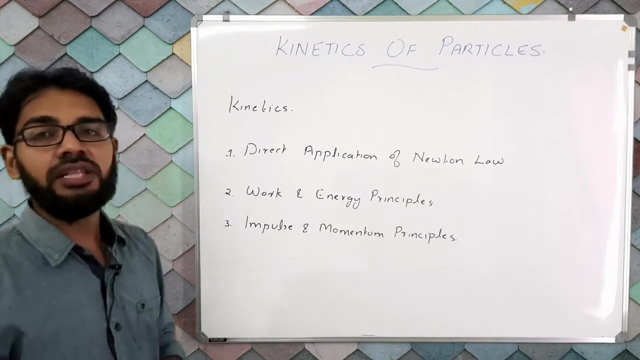 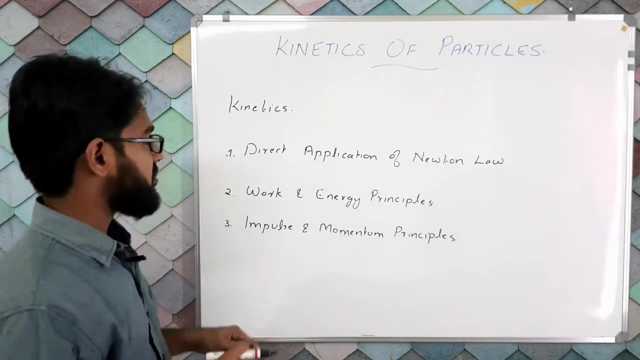 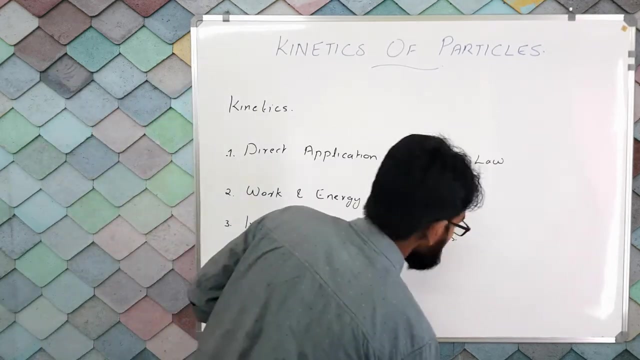 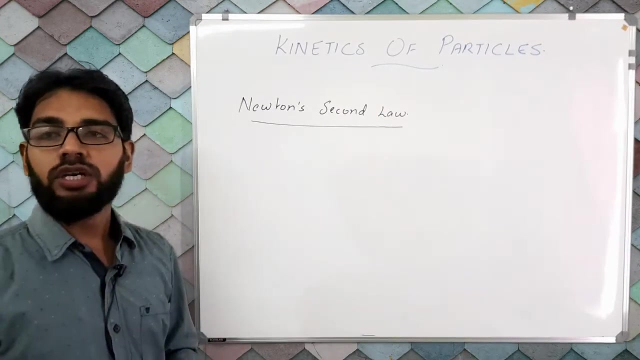 And the third one is impulse and momentum principles. Now these are the three different approaches by which you can solve problems on kinetics. Now, in the next few lectures, we shall be focusing on the direct application of Newton's law. The Newton's second law is one of the most important laws you must have studied in your 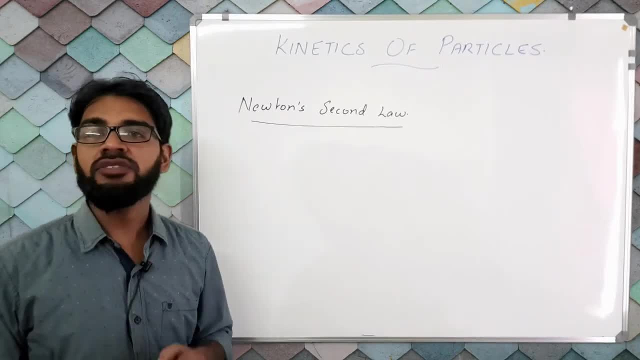 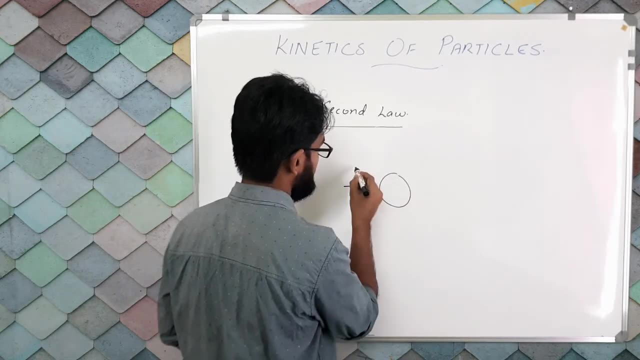 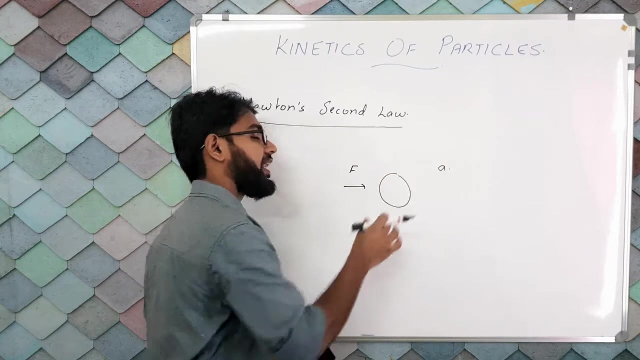 higher secondary classes. Now the basic relation in Newton's law is between force and acceleration. So, as such, if I have a body and I apply some force, I can measure the value of acceleration. We get a relationship between force and acceleration. Now the Newton's laws have been. 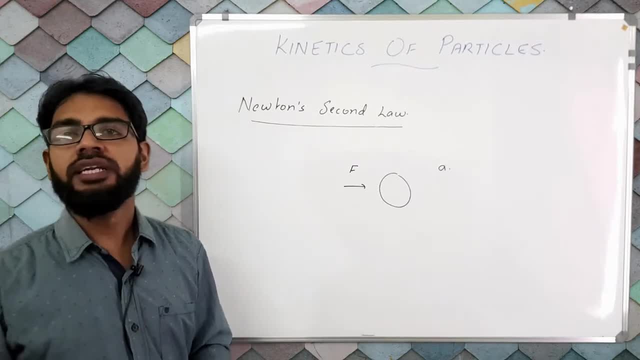 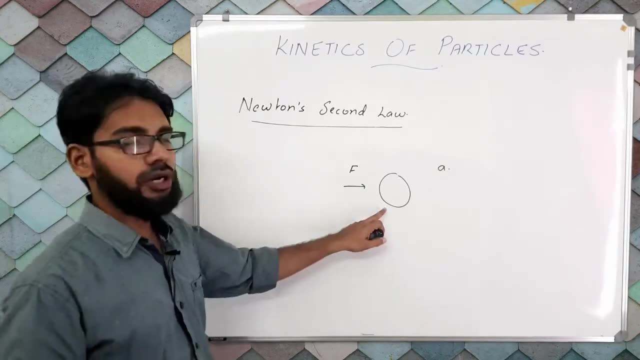 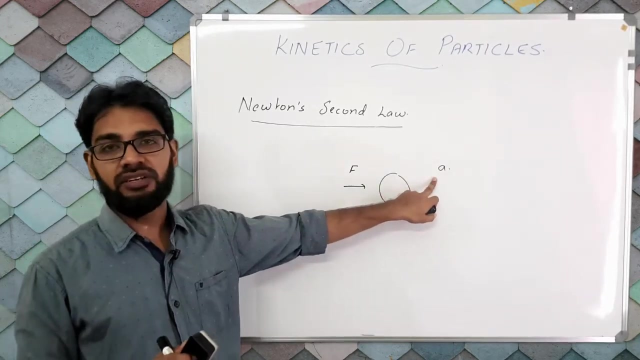 analyzed and experimentally proved in different ways. So let's get started Now. how do we prove the Newton's law? Now take a body, for example, of significant mass. Apply a single force and measure the acceleration. Repeat the experiment with different values of. 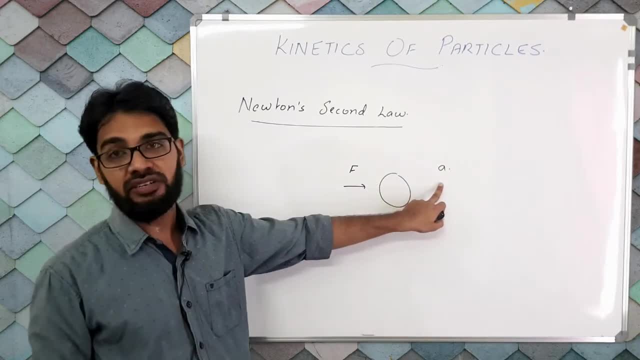 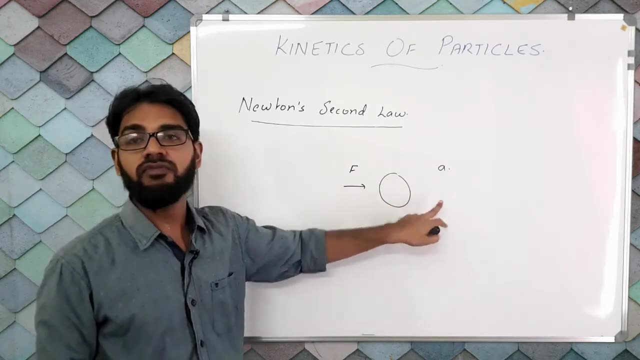 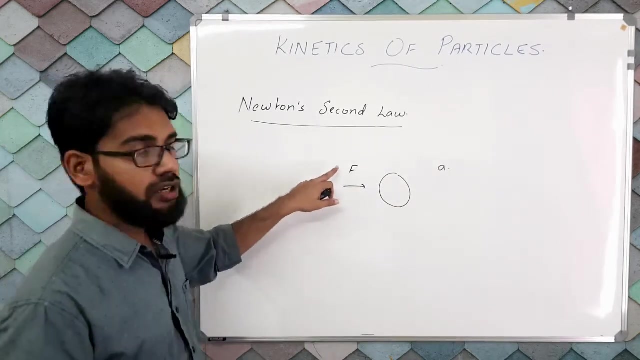 force and in each case, measure the corresponding acceleration. You must remember one thing is that you must be able to measure both the force and acceleration without much error. Now, if you look at the results of these, you can observe that the ratio of force to 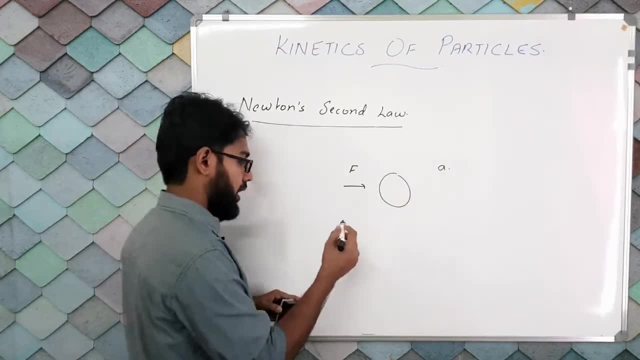 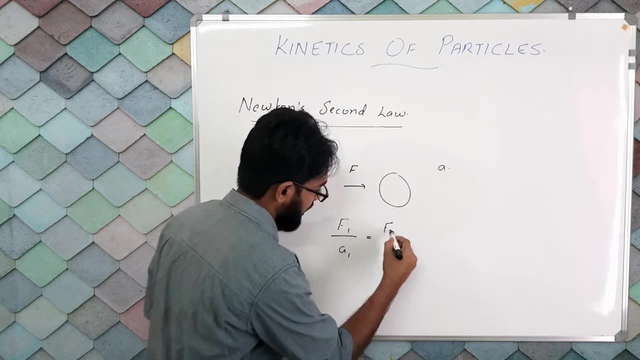 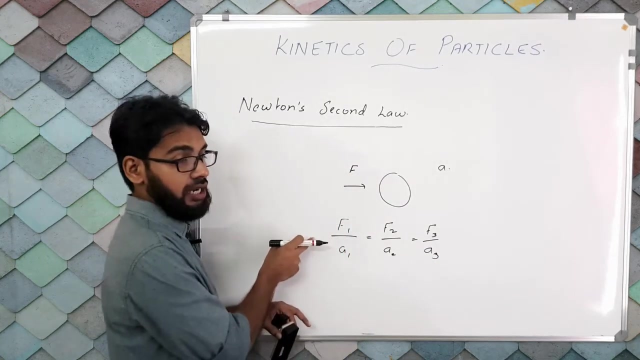 acceleration is always constant. So if I have a number of forces and if I measure the corresponding value of accelerations, I would get: F1 by A1 is equal to F2 by A2 is equal to F3 by A3. These are all for a single mass m This will seem to have a constant value. 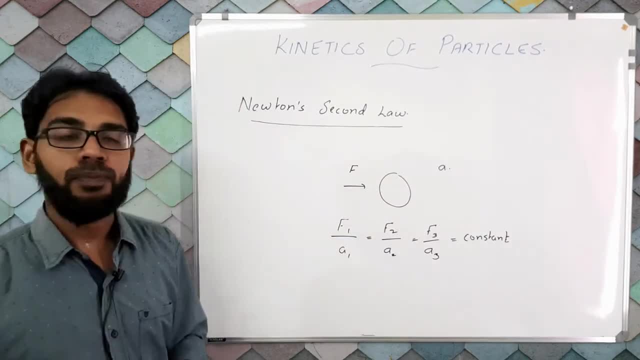 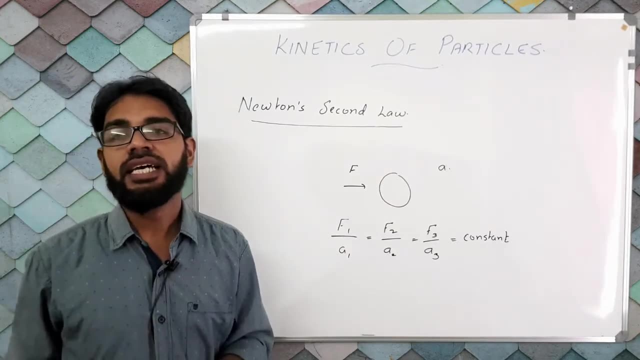 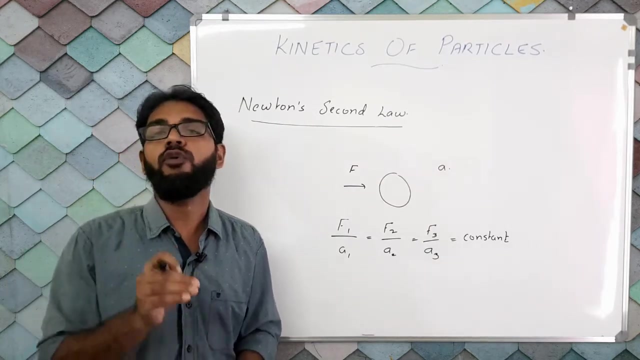 It has a constant value. Now this constant refers to the inertia of the particles. The Newton's first law indicates that the body continues in a state of rest or in a state of constant velocity if no external force acts on it. Therefore, inertia can be seen as the 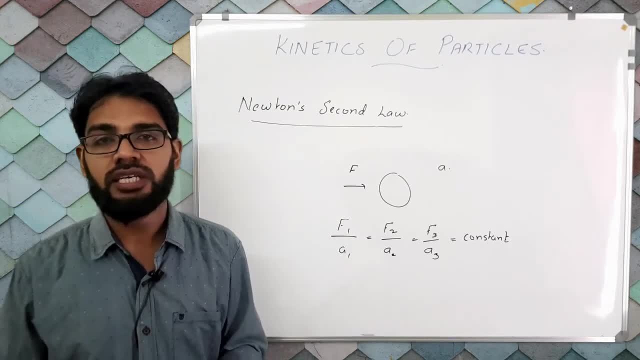 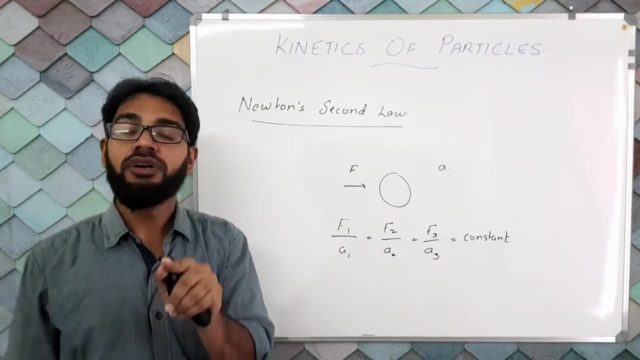 resistance to the rate of change of velocity. The resistance to the rate of change of velocity. The resistance to the rate of change of velocity: 1.1 income minus one unit mass times root 2 minus constant into solar which generations of velocity? Now, since mass is a quantitative measure of inertia, we can write this corresponding: 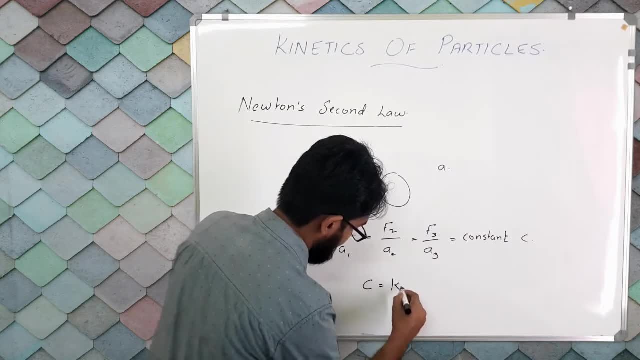 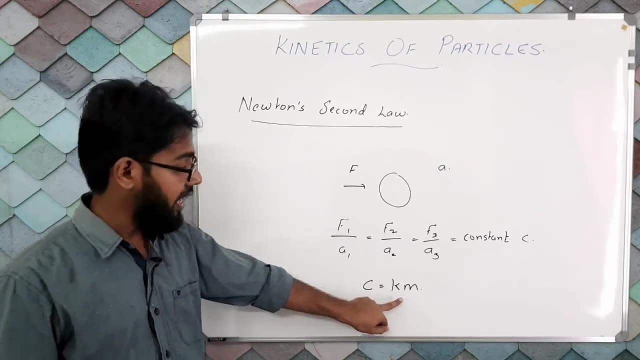 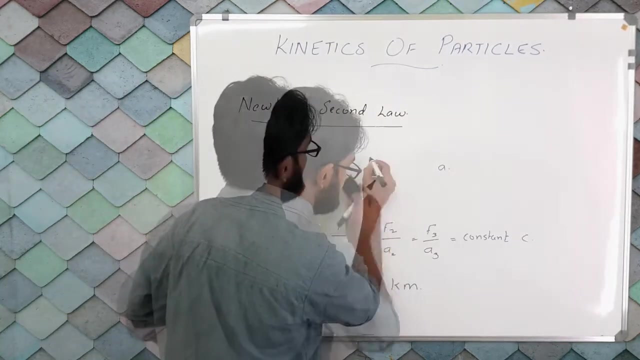 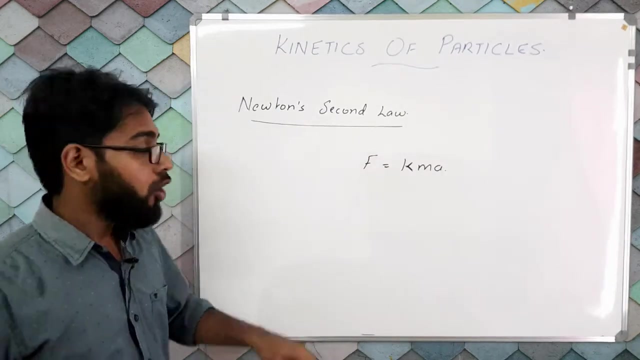 constant C as Km, where m is the corresponding mass of the body or the mass of the particle and K is the corresponding constant. Now from this we can get that F equals KmA. Now on observation you can see that the acceleration is always in the direction of. 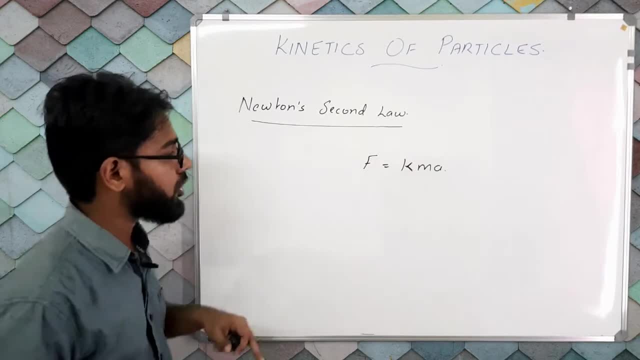 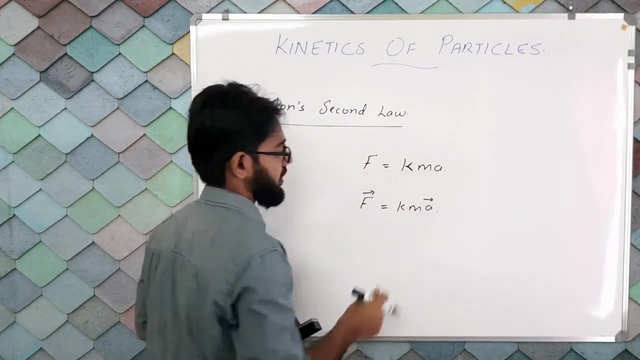 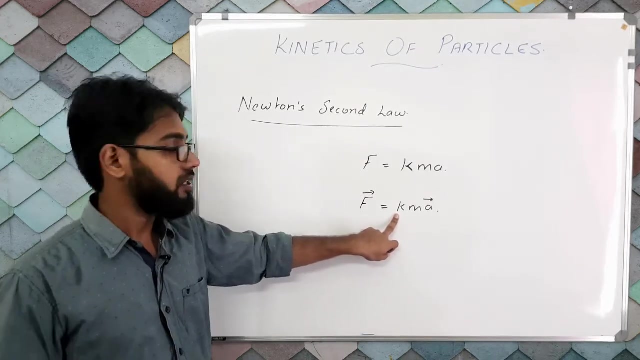 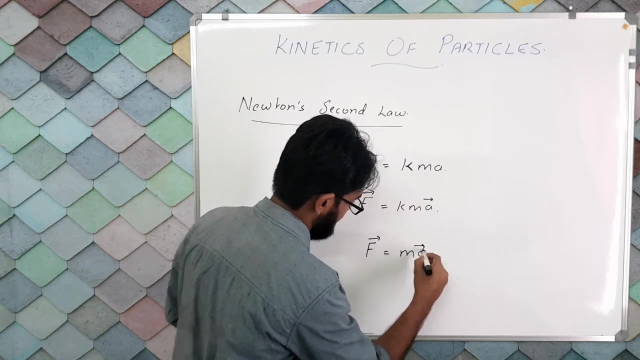 force. Hence a vector relation of the above equation can be written as: F vector equals KmA. Now the value of K can be taken as unity when it comes to SI units. So this equation gets reduced to F vector equals m into A vector. This is the corresponding equation you must have studied in. 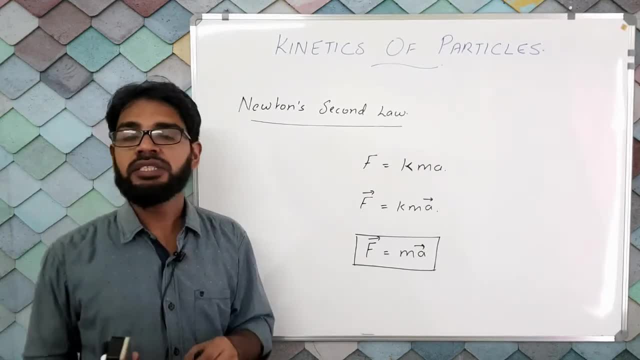 your higher secondary classes. Now, if a particle is subjected to several forces, then the Newton's law takes the force. So if a particle is subjected to several forces, then the Newton's law takes the force. So if a particle is subjected to several forces, then the Newton's 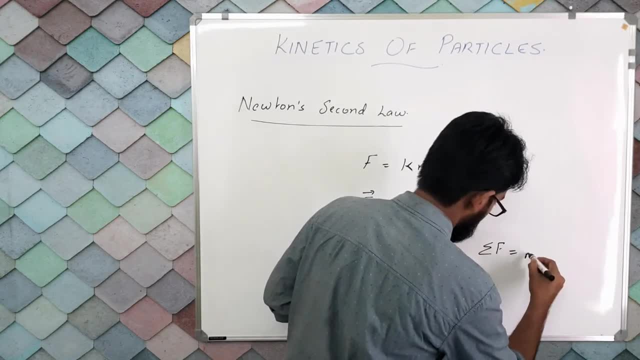 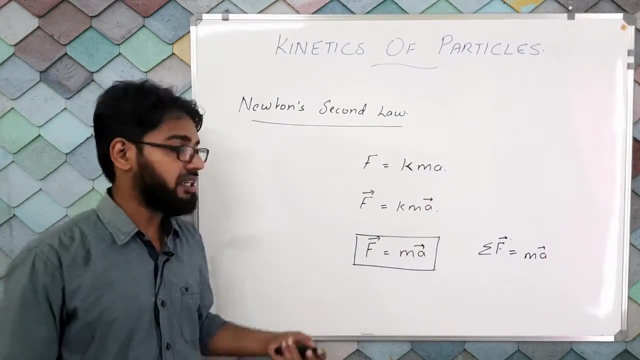 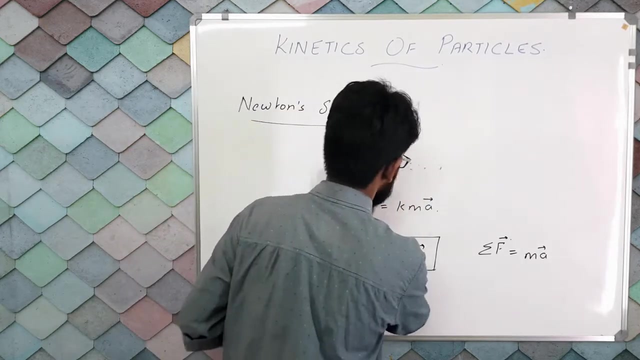 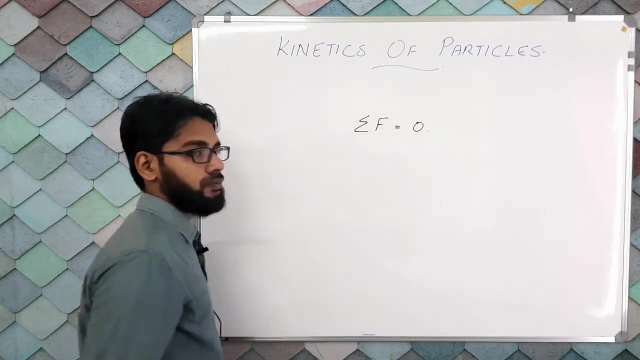 law takes the force. So if a particle is subjected to several forces, then the Newton's resultant, or the sum of all the forces acting on the particle. Now moving on, in statics you had used the equation sigma F equals 0. However, in dynamics, the Newton laws gives: 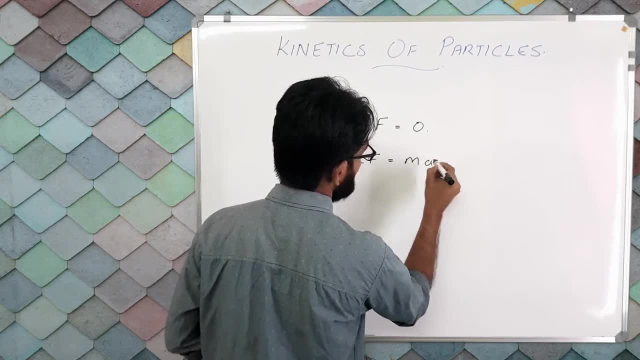 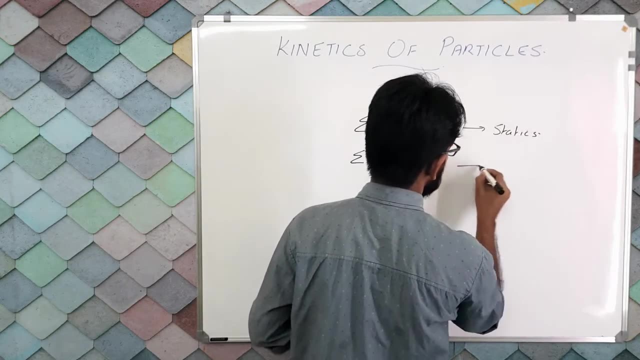 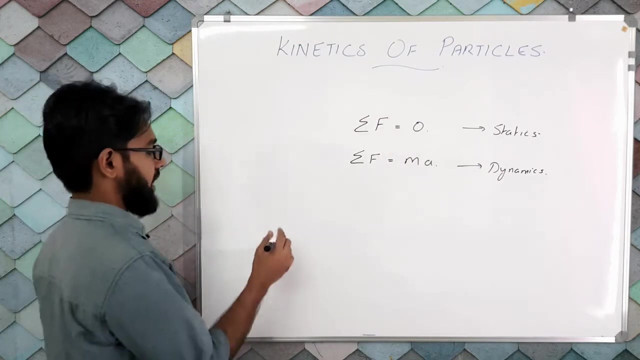 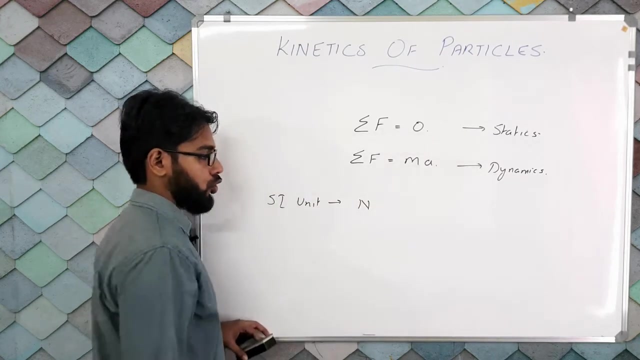 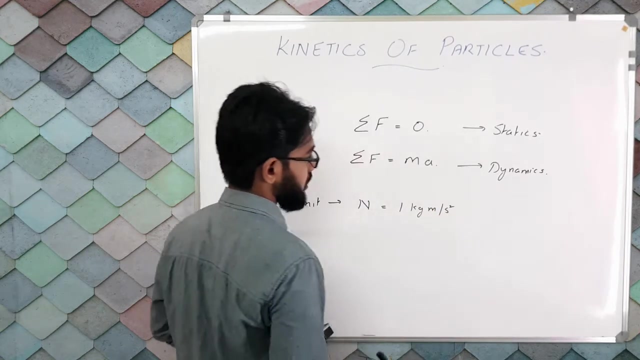 us sigma F equals m into k. So this is in statics, this is in dynamics. Now the SI unit of force is Newton. So 1 Newton is 1 kilogram meter per second. So this is the second square. So mass as a unit of 1 kilogram and acceleration 1 meter per second square. 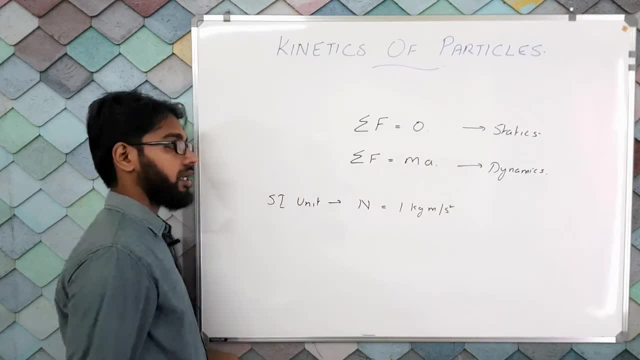 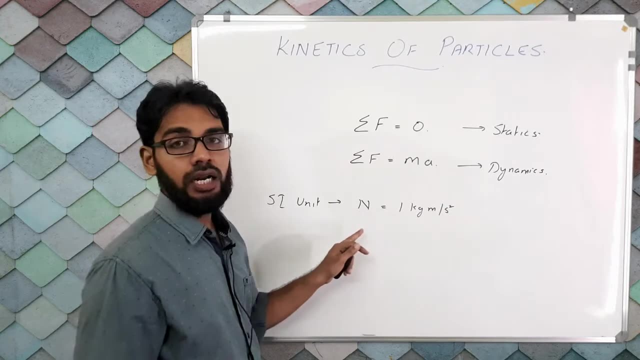 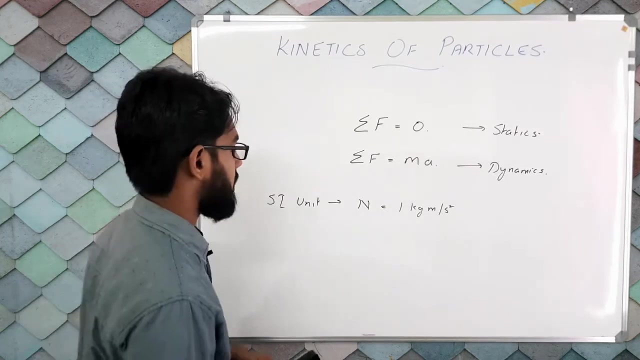 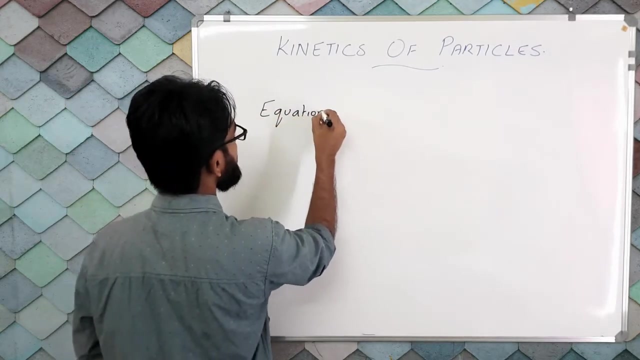 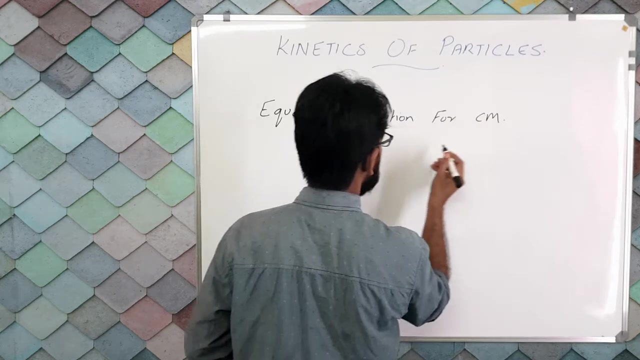 So 1 kilogram meter per second square is 1 Newton. So whenever you solve problems you should ensure that the corresponding units are properly converted so that you do not get mistakes. Now we go to the topic: Equation of motion for center of mass, for CM, center of mass. Now in my first lecture, 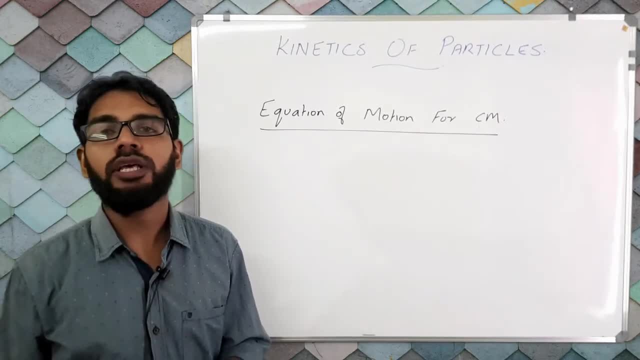 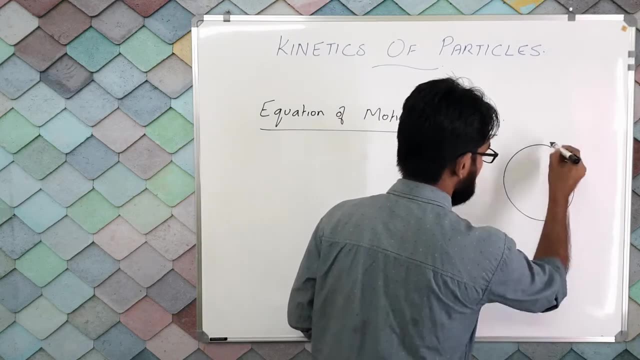 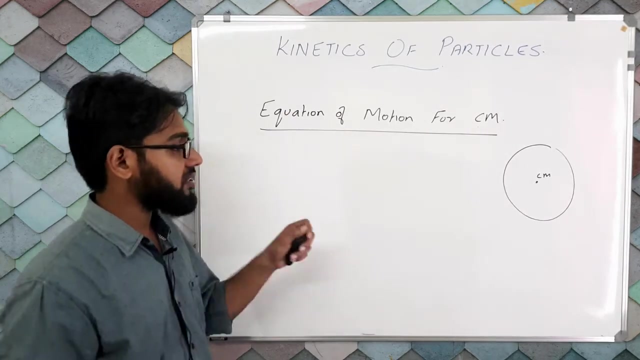 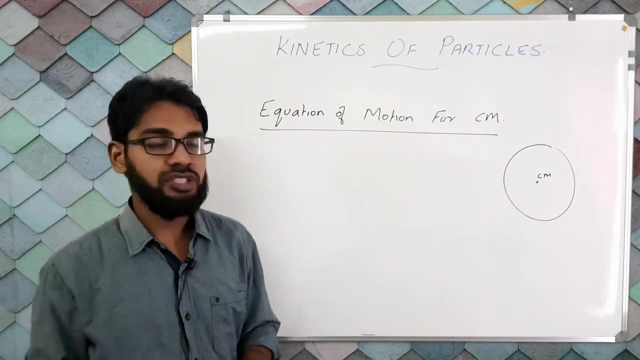 I had said that when we idealize a body of significant size to a particle, we consider the motion of the center of mass For describing the motion of the body. Now this idealization works because all the particles within the corresponding body has the same motion parameters as the center of mass. Now 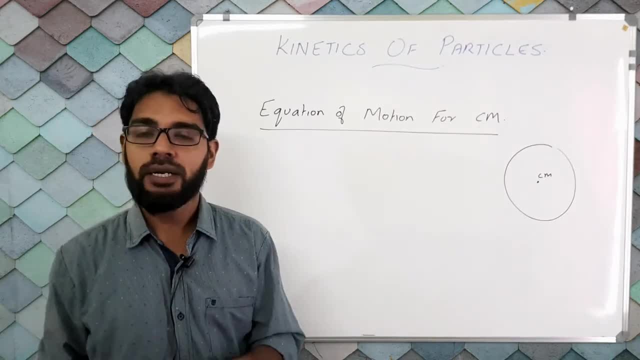 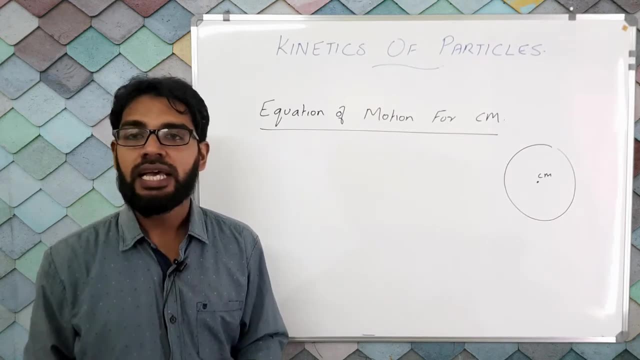 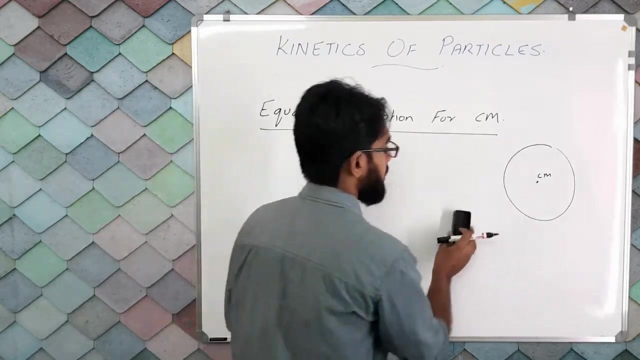 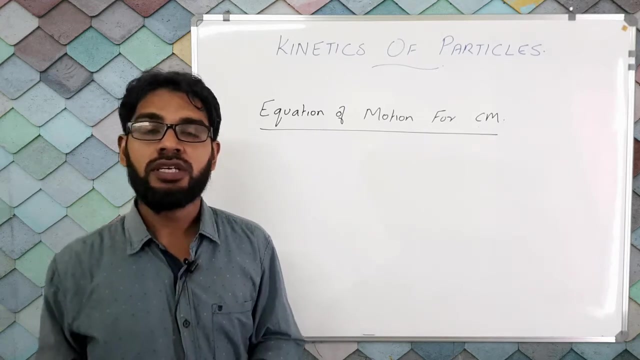 the Newton's second law was actually postulated for a particle. In this corresponding topic we shall see that if a Newton's law for a system of particles can be described by considering only the mass center, Now in case of a system of particles within a body, there are two types of forces: that 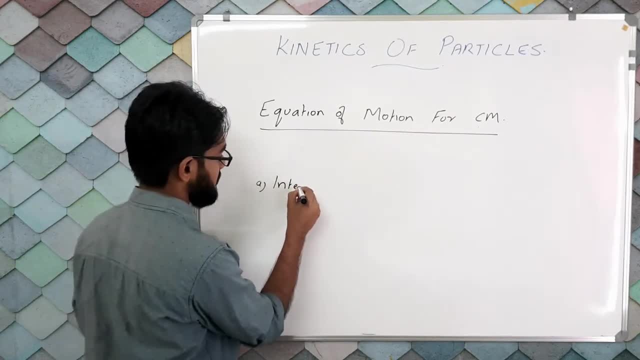 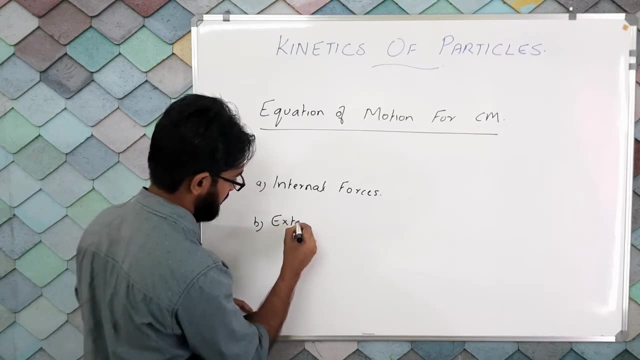 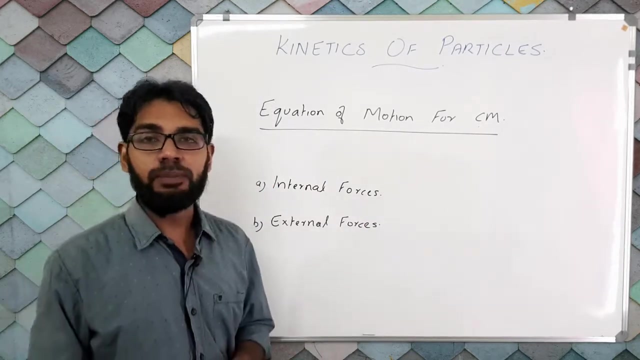 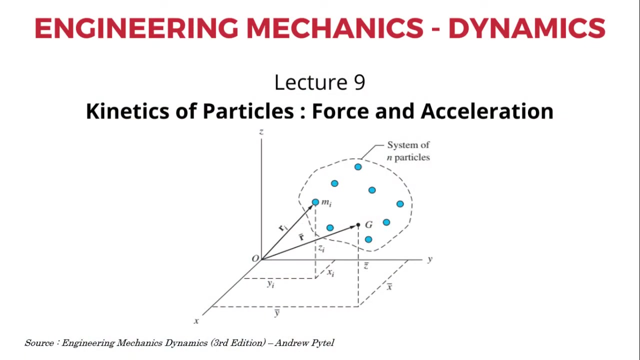 come into picture A- internal forces and B- external forces. Now consider: I have an arbitrary system of particles as shown in this figure. Assume that no mass enters or leaves the system, Let Mi be the mass of the ith particle and Ri be its position vector, So the total mass. 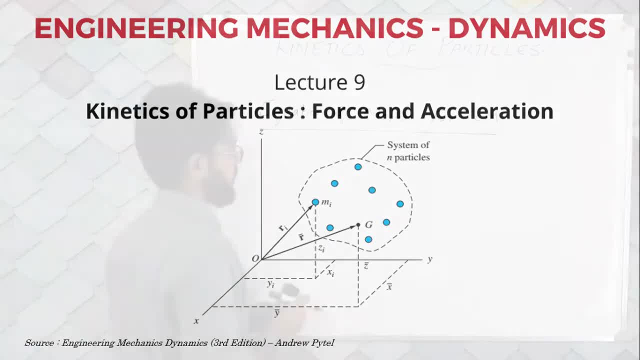 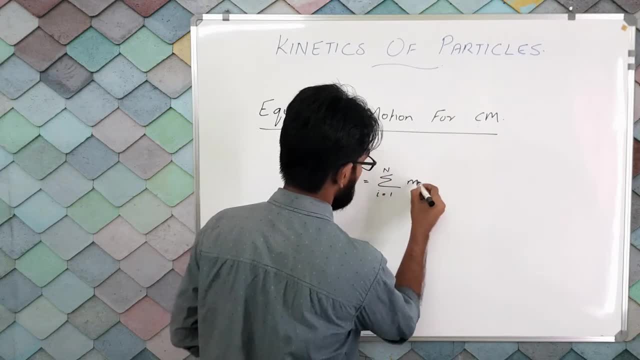 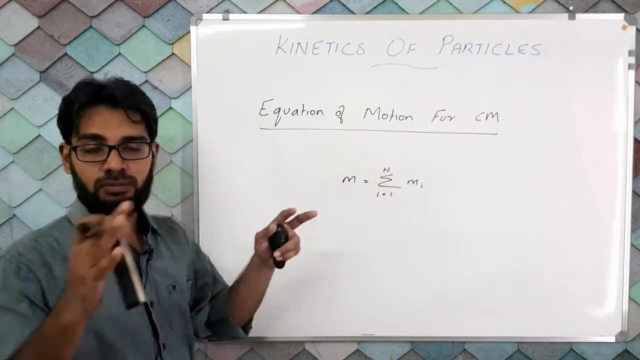 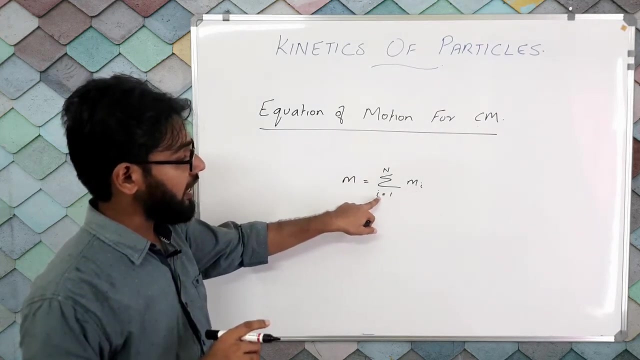 of the particle can be given as: M equals sigma i from 1 to n Mi, where m is the corresponding mass of the entire system of particles put together. mi is the mass of the ith particle. So if you sum it from corresponding i equals 1 to capital N. 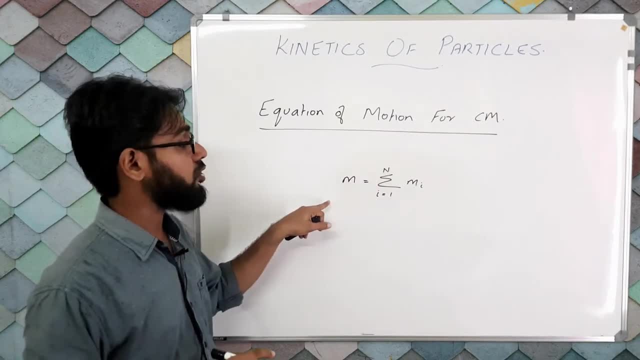 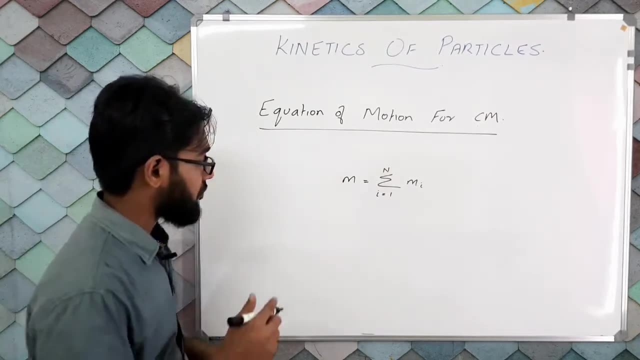 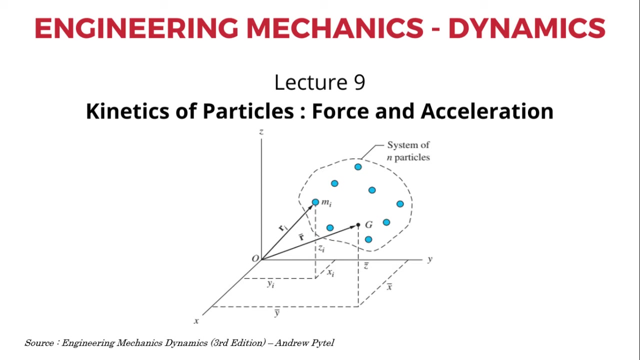 where capital N is the total number of particles. So this will give you the mass of the entire system of particles. Now suppose the position vector of the center of mass. If you see the figure, you can see that the center of mass is represented by the capital G. 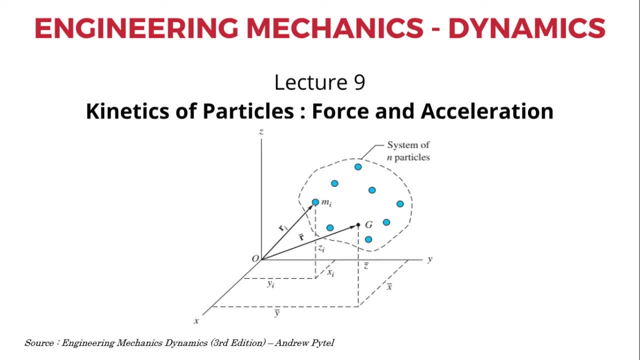 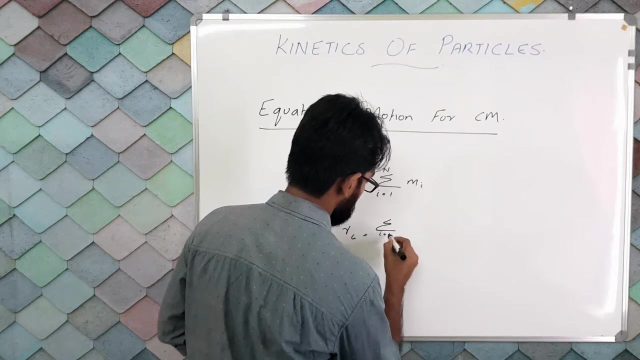 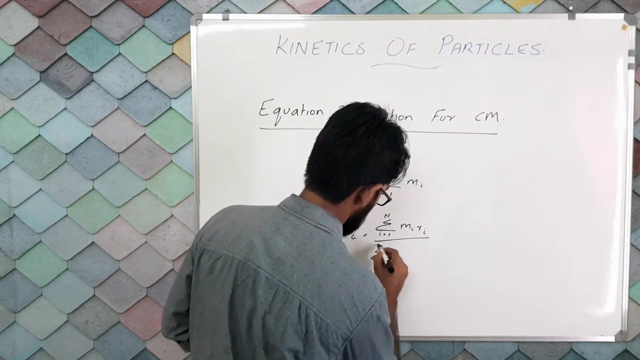 Now, if the position vector of RG, whose coordinates are given in terms of x dash, y dash and z dash in the Cartesian coordinates, The position vector RG of the center of mass of the system of particles can be given as: RG equals sigma i equals 1 to N mi. ri, divided by sigma i, equals 1 to N mi. 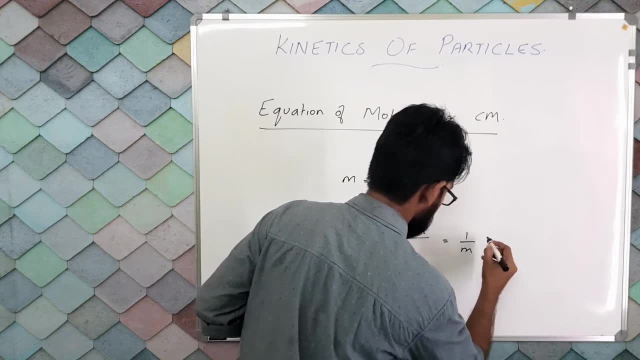 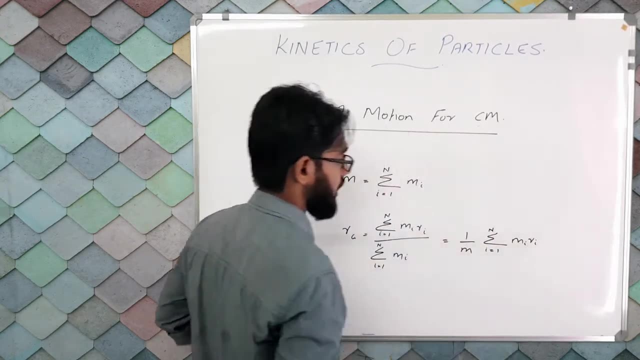 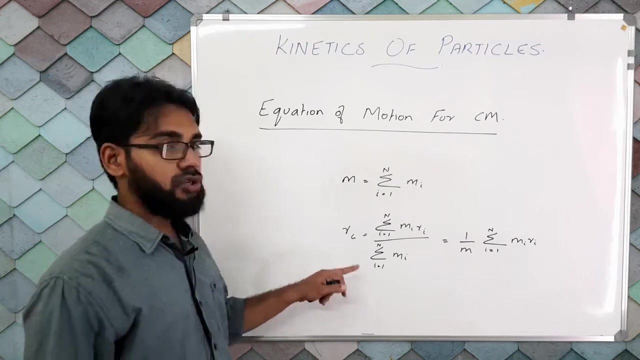 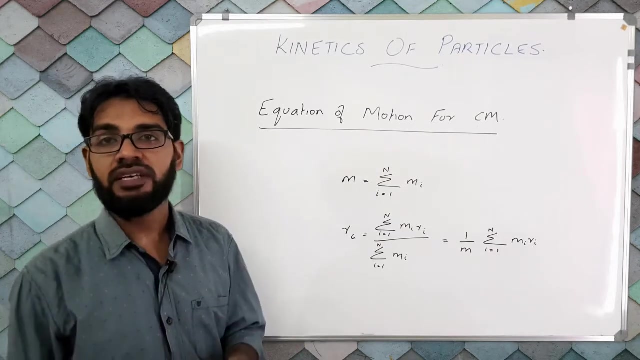 which I can give it as 1 by M sigma i equals 1 to N mi ri, where ri is the position vector of the ith particle. Now engineers usually use the center of gravity and center of mass interchangeably, since these two points coincide in most of the applications. 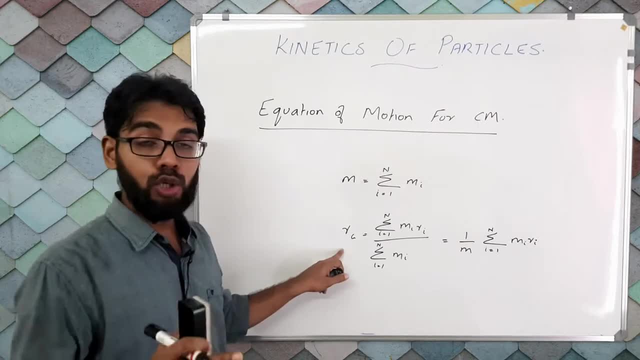 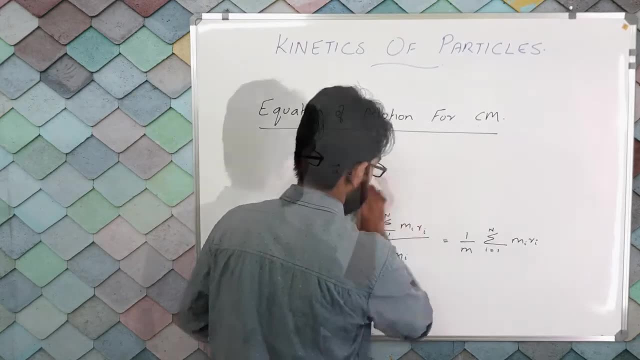 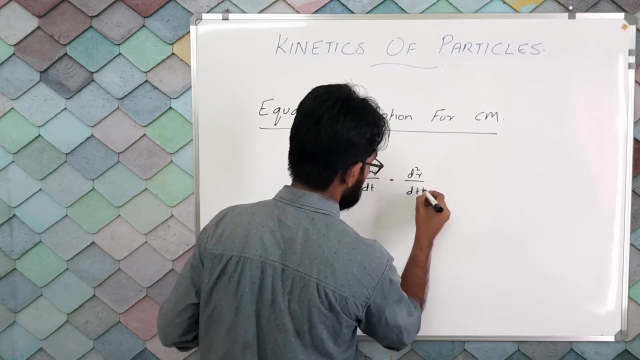 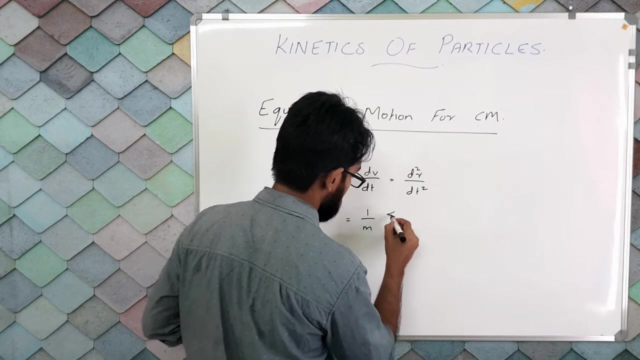 Now if I differentiate this corresponding equation twice to get the corresponding value of acceleration of center of mass, I would get a equals dv by dt is equal to d square, R by dt square, Which would be equal to 1 by M sigma i equals 1 to N mi ai. 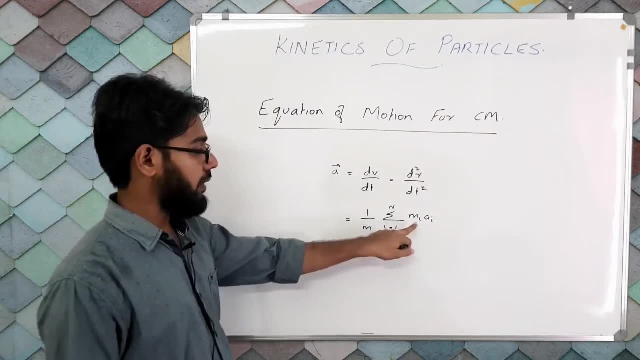 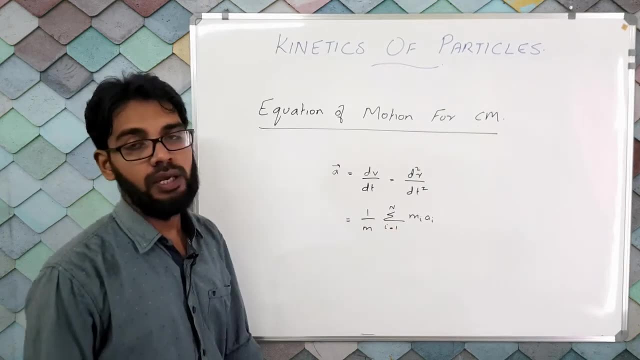 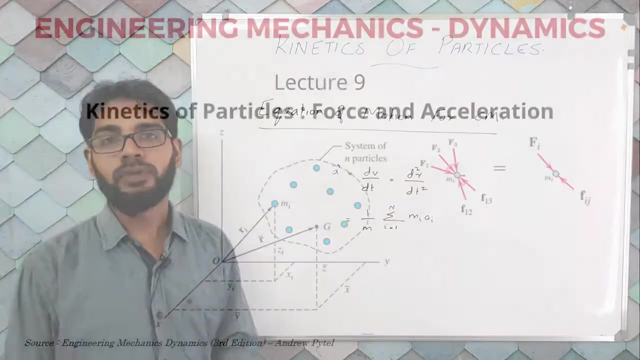 Now this will remain. 1 by M will remain a constant, mi will remain a constant. So when I differentiate Ri, it will get converted into ay. Now this corresponding ai indicates the acceleration of the ith particle. Now let us come to forces. 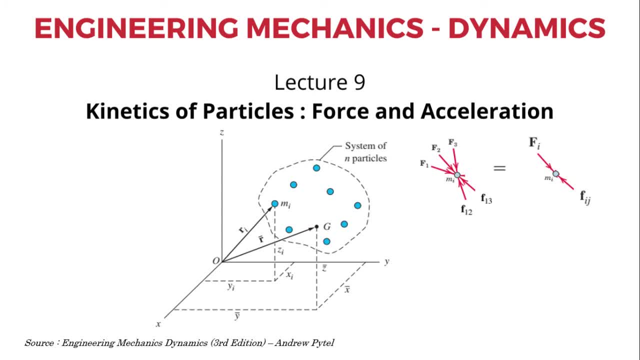 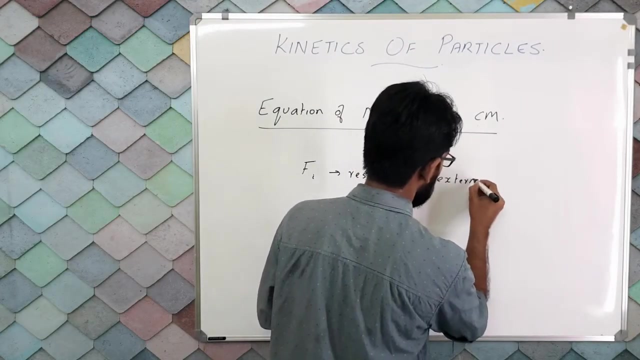 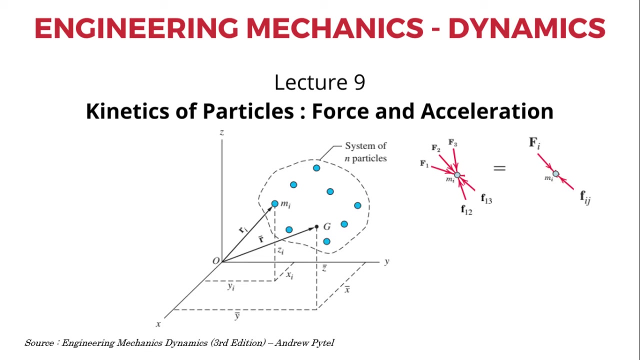 Let each particle i be exerted upon by several external forces, as shown in this figure, The resultant of all the external forces can be given as Fi, which may include its weight, its interactions with other particles that are not included within the system. In addition to the external forces, the particles of the system may also be subjected to forces. 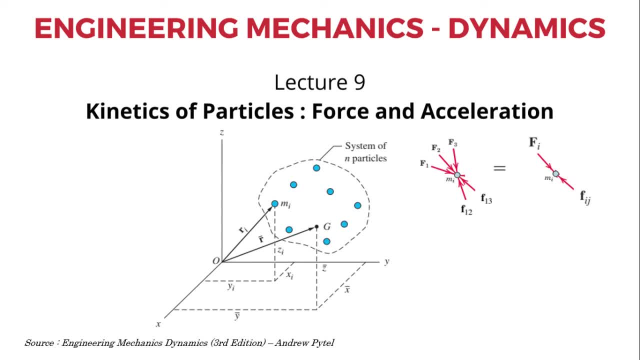 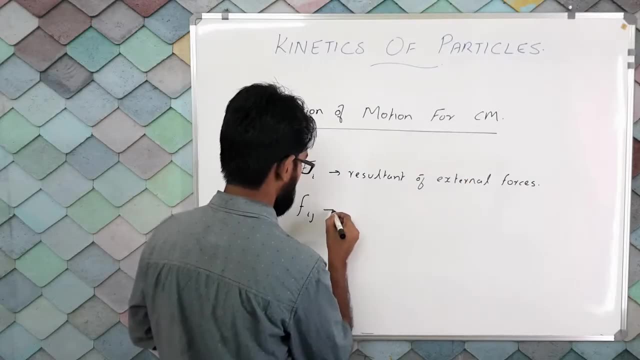 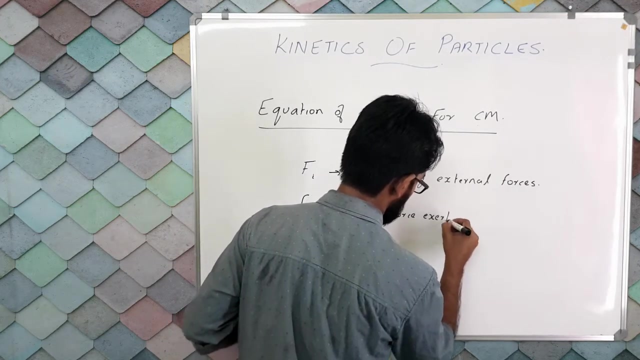 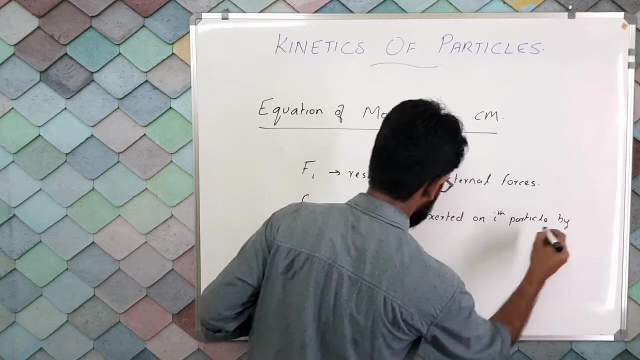 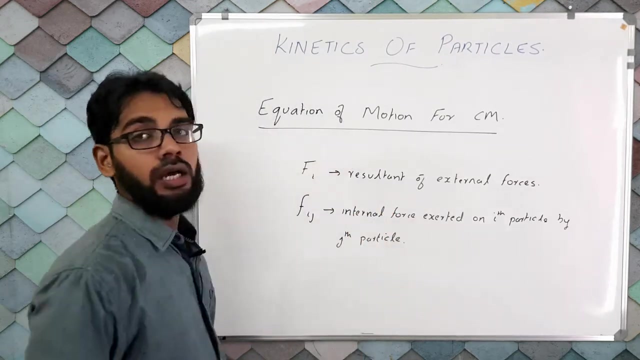 that are internal to the system. Internal forces are caused due to interactions of particles within the system. Let the internal forces be represented by Fij. Fij indicates the internal force exerted on i-th particle by j-th particle. Now each particle can have an interaction with each other particle in the system. 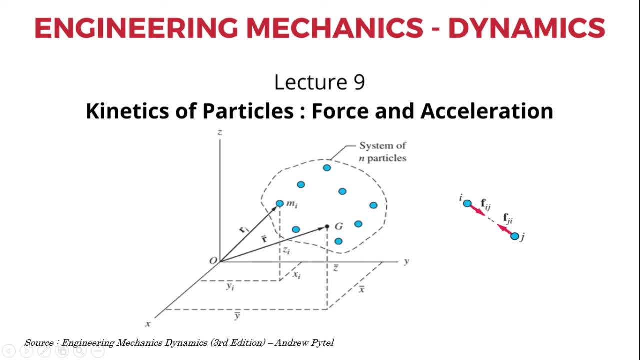 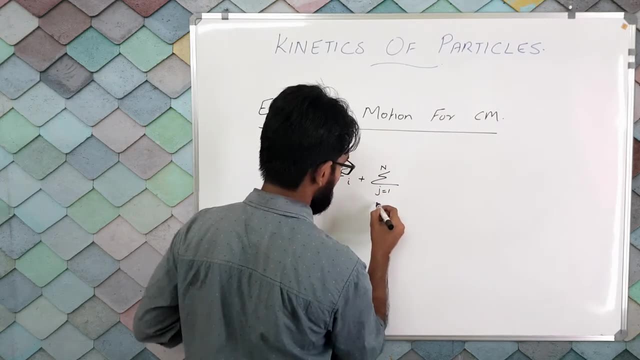 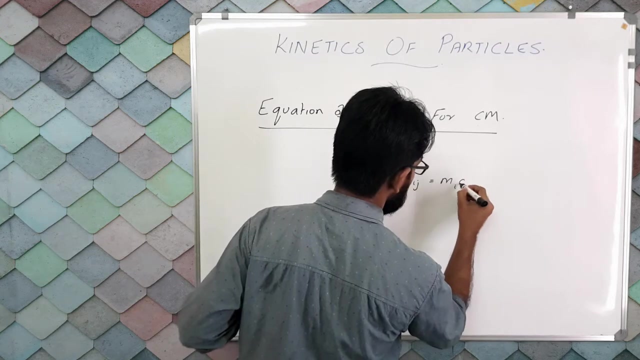 But only one such interaction is shown in this corresponding figure. Now let us apply the Newton's second law on i-th particle. So we have Fi plus sigma j equals 1 to n over j, not equal to i. Fij is equal to mi a-th. 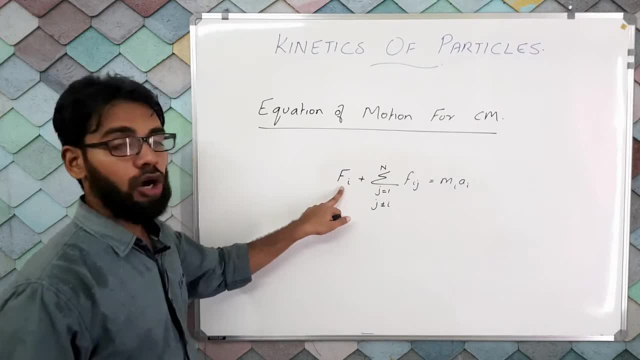 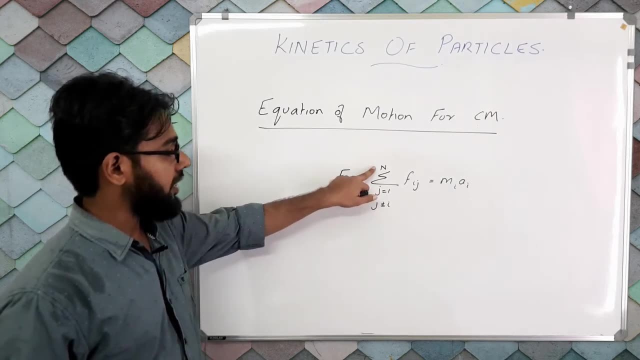 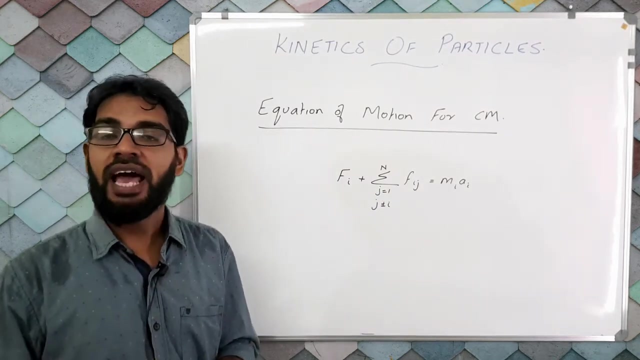 Here: Fi indicates the resultant of all the external forces acting on the i-th particle. Sigma j equals 1 to n. j not equal to i. Fij indicates the summation of all the internal forces acting on the i-th particle by all the other corresponding particles in the system. 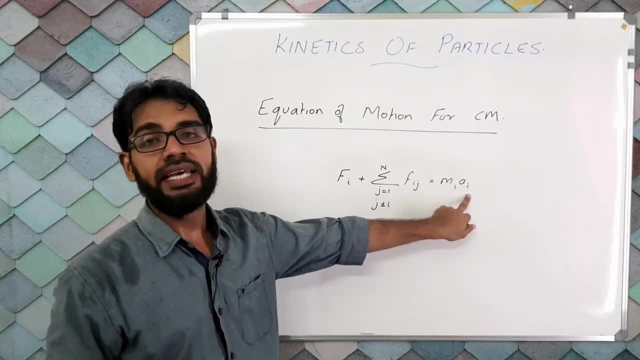 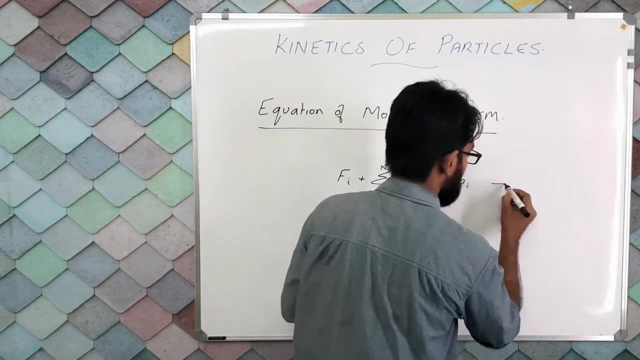 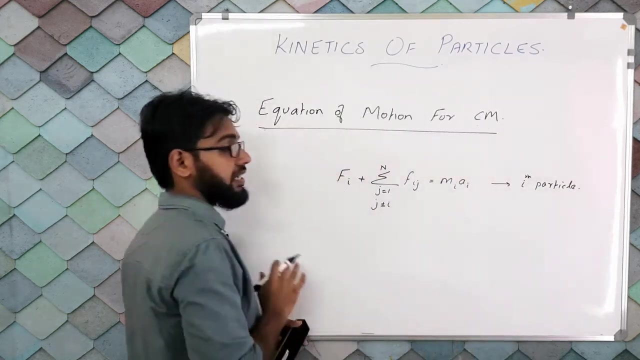 mi is the corresponding mass of the i-th particle and ai is the corresponding acceleration of the i-th particle. Now, this is for a single particle. Now this is for a single particle. If I submit all the corresponding equations of all the particles, I would get. 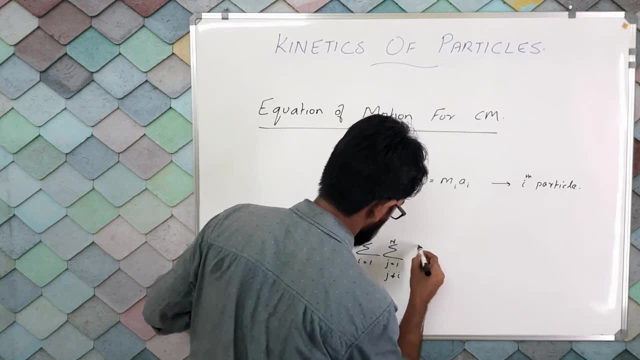 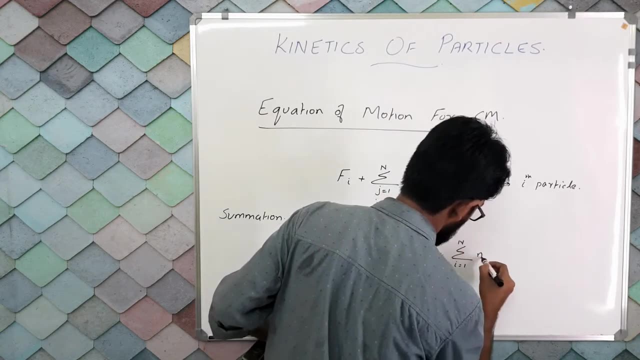 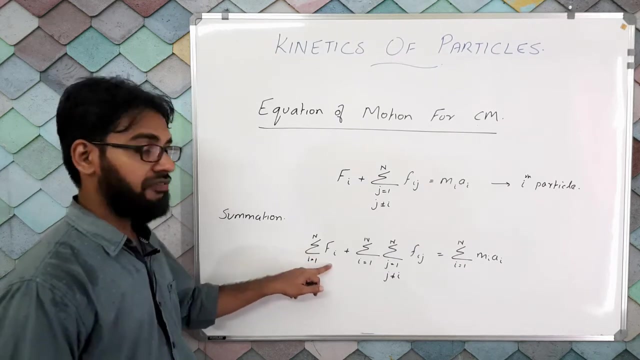 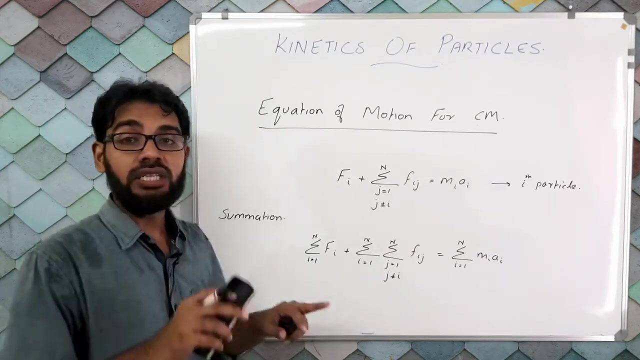 This corresponding equation, Where sigma i equals 1 to n, Fi indicates the corresponding forces, all the external forces that are acting on the system of particles. Sigma i equals 1 to n. Sigma j equals 1 to n. Sigma j equals 1 to n. 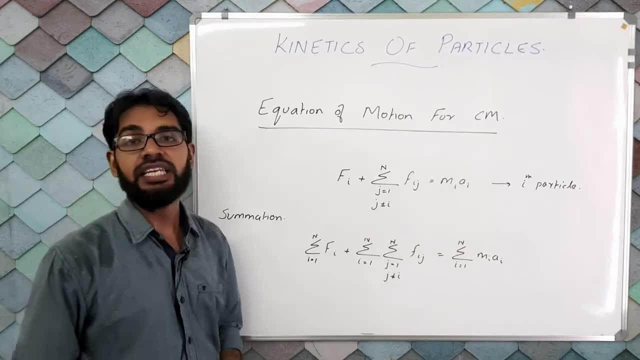 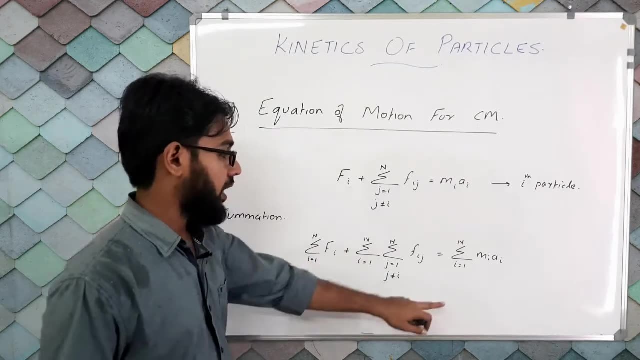 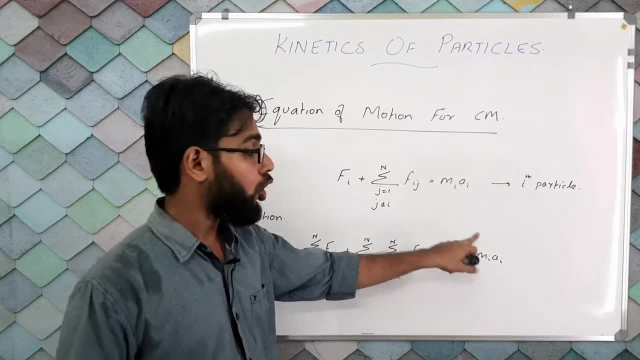 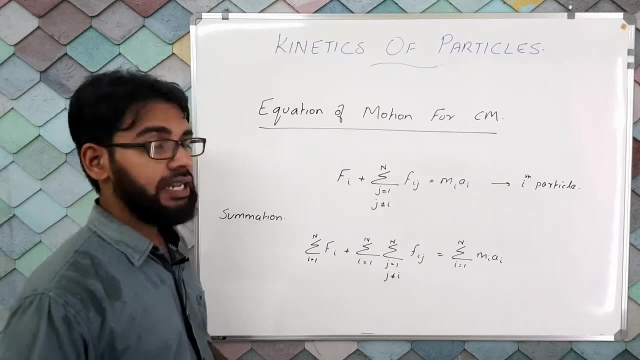 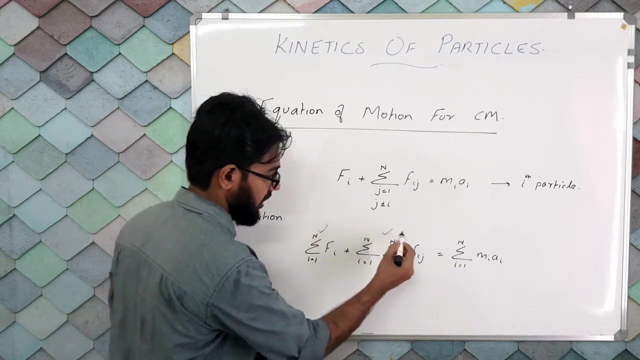 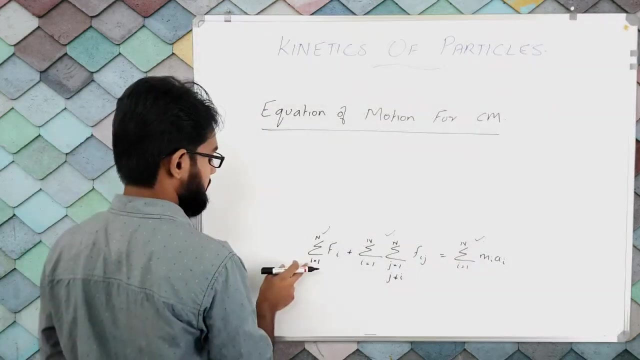 summation of m a for all the particles within the system. Now, if you look at this corresponding equation closely, we can make three different simplifications: First for this, the second for this and third for this. Let us come to each of these separately. I can simplify this equation. 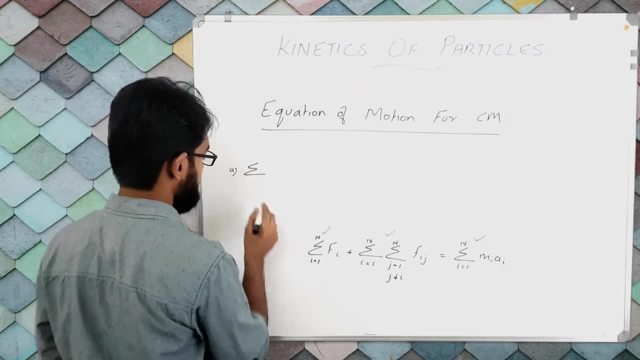 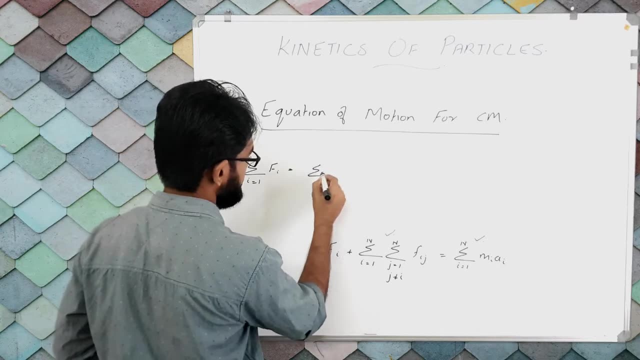 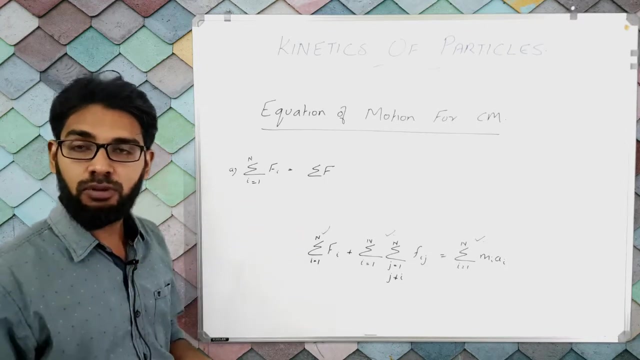 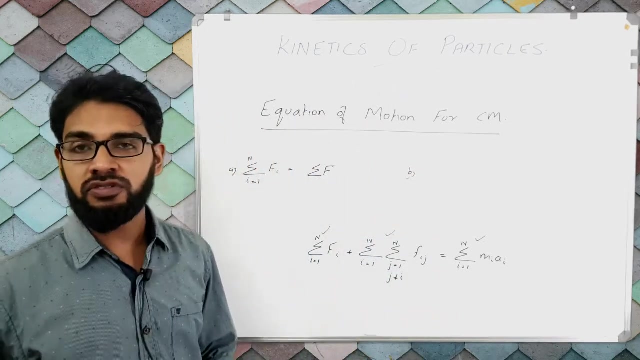 in three aspects. First one: sigma i equals 1 to n f. i is equal to sigma f. Now sigma f represents the sum of all the external forces acting on the system of particles together. now the second aspect. you know that the internal forces occurs in pairs that are equal in magnitude. 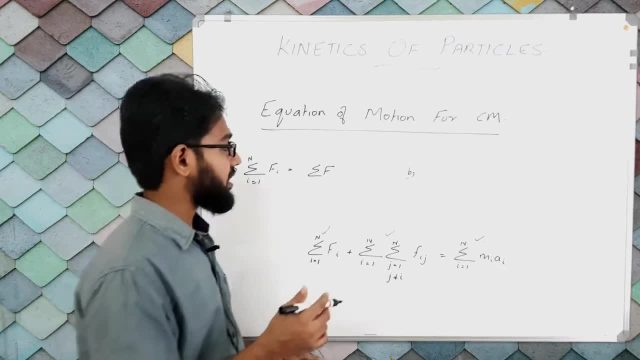 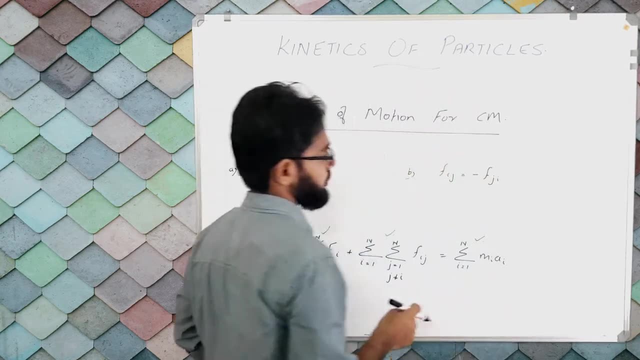 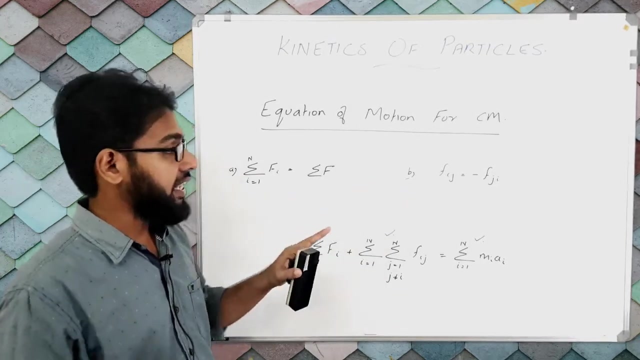 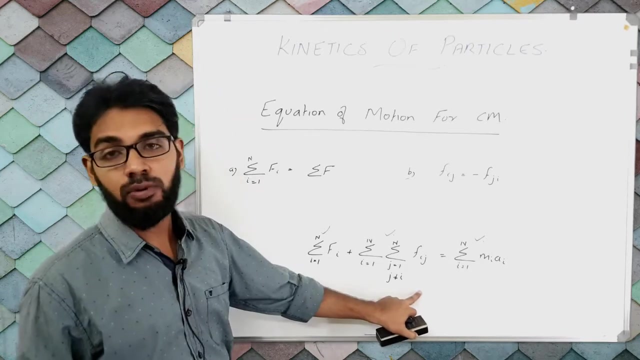 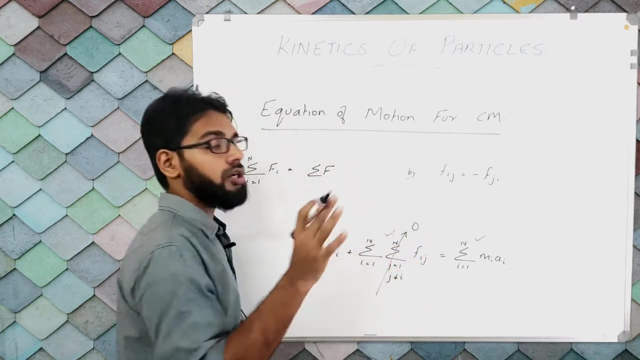 opposite in direction and are collinear. so i can write: f i j is equal to minus f j i. okay, as per now, as per the newton's third law. now, if i take the sum of all the internal forces acting on the system means this corresponding part, you will find that this will turn out to be zero. since all these 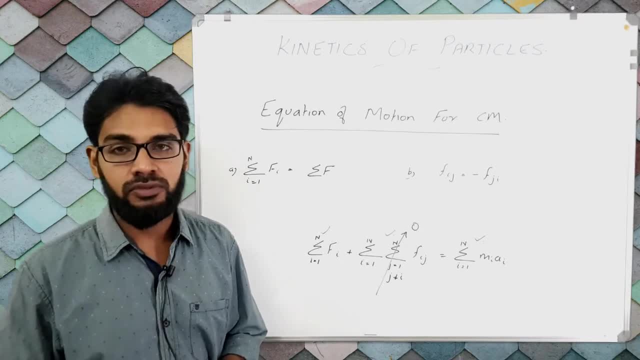 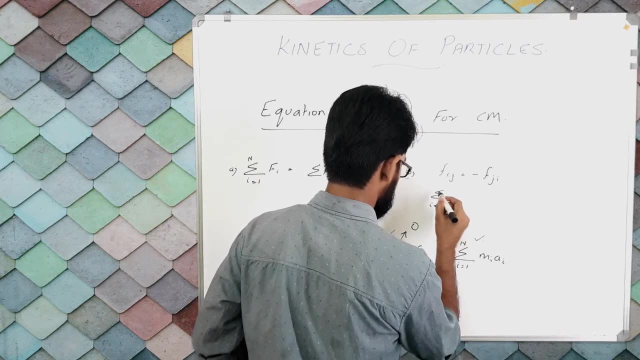 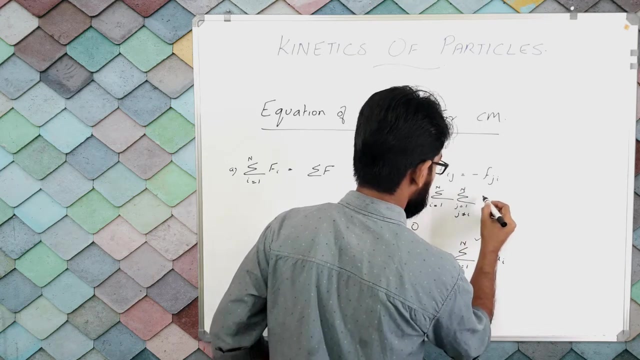 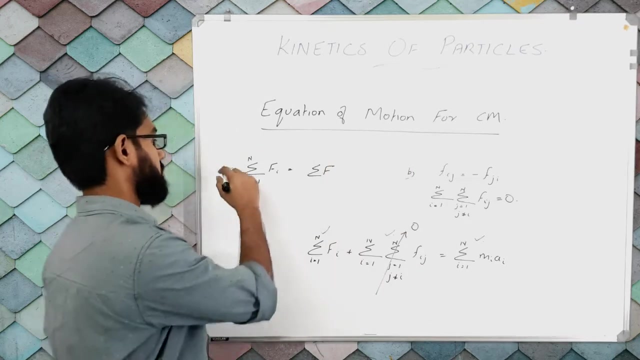 corresponding forces will cancel out each other. so this is the second aspect. sigma i equals 1 to n, sigma j equals 1 to n, j not equal to i. f, i, j is equal to 0. so the first, the second, now the third aspect, c is sigma. 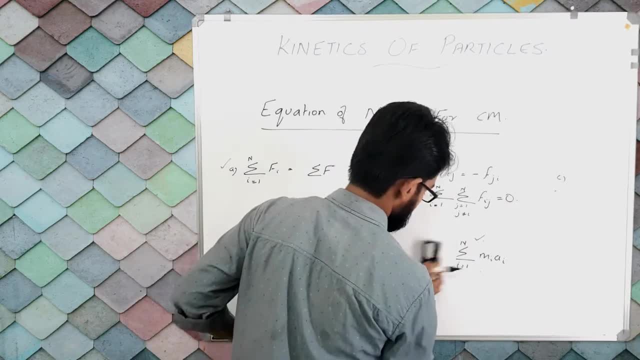 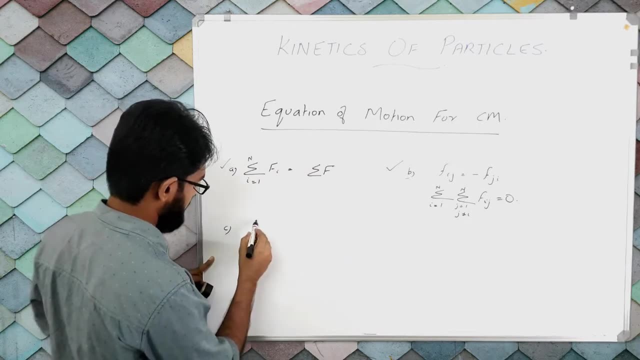 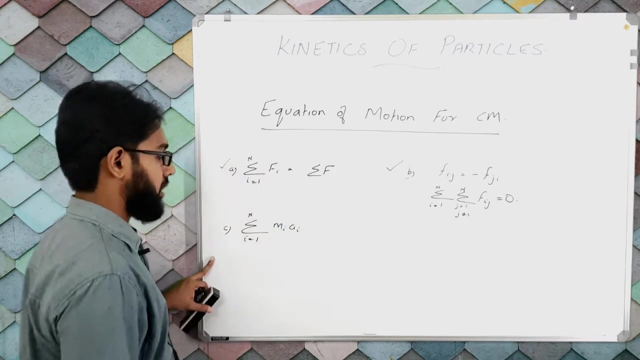 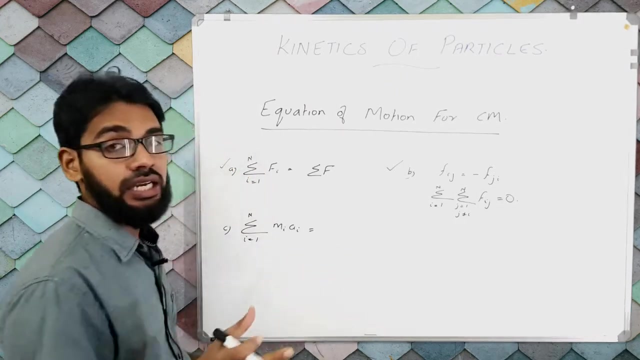 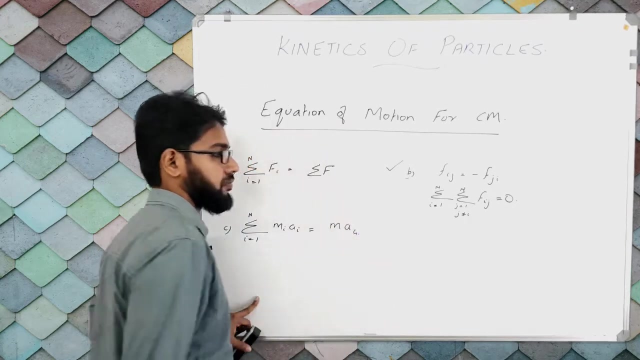 i shall rub it out here: sigma i equals 1 to n, m, i, a, i. now we have already studied earlier that this corresponding thing can be expressed in terms of the mass sender as m into h, m into 80.. now, applying all these three things, 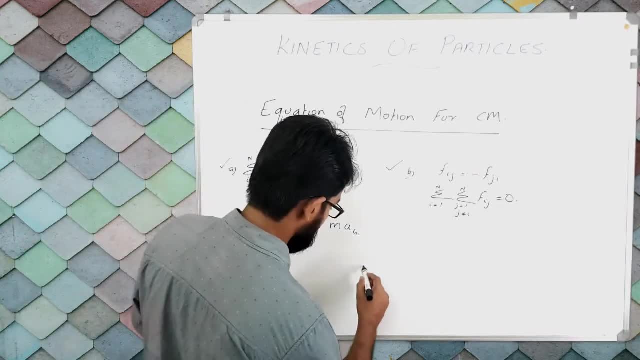 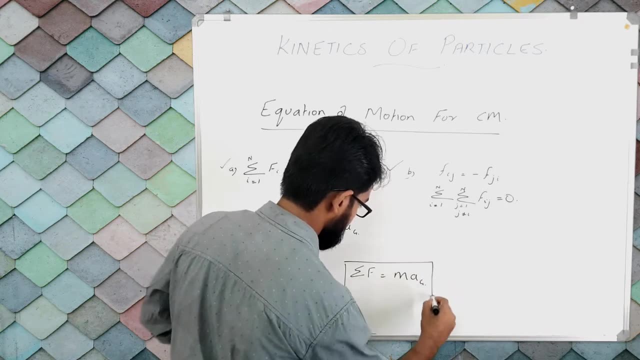 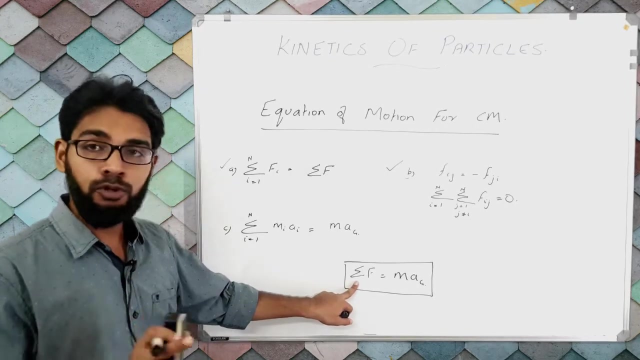 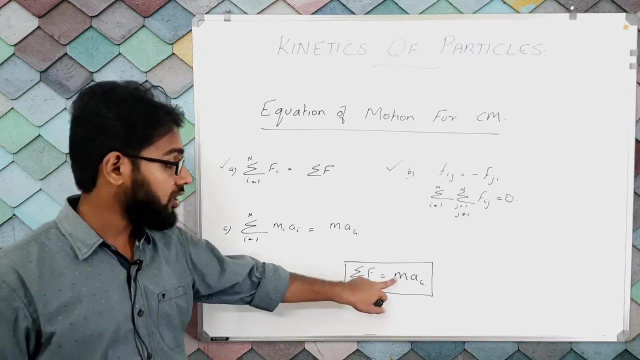 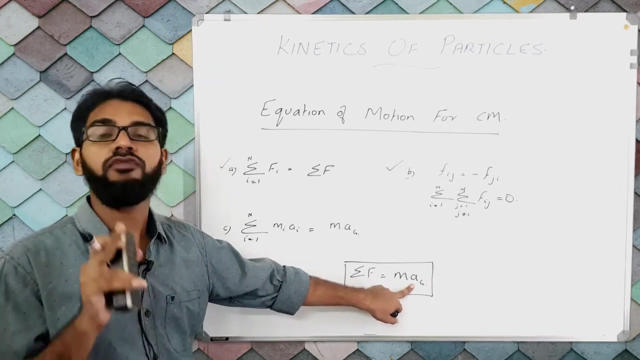 in the corresponding equation we would get that sigma f is equal to m a, g. This indicates that the sum of all the external forces acting on the system of particles is equal to the corresponding total mass of the system of particles, multiplied by the acceleration of the center of mass. 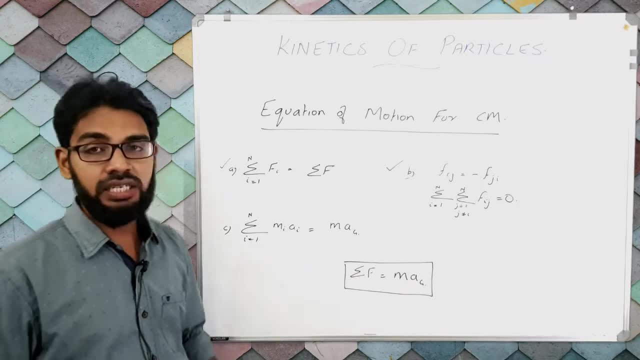 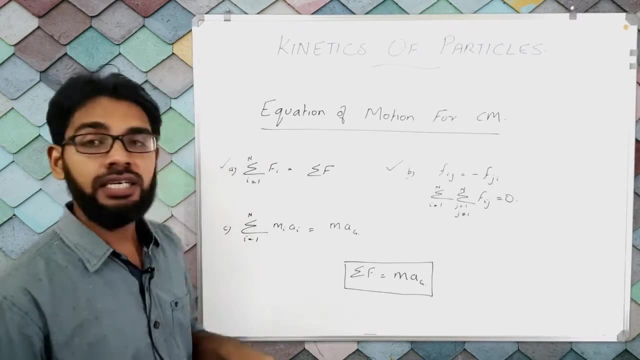 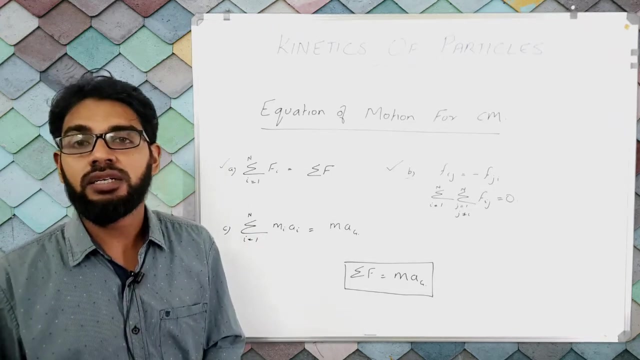 Now, if you look this closely, it is similar to the corresponding Newton's law for a single particle, except that here sigma f represents the corresponding force acting on the entire system of particles together, and a g represents the acceleration due to gravity of the center. 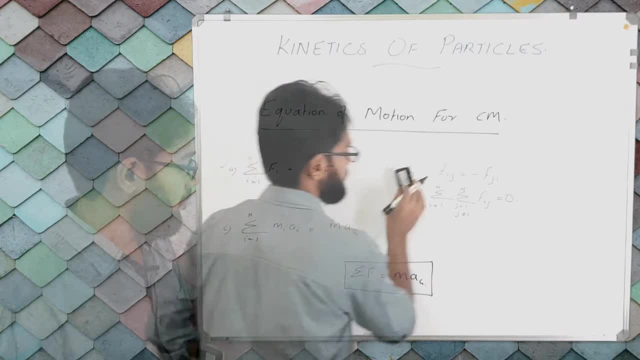 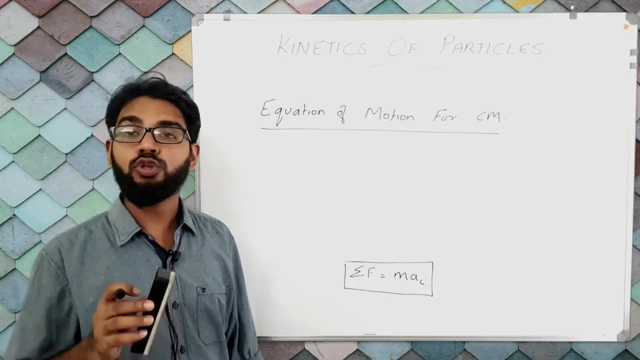 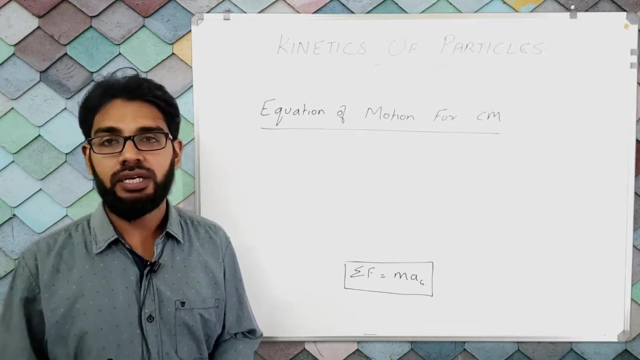 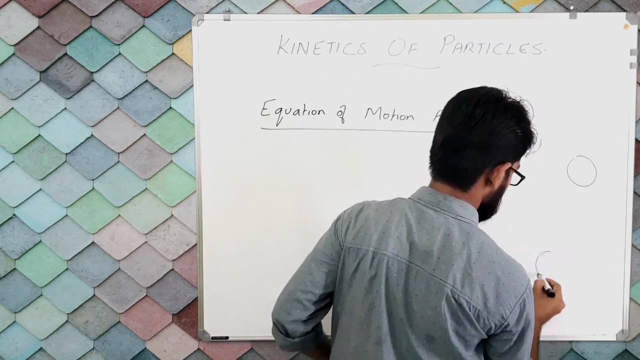 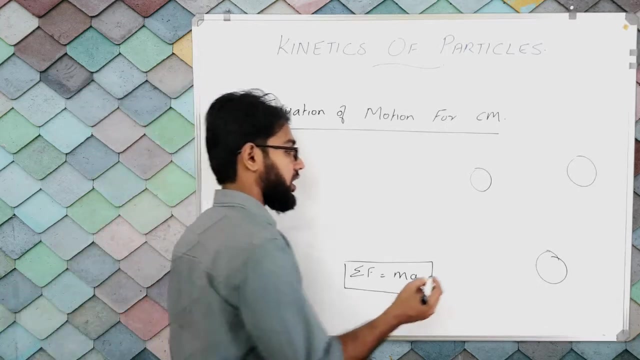 of mass. Thank you. Now. this corresponding equation, sigma f equals m into a g, is also valid for a system of bodies where each body can be idealized to a particle. So if you have a system of bodies that is acted upon by some external forces, if we 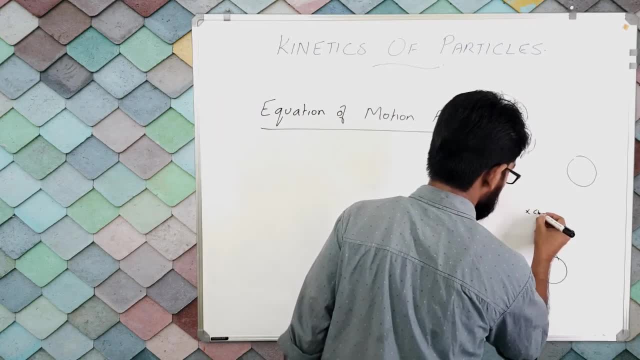 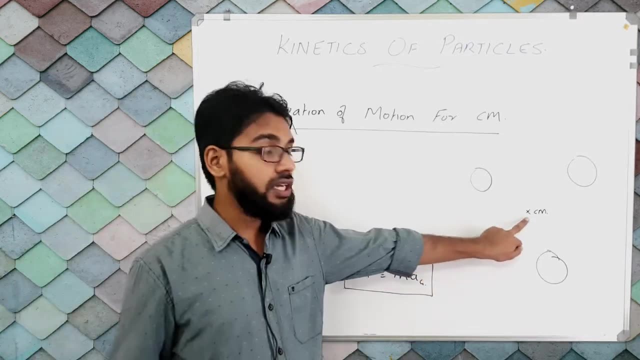 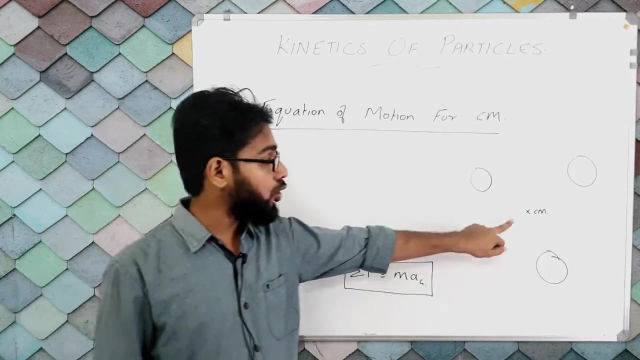 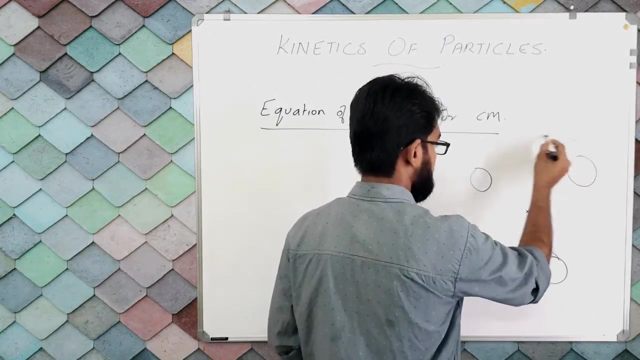 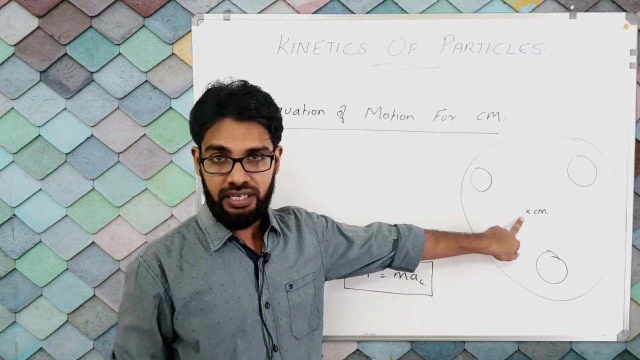 are able to find the corresponding Center of mass of this system of particles, then the acceleration of the mass center and the corresponding external forces acting on the mass center is sufficient in describing the motion of the system of particles as a whole. I repeat: the corresponding acceleration of the mass center and the external forces acting. 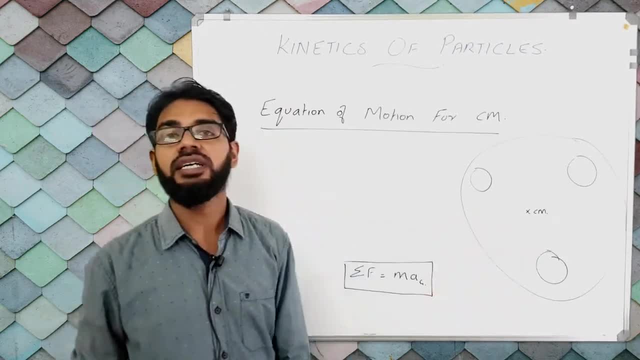 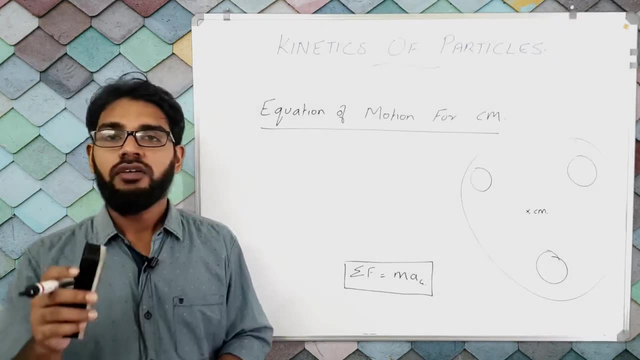 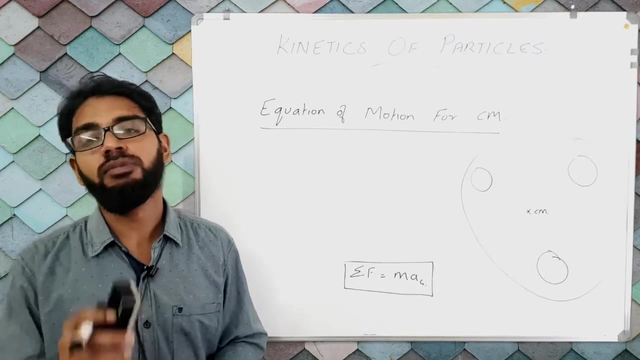 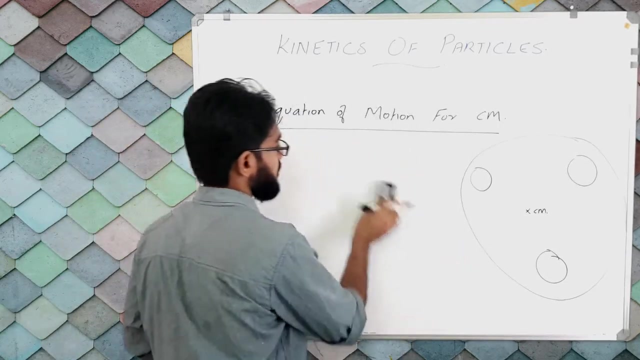 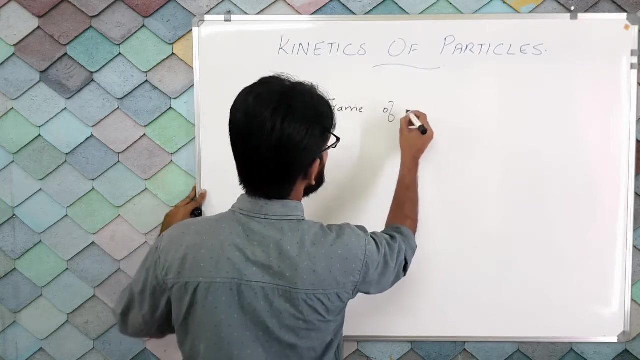 on the mass center, forces acting on the mass center- is sufficient in describing the motion of the system of bodies as a whole. We shall discuss the problem related to the motion of mass center when we deal with the kinetics of system of particles later Now. the next topic which we shall discuss today: inertial frame of reference. 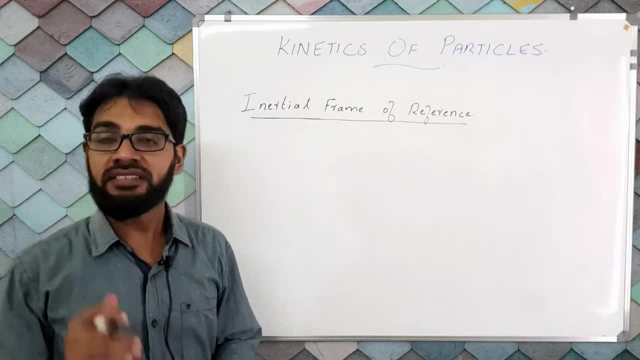 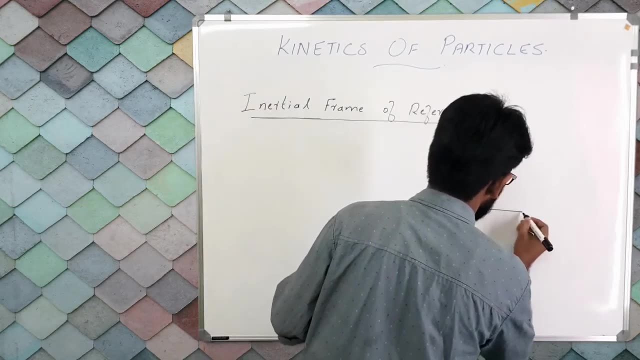 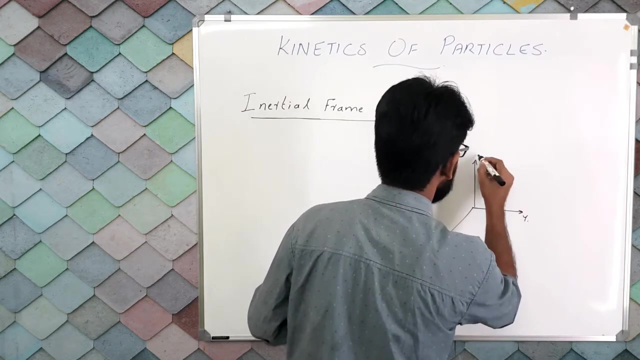 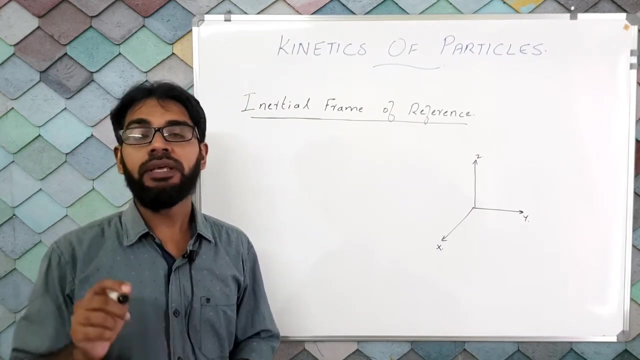 In kinematics of particles we had discussed that the position, velocity and the force of the motion of the system of particles are different. The position, velocity and acceleration were specified on the basis of a reference frame. Now Newton, however, stated that the second law can be expressed only in a frame of reference. 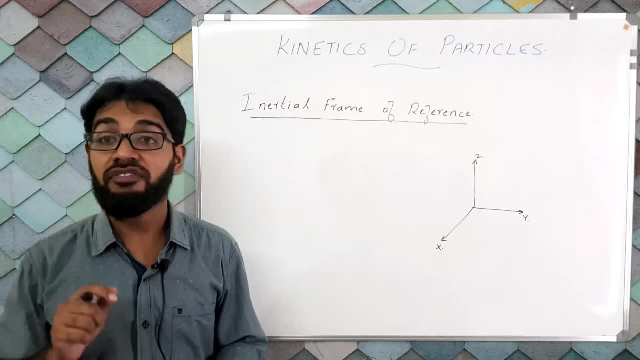 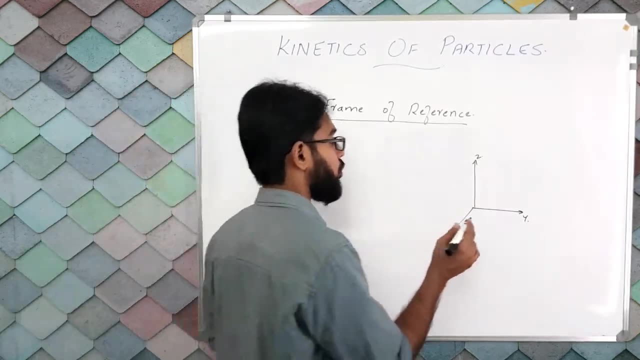 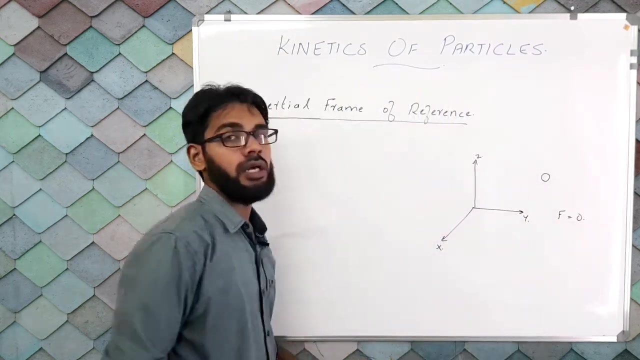 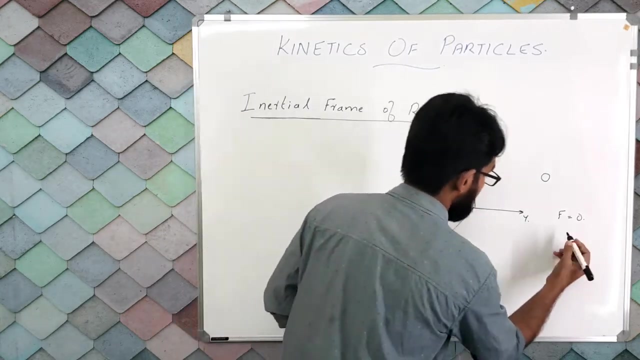 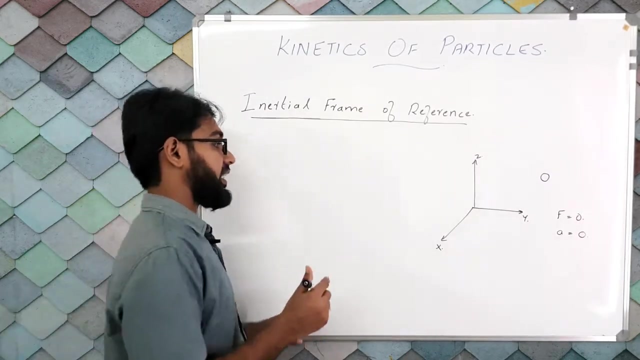 that is at rest with respect to the fixed stars. To understand this concept better, let us consider a particle with no force acting on it. Now the acceleration of this corresponding particle with respect to this reference frame A is equal to 0.. Now let us consider another reference frame. 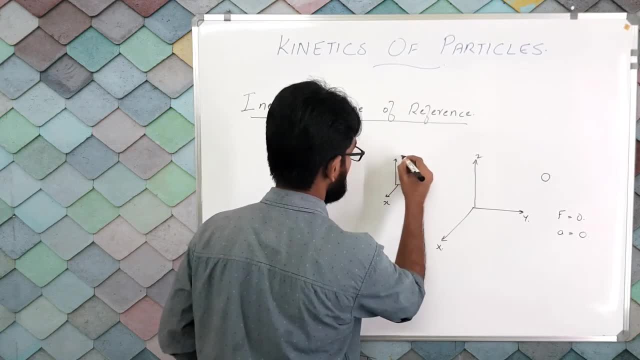 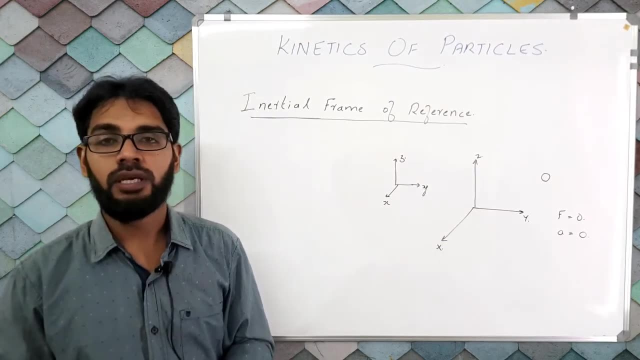 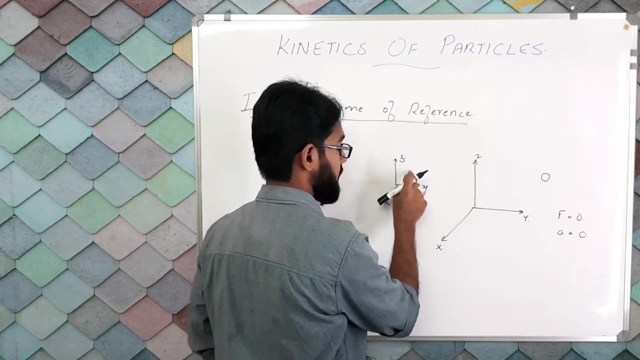 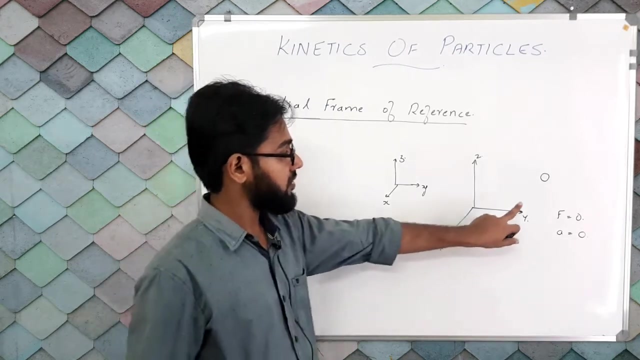 that is accelerating with respect to this primary reference frame. Now, if you see, if you measure the acceleration of this particle with respect to the second reference frame, it will not be 0.. So in this corresponding frame of reference, the Newton's law, 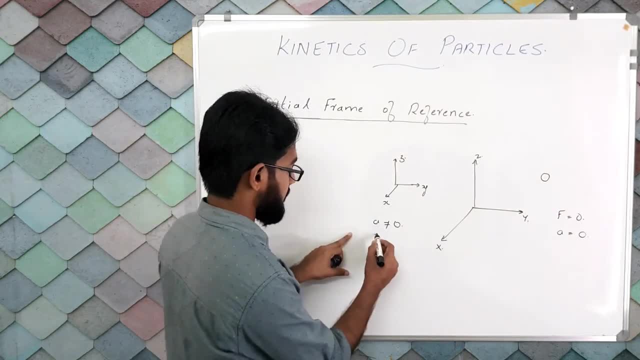 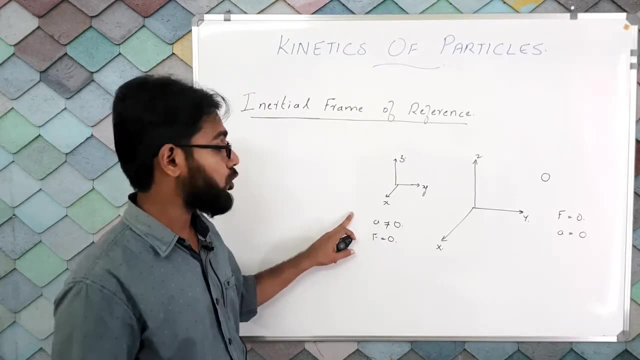 is valid. However, in this case the final reference frame of reference A is equal to 0. In this corresponding reference frame, the Newton's law is not valid, So this gives an error in the Newton's law in case you consider an accelerating frame of reference. 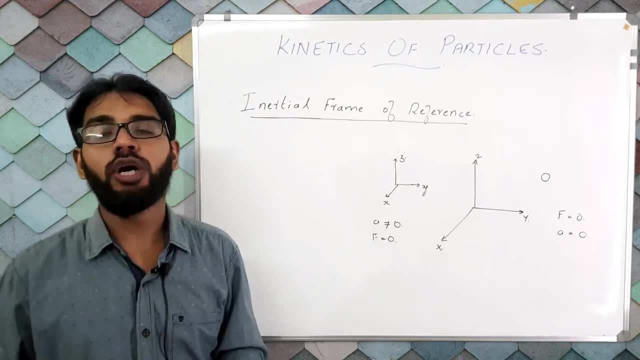 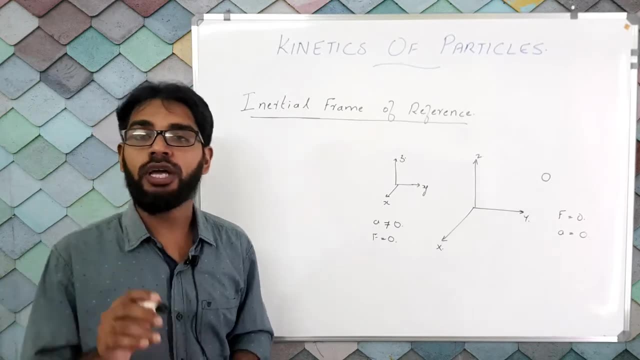 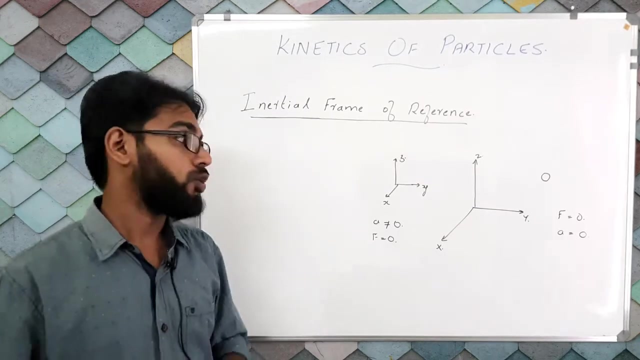 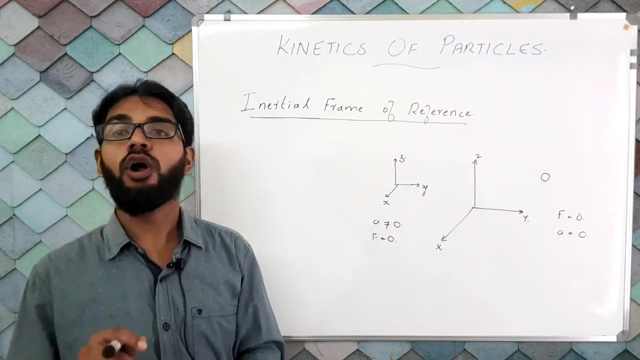 So that is the reason why I stated that the Newton's law cannot be directly applied to all reference frames. A reference frame in which the Newton's law can be applied is called the inertial frame of reference or the Newtonian frame. Now, the acceleration measured with respect to the inertial frame of reference is called absolute. 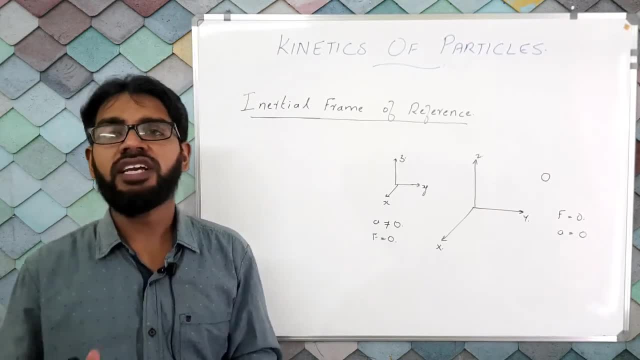 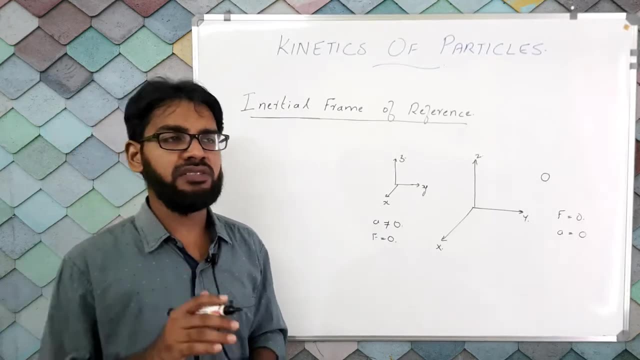 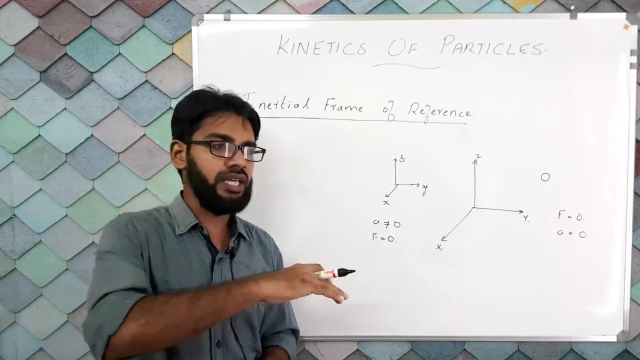 For most of the problems on the surface of the earth, we consider the reference frame fixed to the earth as the inertial frame of reference. This gives us sufficiently accurate results, though there may be small corrections that need to be applied to include the acceleration of the earth. But these corrections are negligible for most of the problems on the surface of the earth and hence we don't consider them in our calculations. However, in the case of motion of, in the case of motion of rockets and, say, precise engineering systems, the acceleration of the Earth also need to be considered. 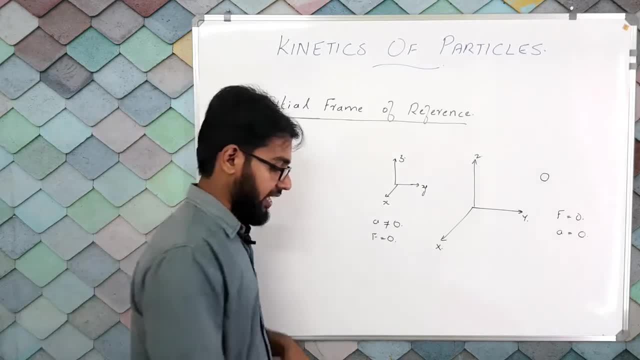 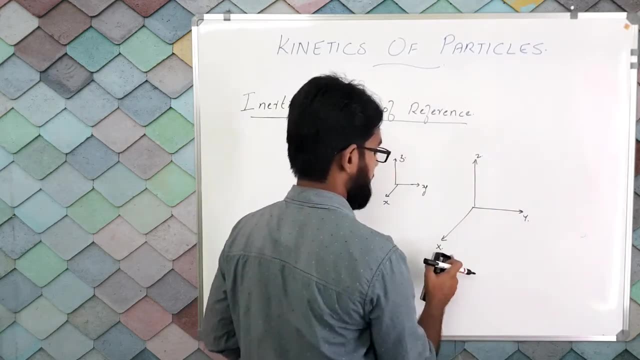 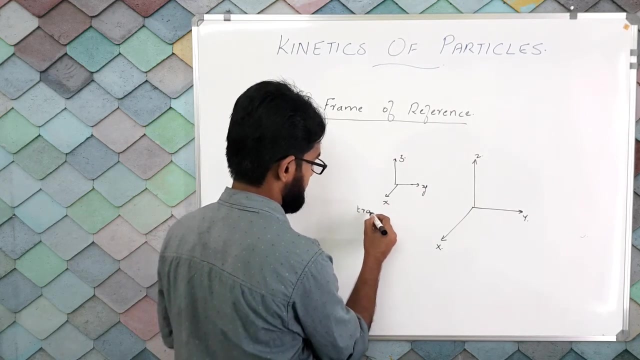 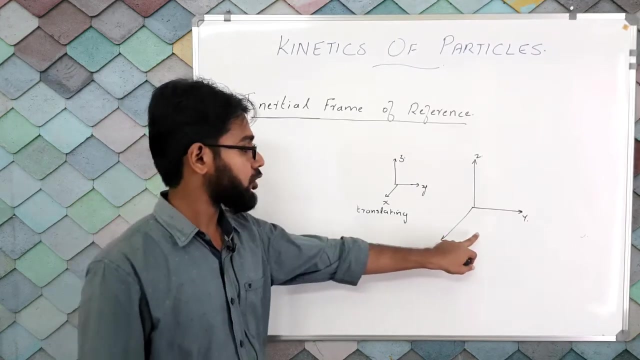 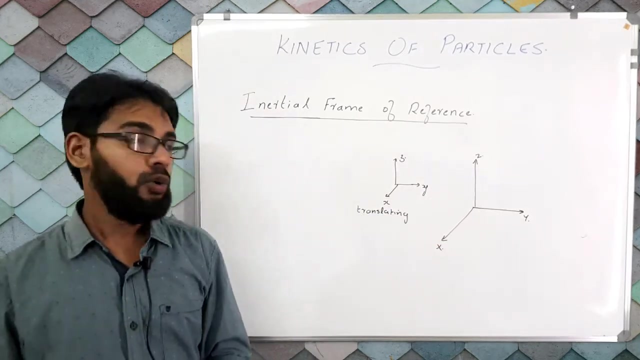 into account. Now suppose I have a primary frame of reference and a corresponding translating frame of reference that is moving with a constant velocity with respect to the corresponding primary reference frame: x, y, z. Now here we can see that the Newton's law is: 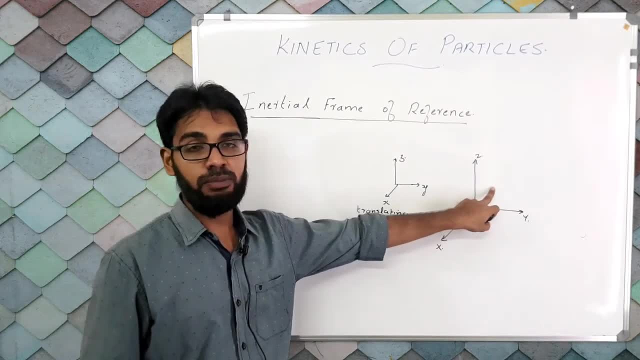 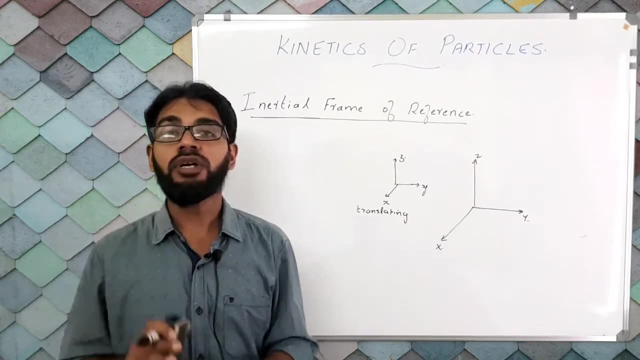 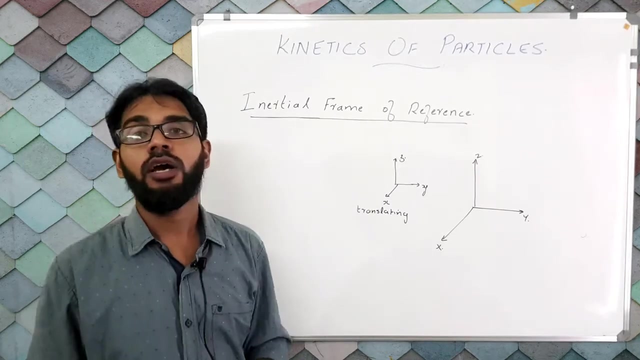 applicable to both the primary inertial frame of reference as well as the translating frame of reference. So in general, we can say that the Newton's laws are valid for all non-rotating reference frames which translate with a constant velocity with respect to the inertial reference. 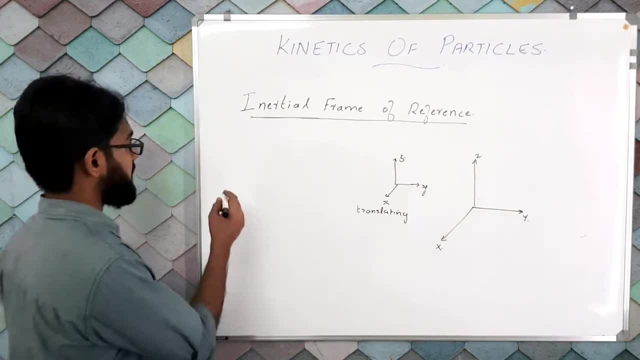 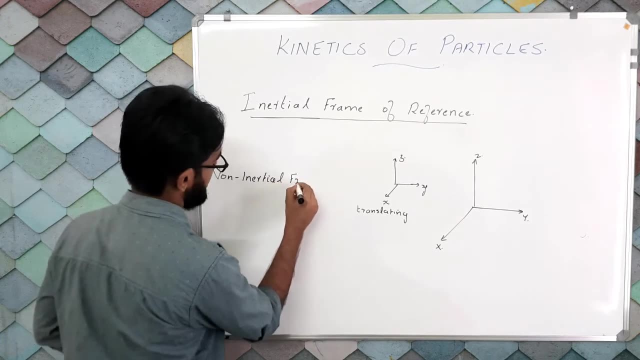 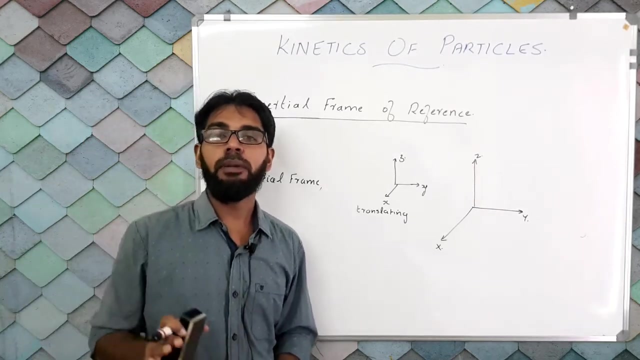 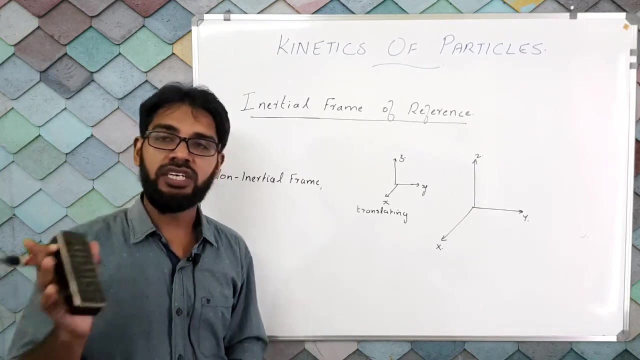 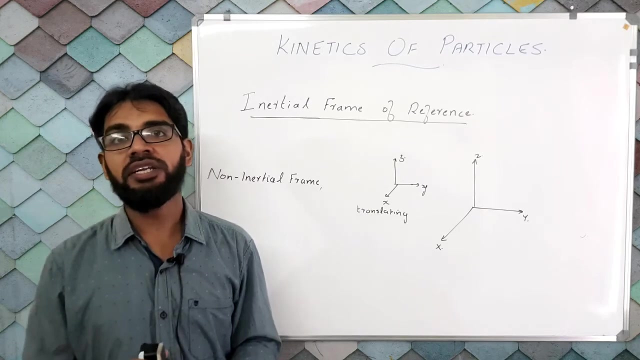 frame In case of a non-inertial frame of reference. here the Newton's second law can be applied by taking into account the acceleration and rotation aspects. We shall discuss more about this topic later, when we deal with kinetics of rigid bodies. Now let us solve a problem here: The mass of the Sierkowski UH-60A. 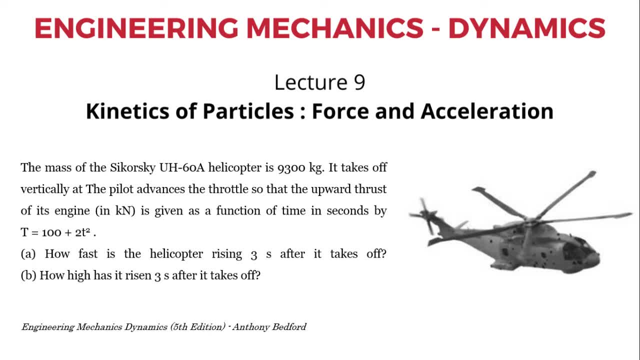 helicopter is 9300 kilograms. It takes off vertically at t equals 0.. The pilot advances the throttle so that the upward thrust of it takes off vertically at t equals 0.. Its engine in kilonewton is given as a function of time in seconds. by t equals 100 plus 2t square. 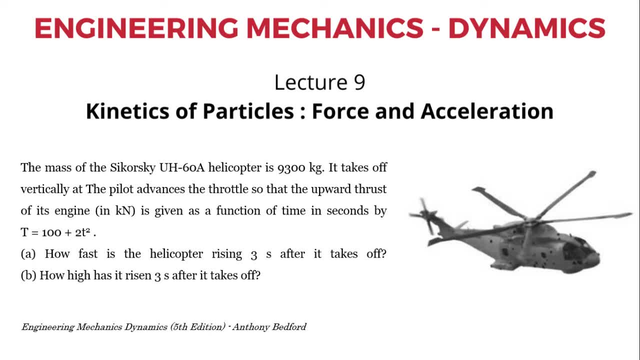 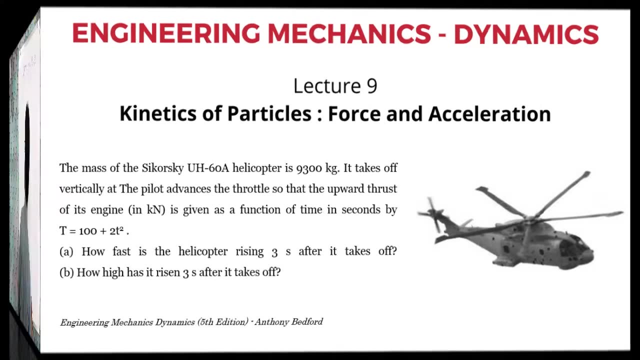 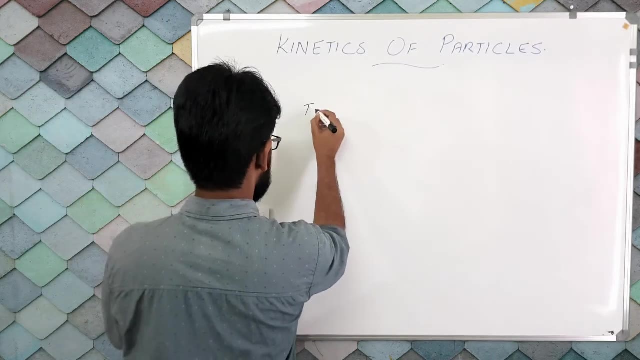 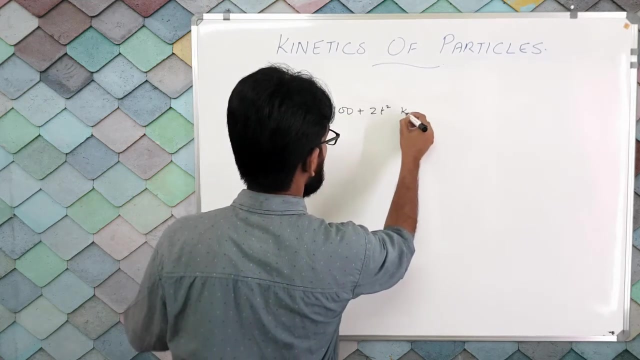 A- How far is the helicopter rising 3 seconds after it takes off? B- How high has it risen 3 seconds after it takes off? This question is from the textbook by Anthony Bedford. Now, given the corresponding throttle, t equals 100 plus 2 t square kilonewton. So if I convert, 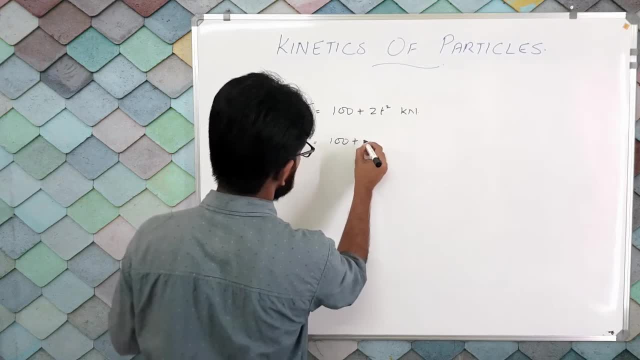 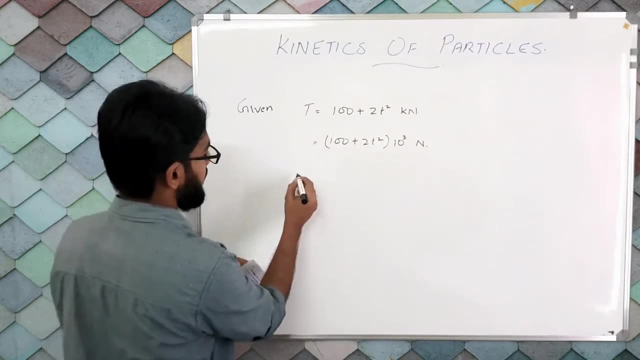 it in Newton. I have 100 plus 2 t square into 10 raised to 3 Newton. The mass of the helicopter is given as 100 plus 2 t square into 10 raised to 3 Newton. So this is the mass of the helicopter. 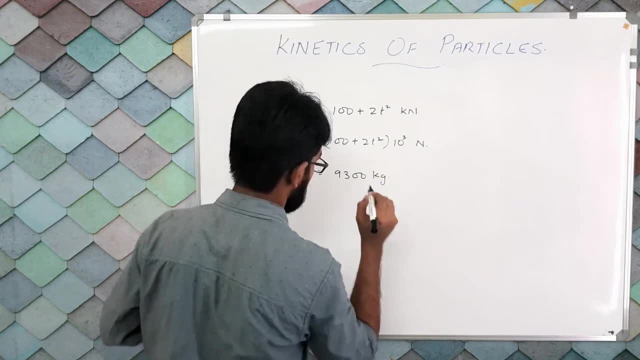 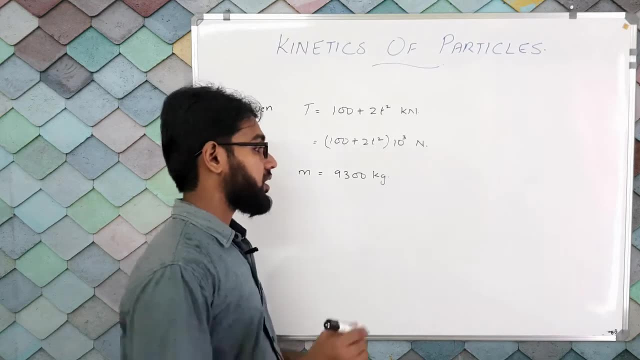 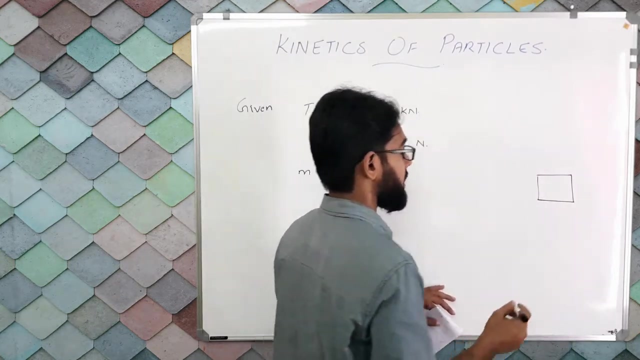 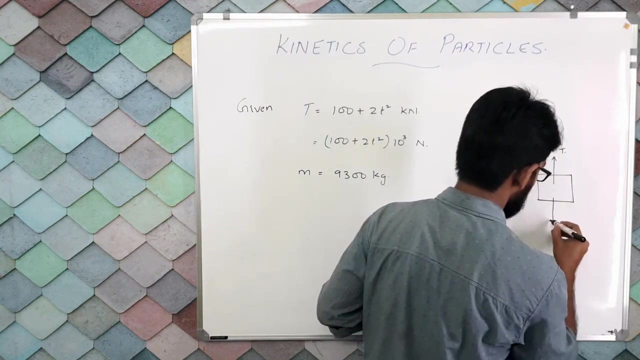 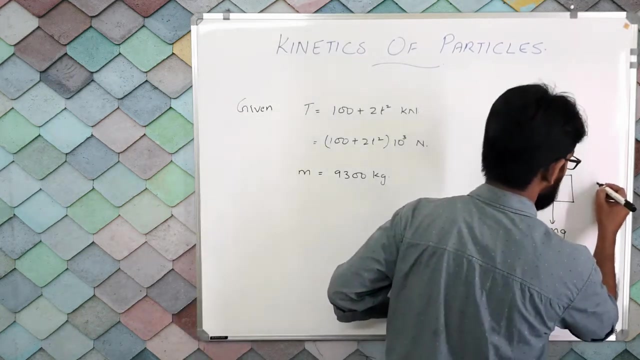 as 9,300 kilograms. When we deal with questions of kinetics it is important that you first draw the free body diagram. So I have here the corresponding thrust acting upwards and the corresponding weight of the helicopter acting downwards: mg. Now the motion is in the upward. 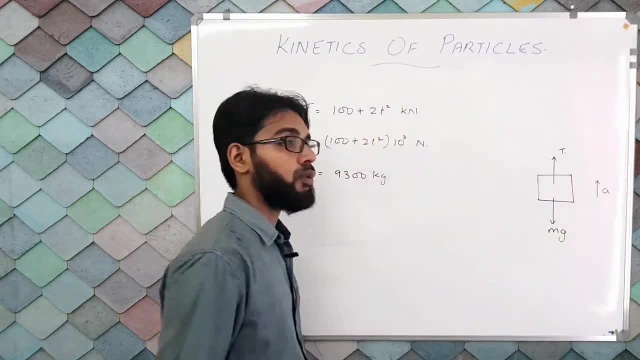 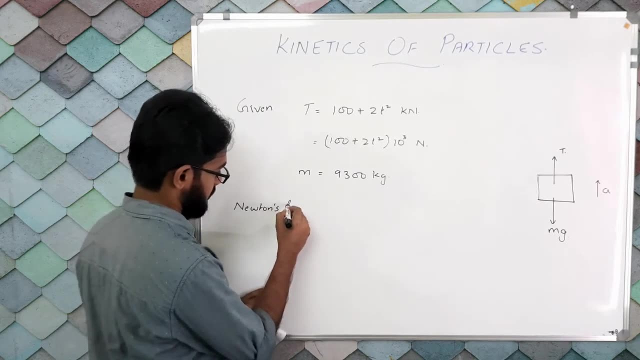 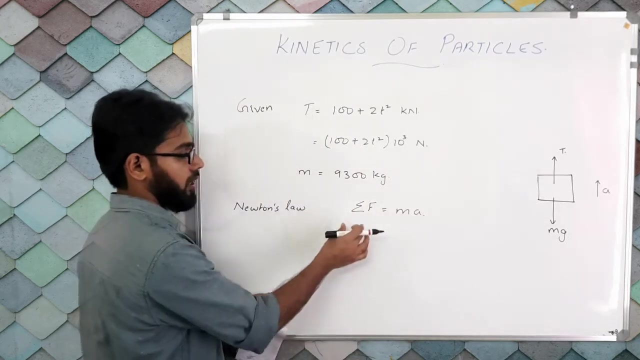 direction, acceleration. hence I had drawn in the upward direction. Now, applying the Newton's law, sigma f equals m into a. Now sigma f is actually the force of the helicopter acting downwards. So I have drawn in the upward direction Now. 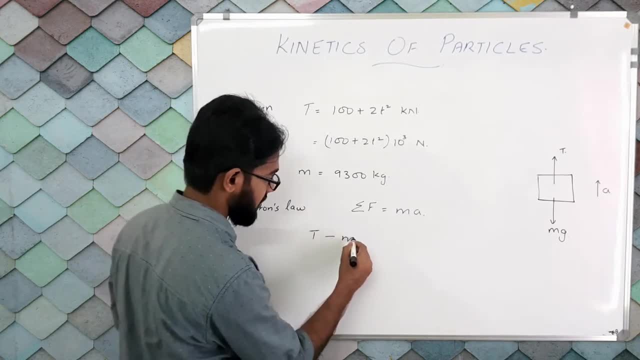 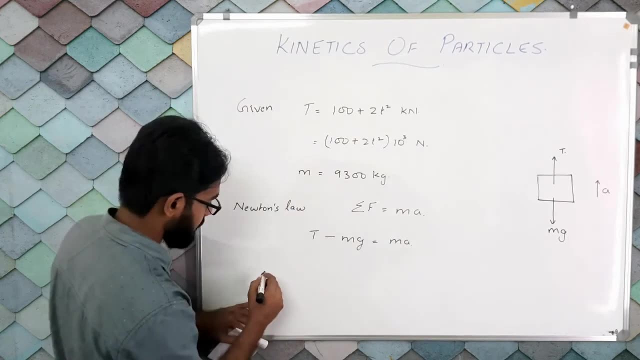 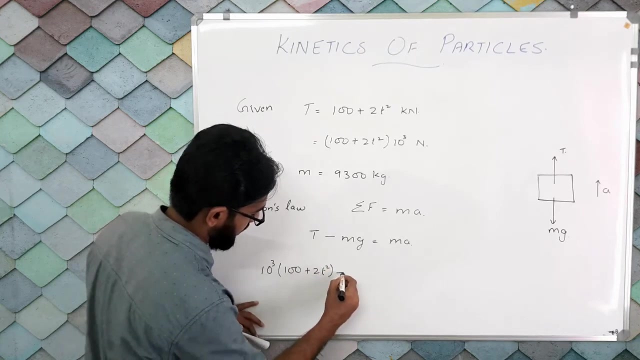 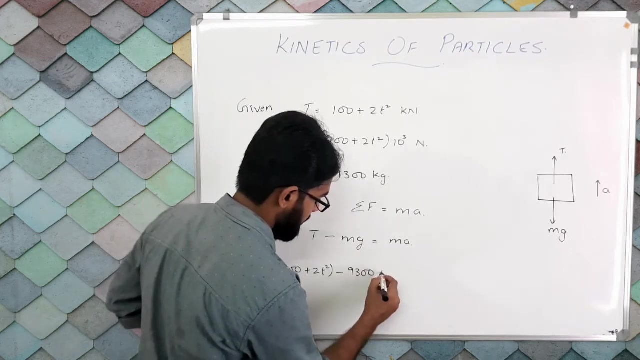 the thrust t minus the weight mg, which is equal to ma. Now thrust t is equal to 10 raised to 3, 100 plus 2 t square minus mass, it is 9,300 kilogram into g, 9.81 meter per second square. 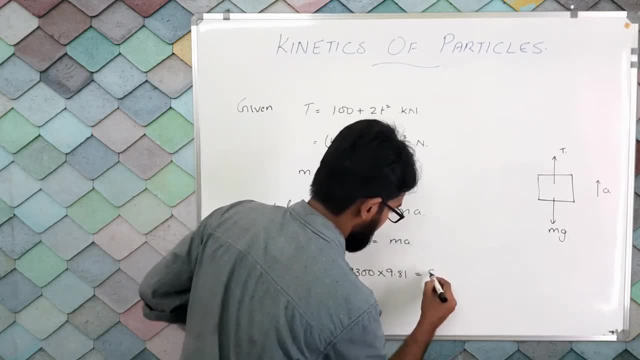 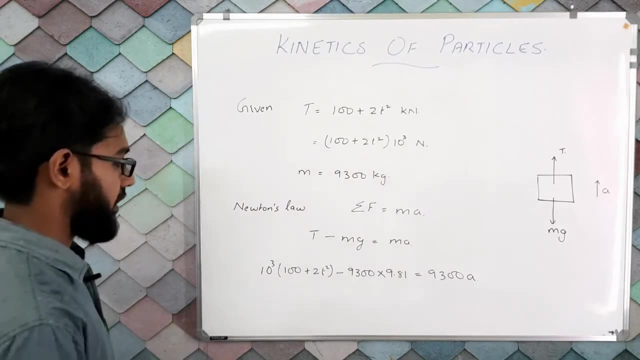 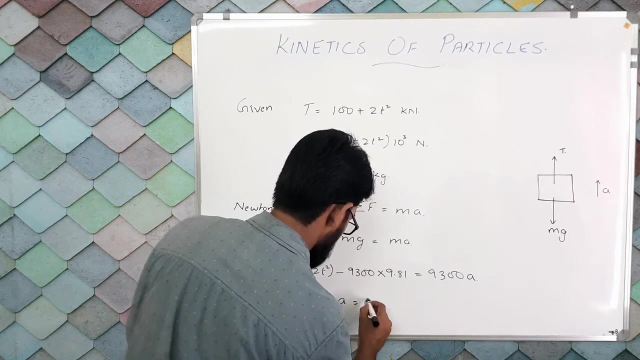 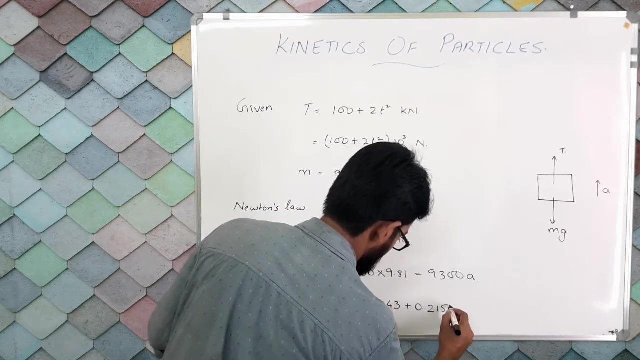 which is equal to mass: 9,300 kilogram multiplied by the acceleration which we have to find out Now. if you solve this, you will get the answer. a equals 0.943 plus 0.215 t square meter per second. 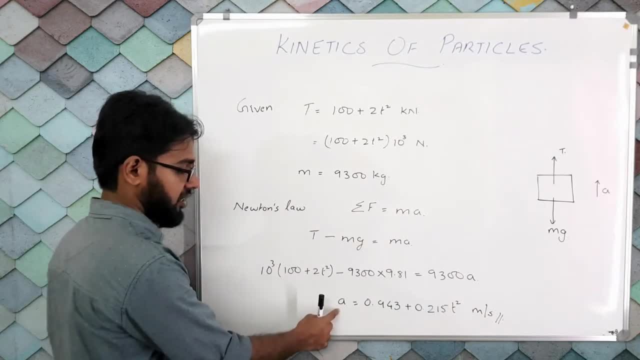 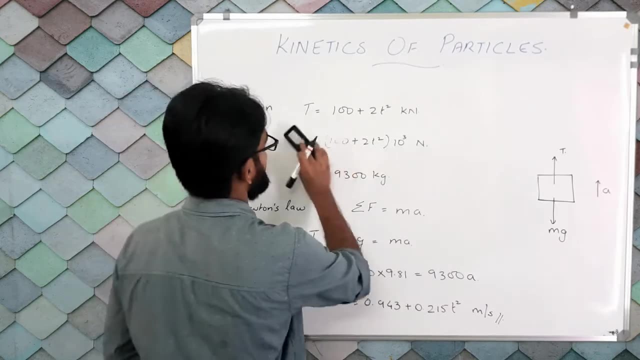 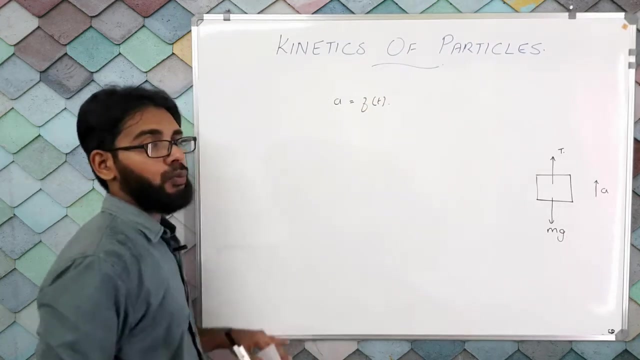 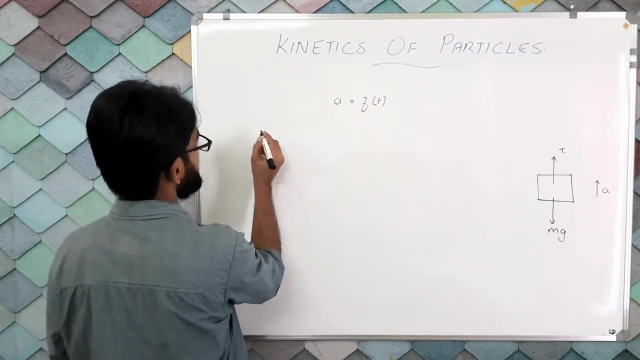 Now, if you look closely, acceleration is a function of time here. Acceleration is a function of time here. Now we had already studied the corresponding integral equations when acceleration is a function of time. So applying these equations here, first I apply the equation. 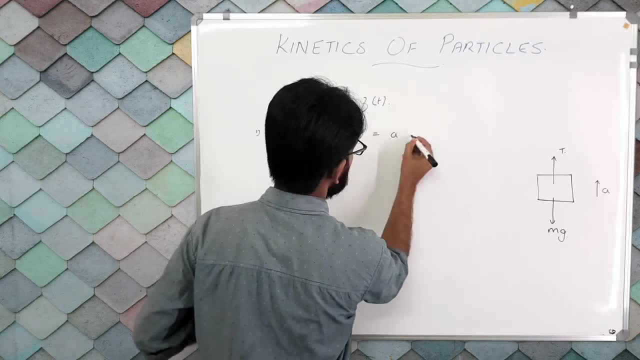 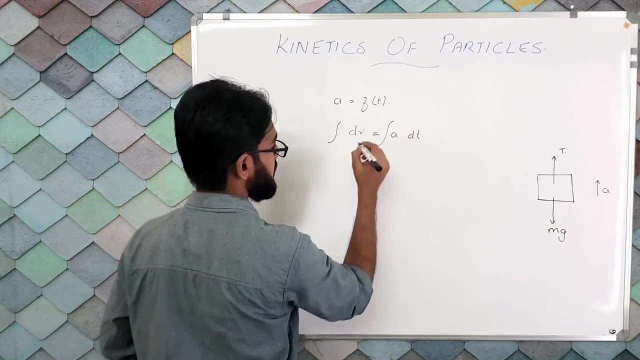 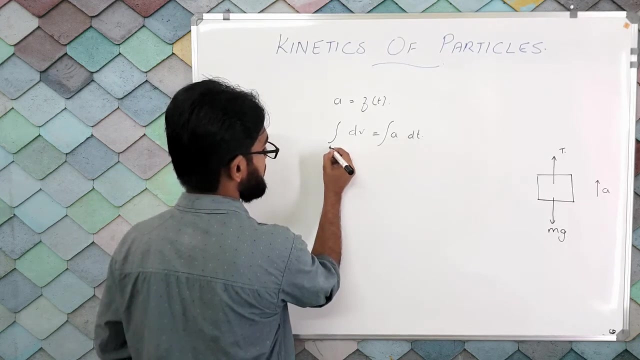 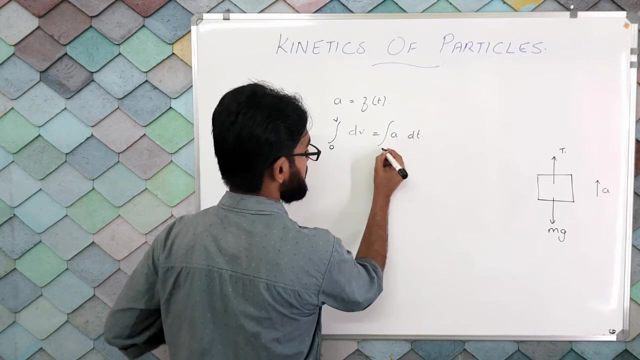 dv. dv equals a, dv, where a is the function of time. So I can integrate both sides Here. on the left-hand side, the corresponding velocity- initially it is 0 to the final velocity, v. Now. on the right-hand side, time from 0 to time. t equals 3 seconds. Now, if I apply this, 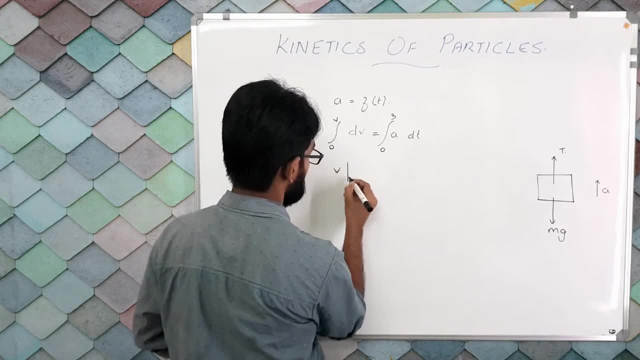 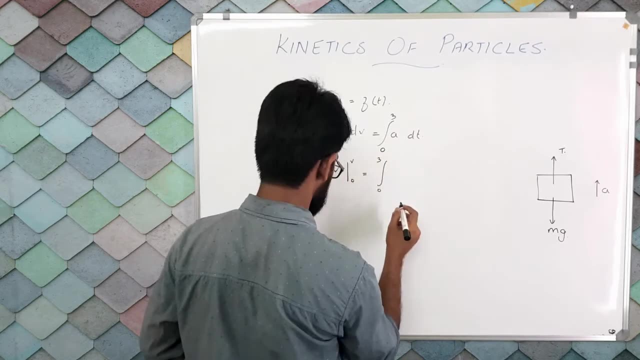 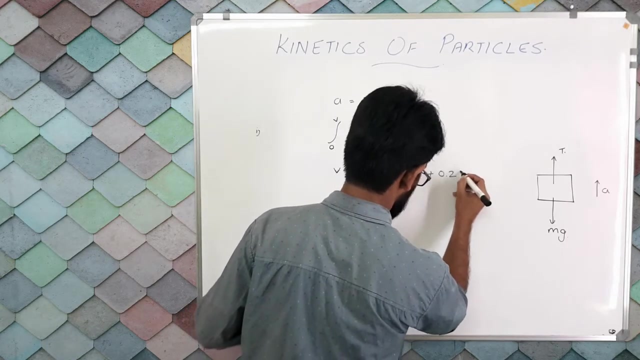 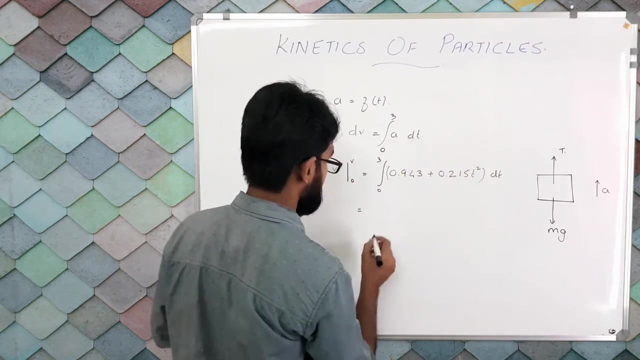 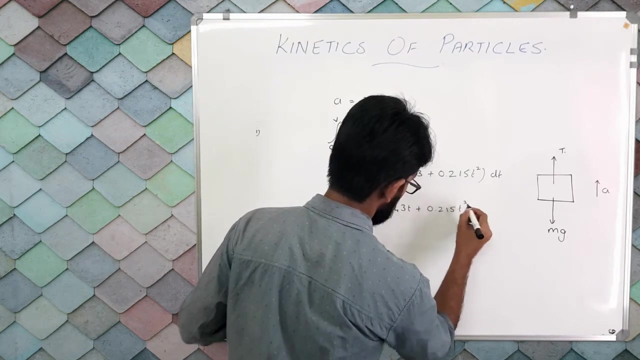 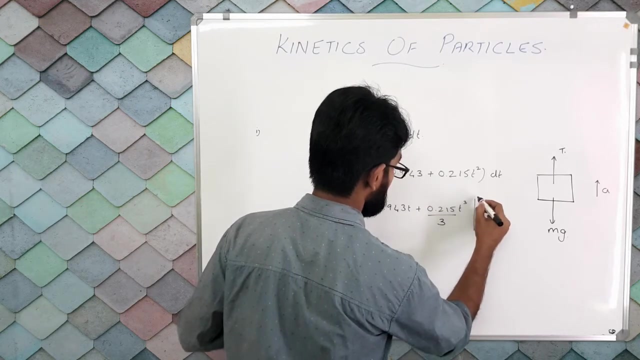 dv v is equal to acceleration. if I remember, it is 0.943 plus 0.215 t square dt. If I integrate I will get 0.943 t plus 0.215 t cube by 3 from time 0 to 3 seconds. 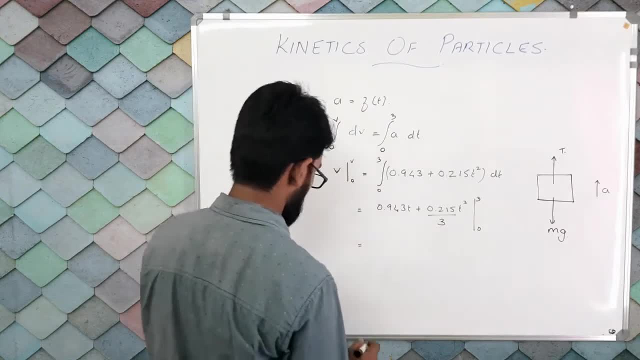 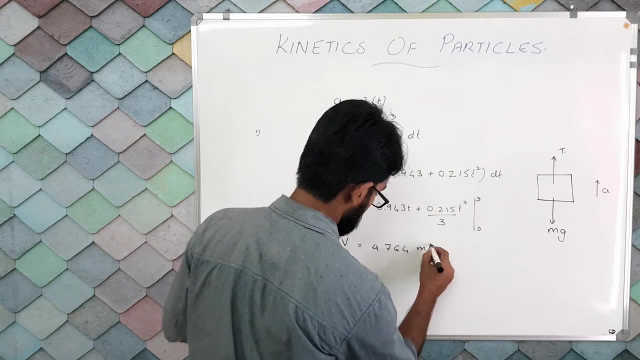 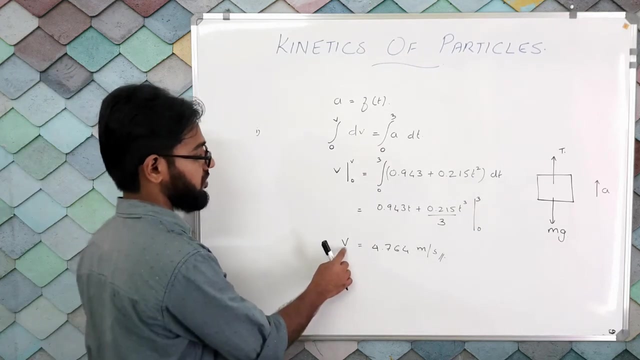 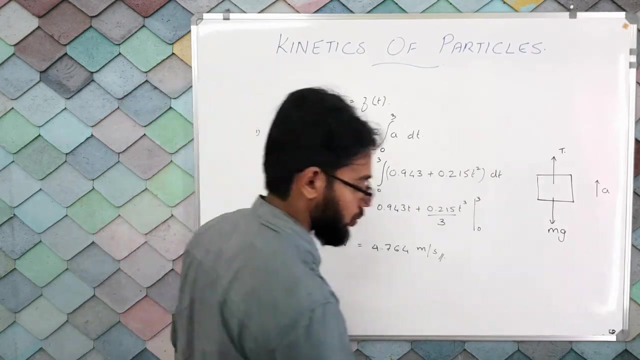 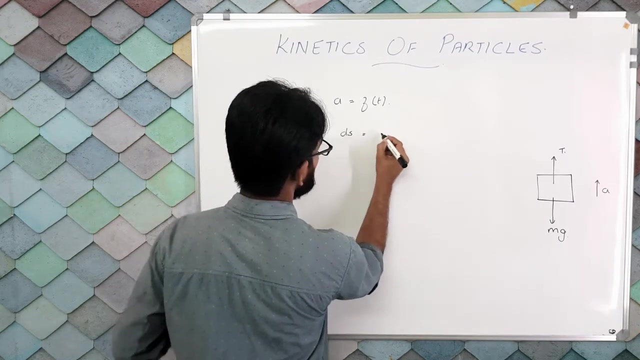 Now, if I substitute this corresponding value, we get v equals 4.764 meter per second. So this is the corresponding velocity at that time Instant, when time t equals 3 seconds. Now moving on, The second equation which we can apply here is: ds equals v. 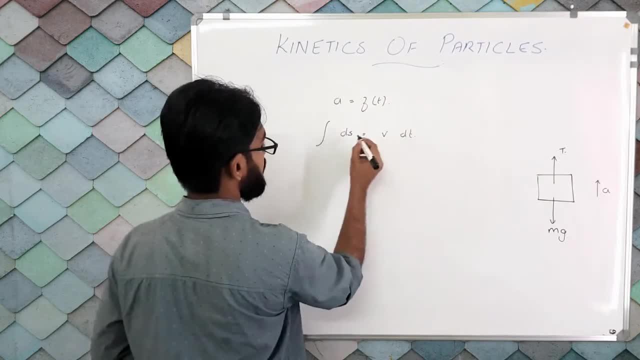 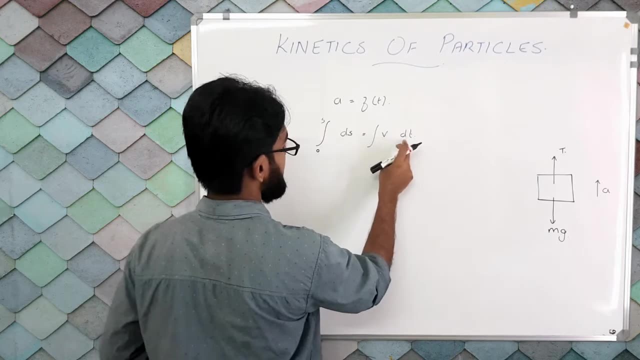 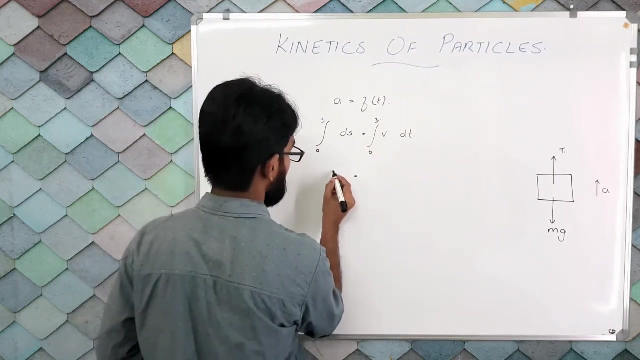 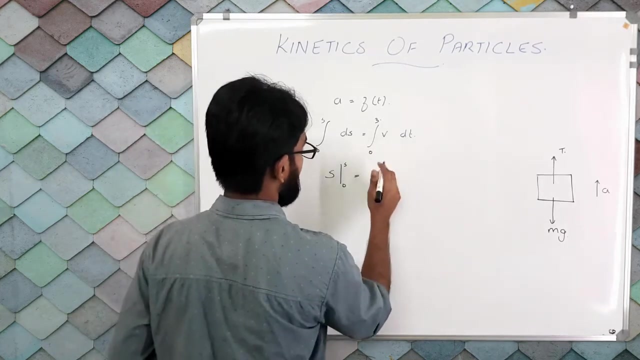 dt. So if I integrate on both sides ds, initially the integral from 0 to s, dt from time, t equals 0 to 3 seconds. Now this will give a value s from 0 to s. Now v is actually the corresponding function of time. 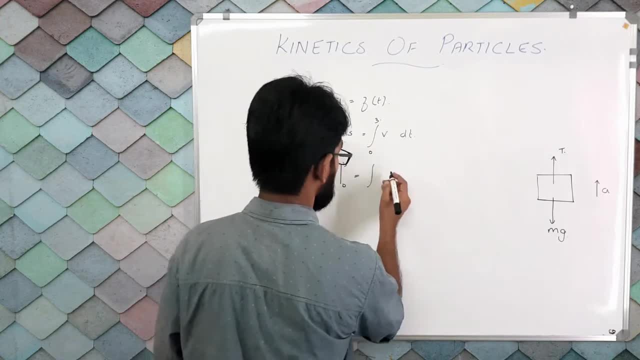 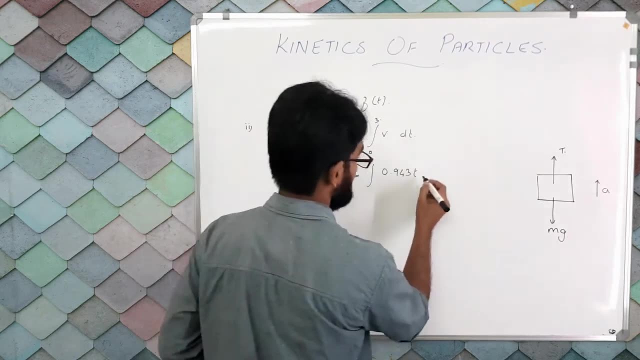 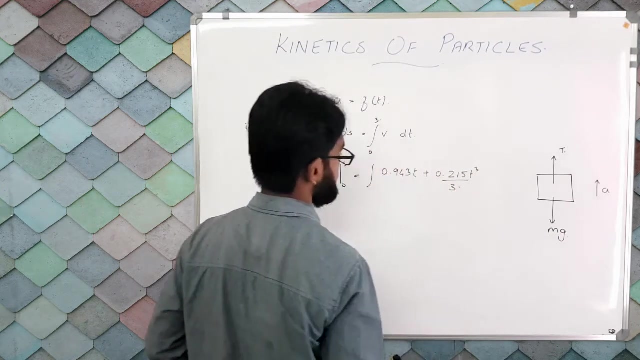 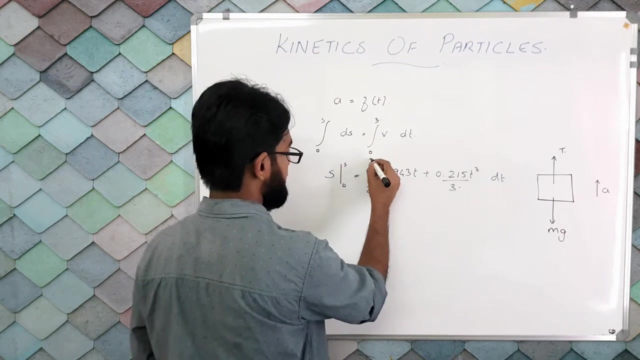 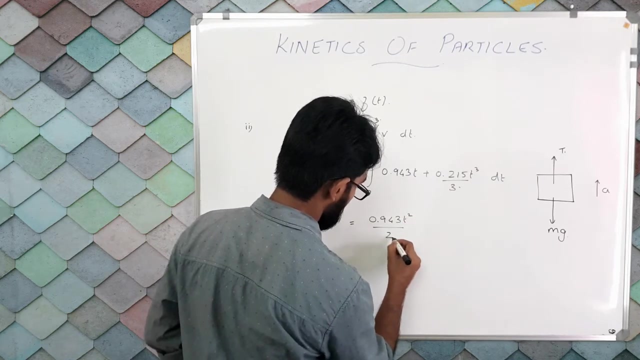 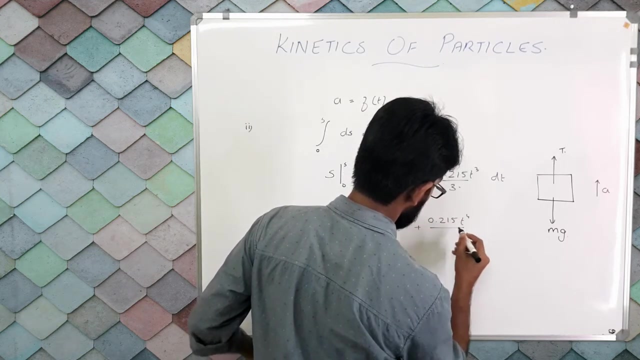 So this corresponding v we can get from the previous equation. From the previous equation we get v equals 0.943 t plus 0.215 t cube by 3.. So by州 sounds like this. Now, if I integrate this I would get: 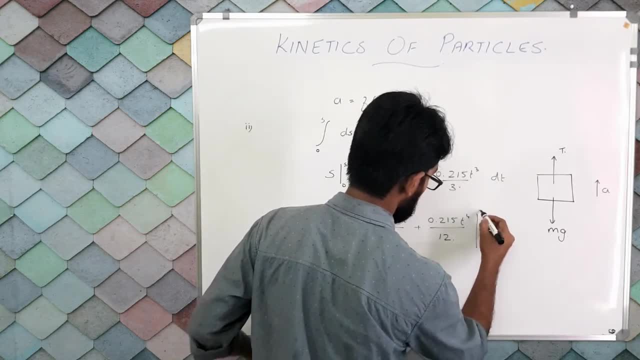 0.943 t square by 2 plus 0.215.3 raise to 4, divided by 12, from time 0 to 3.. If you solve this corresponding equation, you will get 0.943 t square by 3 plus 0.215.3 raise to 4 minus 0.943 t cube by 3.. So if we integrate the sum of the two elements, we will get 0.943 t cube by 3.. So if I integrate this, I would get 0.943 t cube by 2 plus 0.215 t cube by 3.. 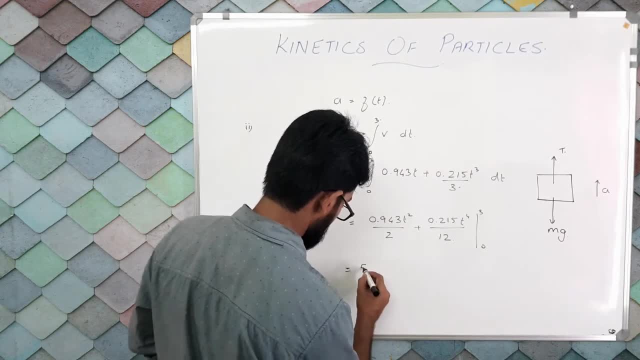 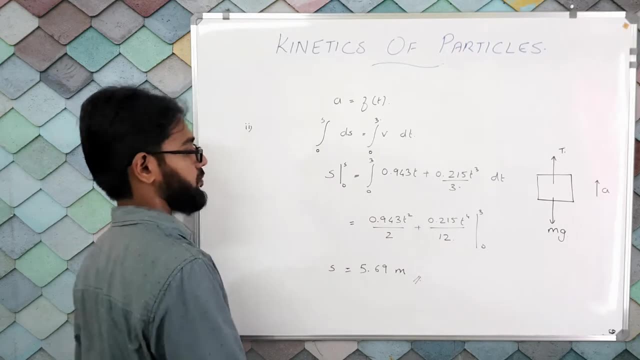 Now, if I integrate this, I would get 0.943 t cube by 3.. Now, if I integrate this, I would get 0.943 t cube by 3.. corresponding equation: we would get s equals 5.69 meters, So v equals 4.674 and the corresponding 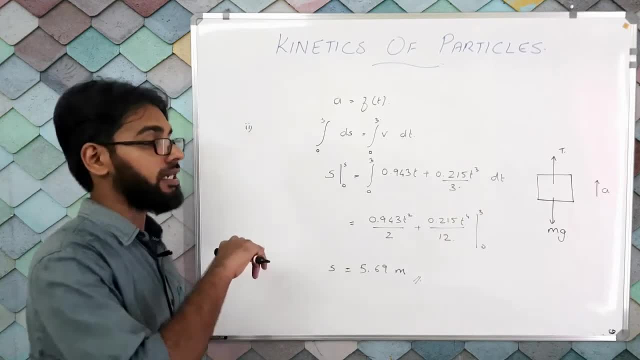 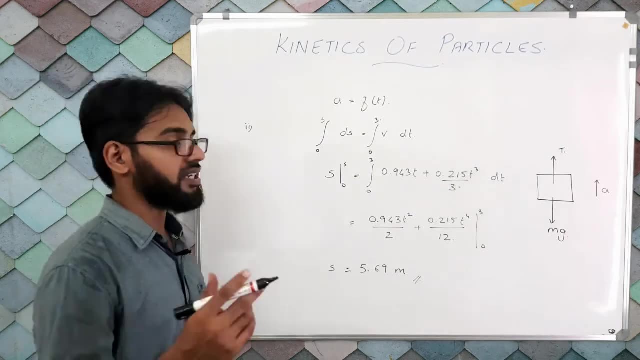 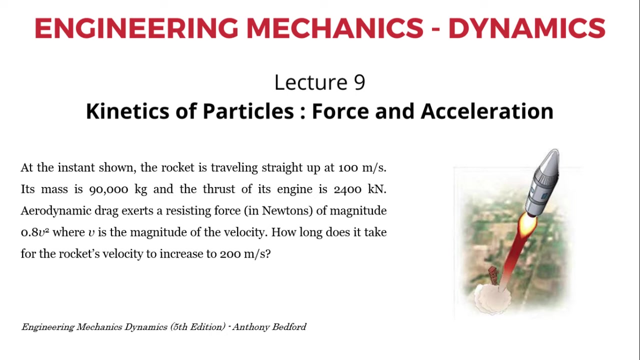 s equals 5.69 meters. at the end of the time, t equals 3 seconds. Now, moving on to a second question. At the instant shown, the rocket is traveling straight up at 100 meters per second. Its mass is 90,000 kilograms and the thrust of its engine is 2,400 kilonewton. 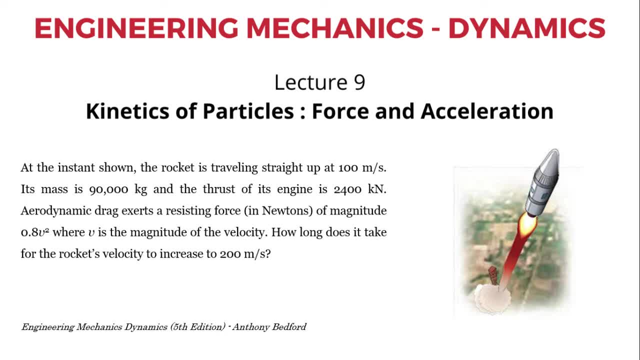 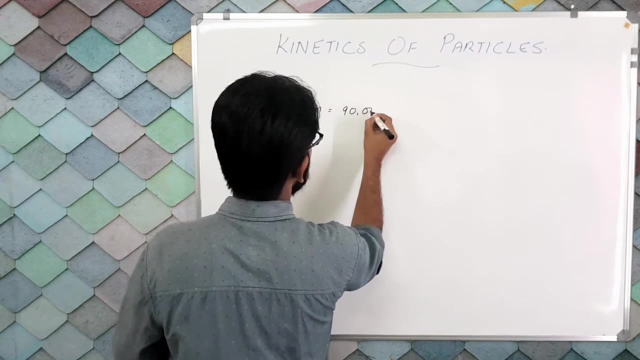 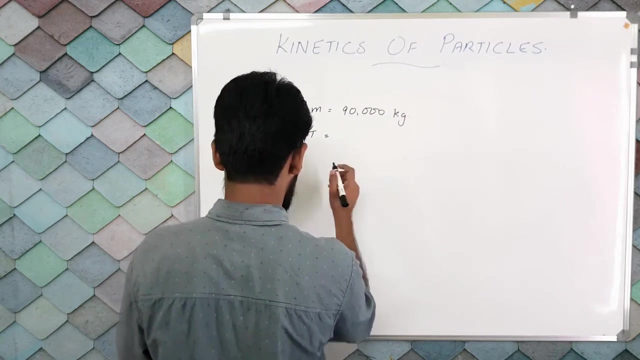 Aerodynamic drag exerts a resisting force in newtons of magnitude 0.8 v square, where v is the magnitude of the velocity. How long does it take for the rocket's velocity to increase to 200 meters per second? Given m equals 90,000 kilograms. the corresponding upward thrust, t, equals 2,400. 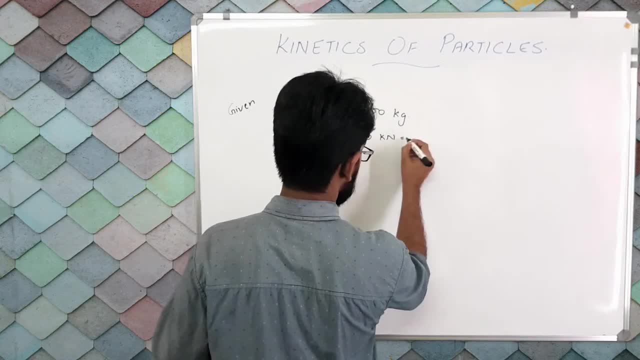 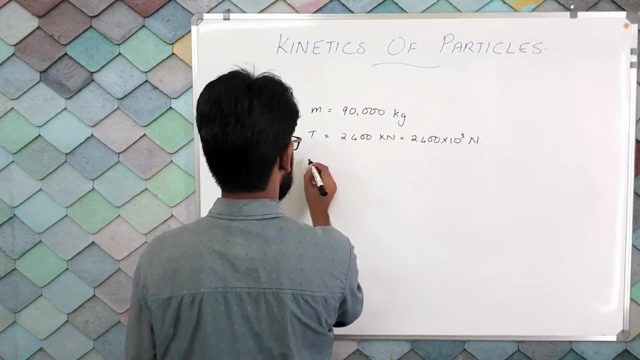 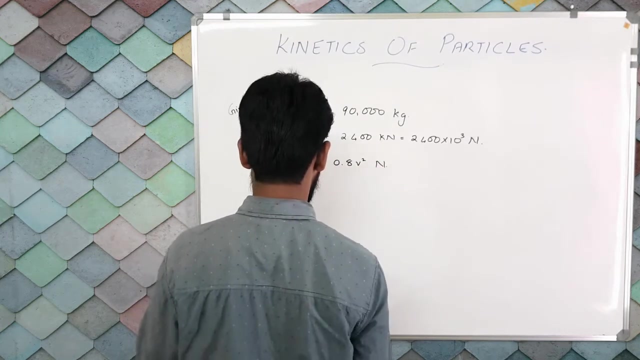 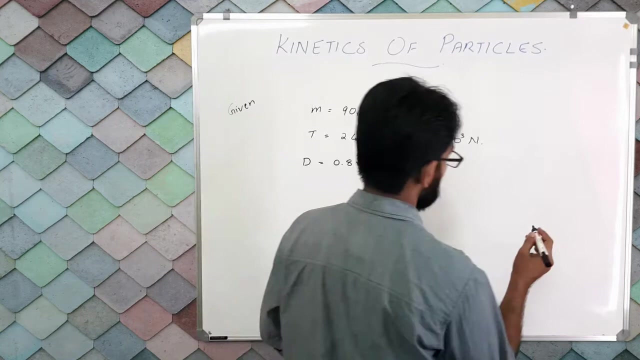 kilonewton, This will turn out to be 2,400.. Now the corresponding aerodynamic drag d equals 0.8 v square newton. Now, as I told you, in any such question, the first thing we have to draw is the free ball diagram. So here we have the 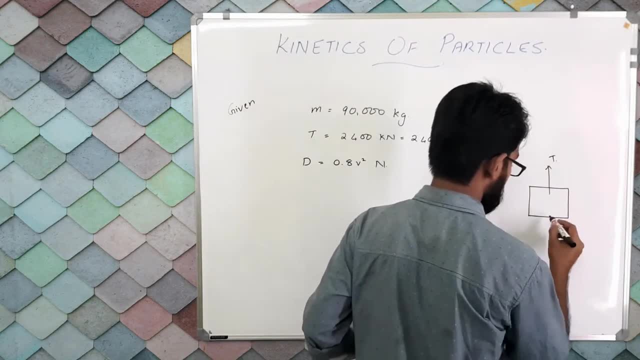 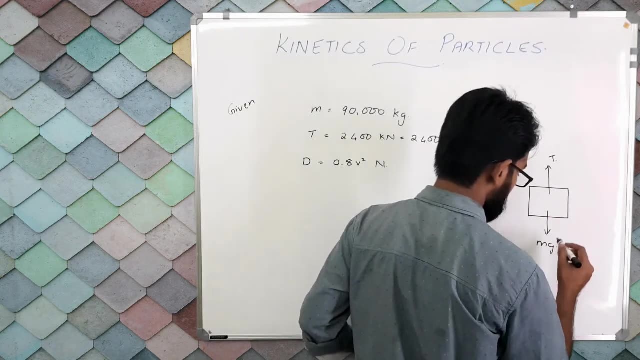 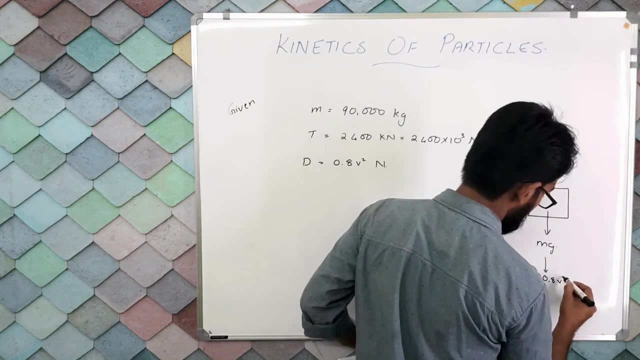 corresponding thrust t in the upward direction. Now the corresponding aerodynamic drag d equals 0.8 v square newton And the weight mg. in the downward direction you also have the corresponding drag force, 0.8 v square. 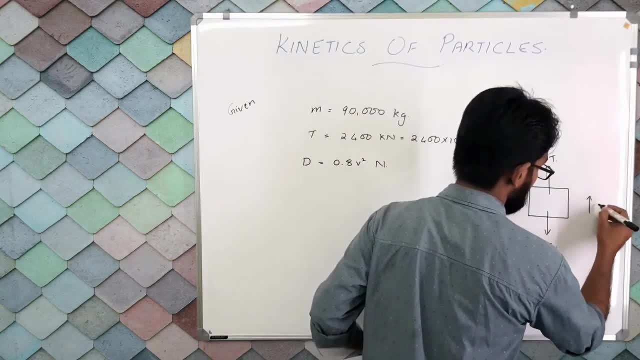 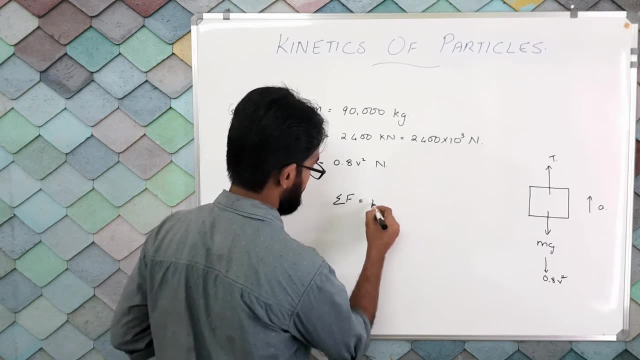 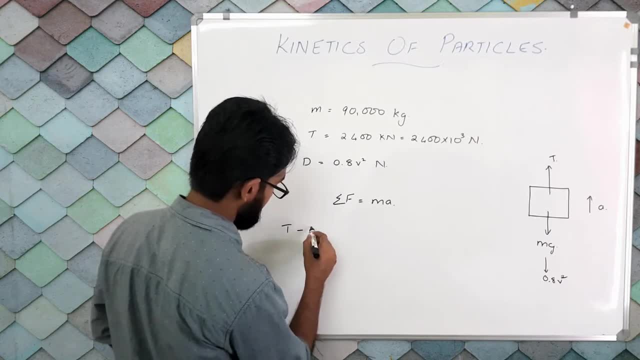 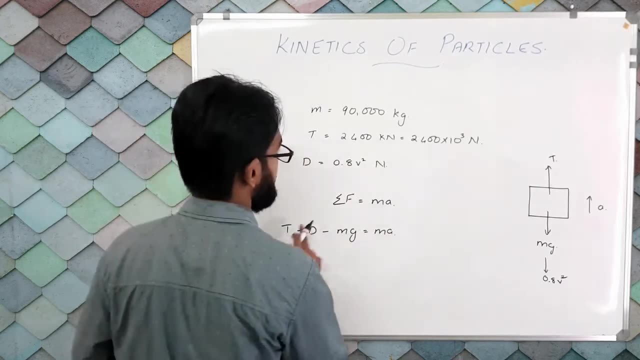 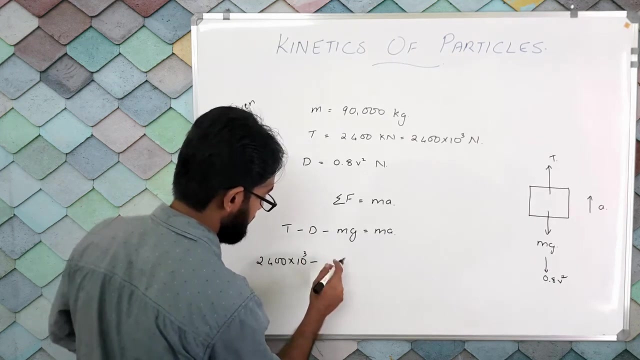 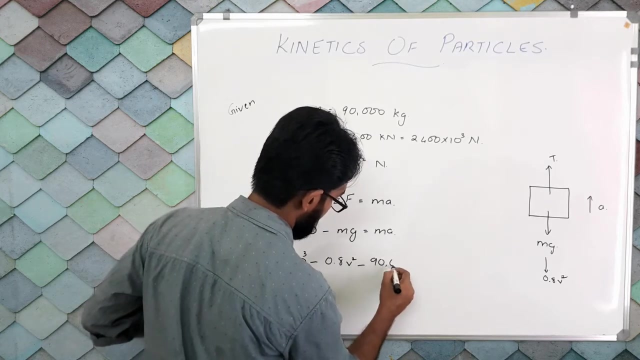 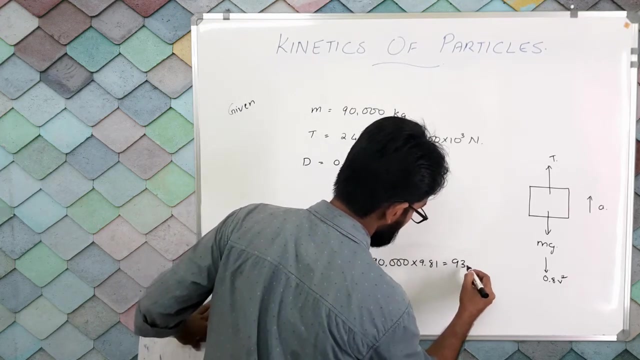 sigma F equals m. a will be equal to T minus D. minus Mg is equal to Ma. Now T it is 2400 into 10. raised to 3 minus D, it is 0.8 V square minus M 90,000 kilogram. G 9.81 is equal to M 90,000 kilogram into A. 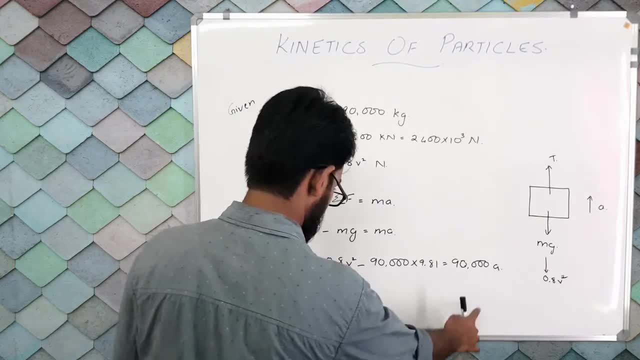 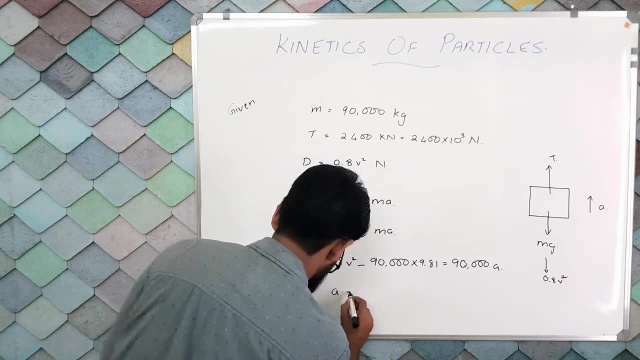 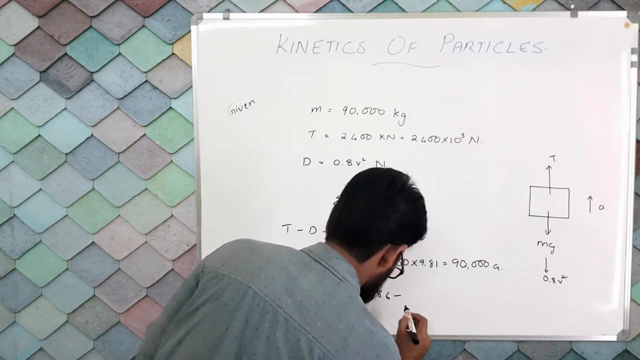 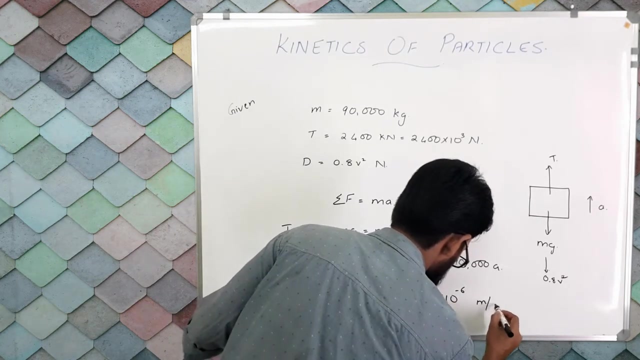 So now, if, if you solve this, you can get the corresponding acceleration in terms of a function of velocity. So if I solve it out, I will get A equals 16.86 minus 8.89 into 10, raised to minus 6 meter per second square. 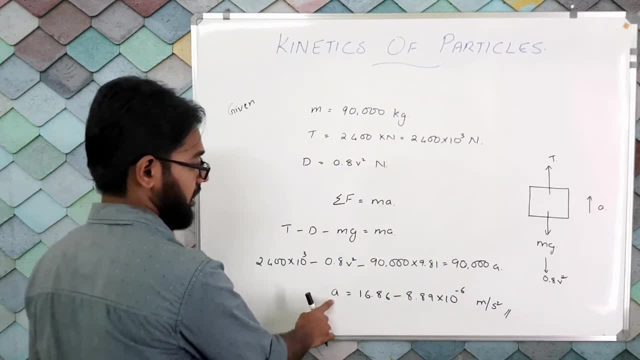 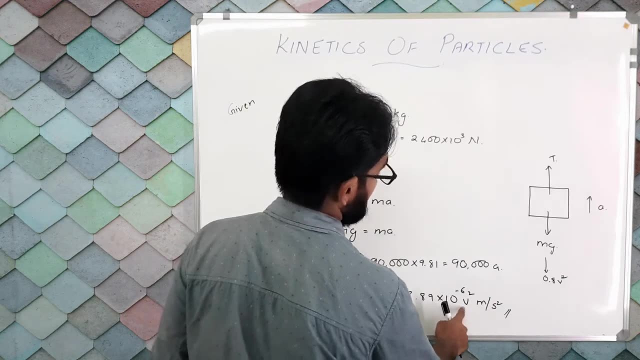 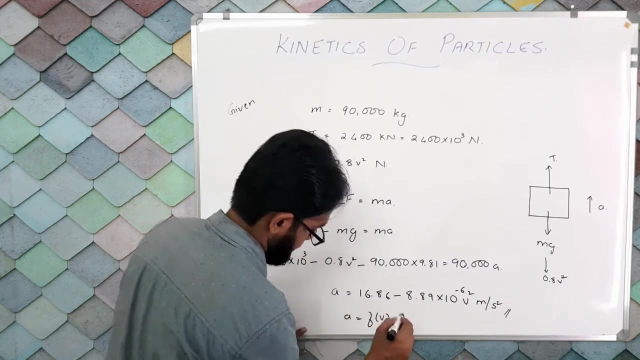 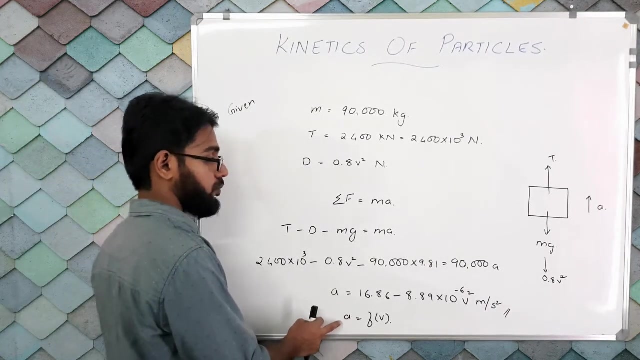 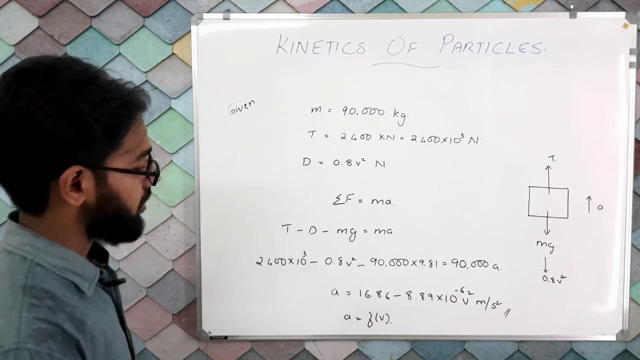 So here I get the corresponding acceleration In terms 8.89 into 10, raised to minus 6 V square meter per second square as a function of velocity. So we can apply the integral equations for this corresponding equation to obtain the value of time at the end of 200 meter per second. 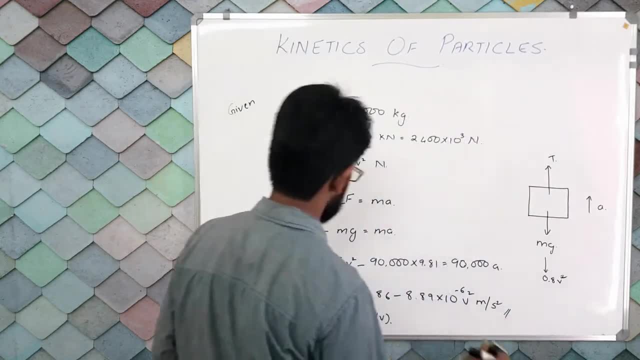 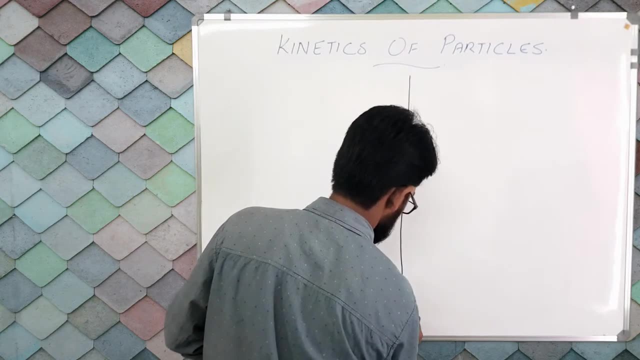 So we can apply the integral equations for this particular equation to obtain the value of time at the end of 200 meter per second square. So we can apply the integral equations for this particular equation to obtain the value of time at the end of 200 meter per second square. 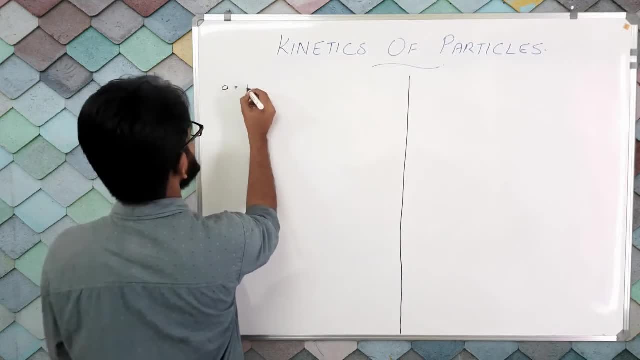 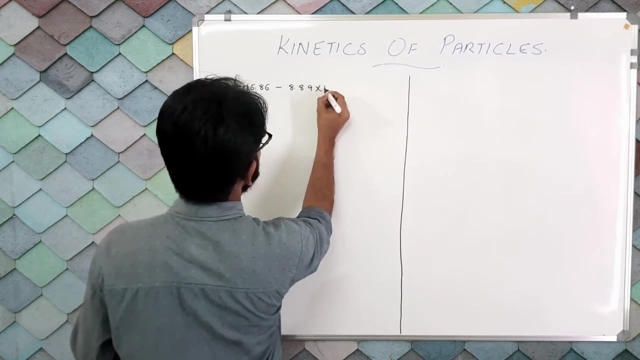 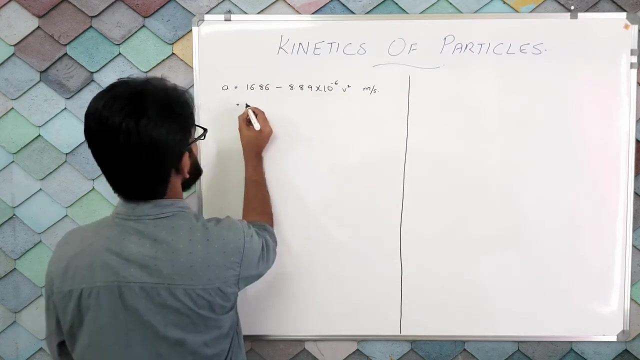 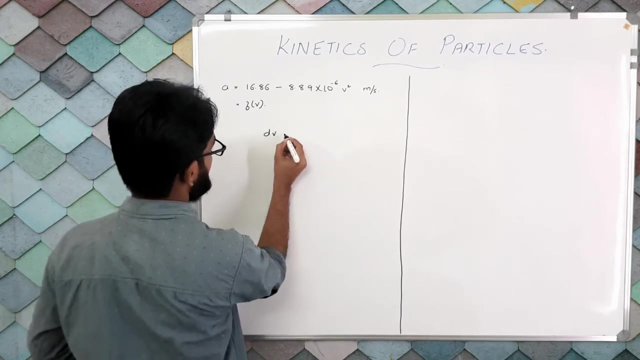 Now, given: A equals 16.86 minus 8.89 into 10, raised to minus 6, V square meter per second, which is a function of velocity, t. Now, if I use the corresponding equation, dv equals a, dt, where a is a function of velocity. 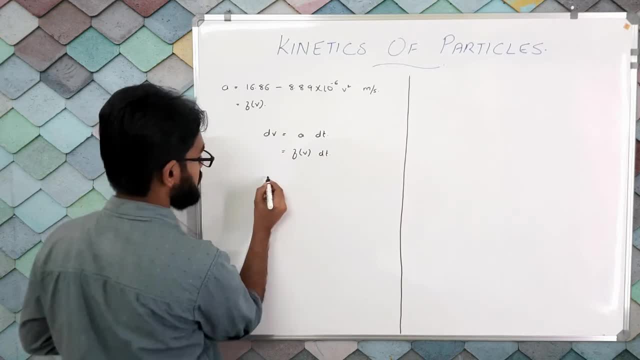 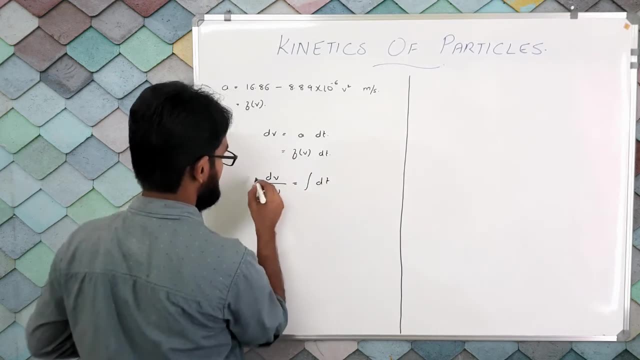 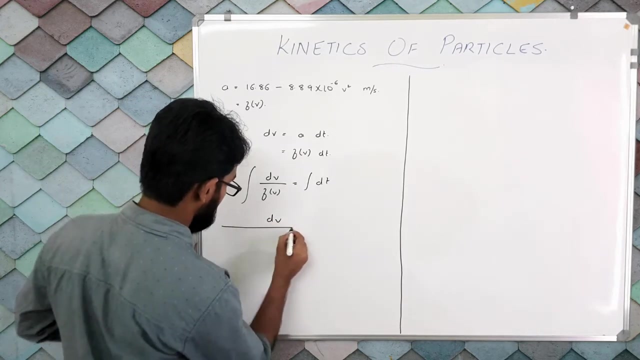 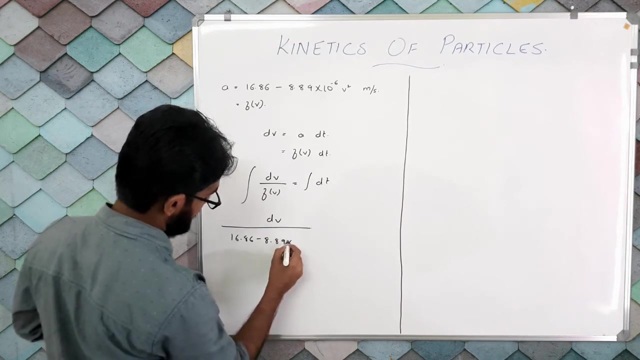 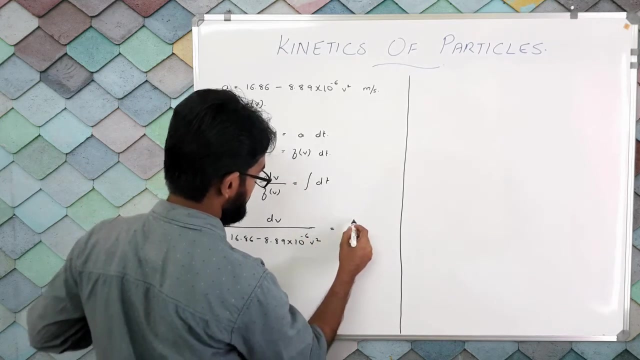 I can bring this corresponding fv downwards. So dv by f of v is equal to dt integrating both sides. So dv divided by 16.86 minus 8.89 into 10, raised to minus 6 v square, is equal to integral dt. 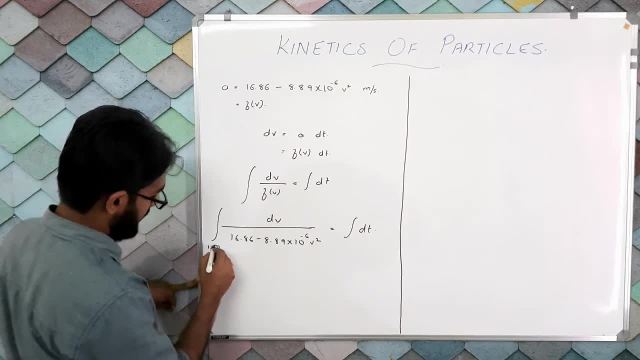 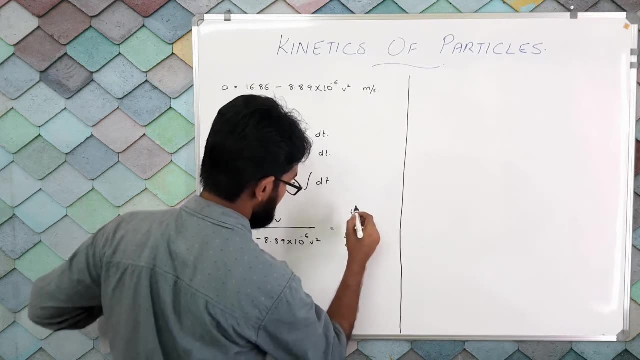 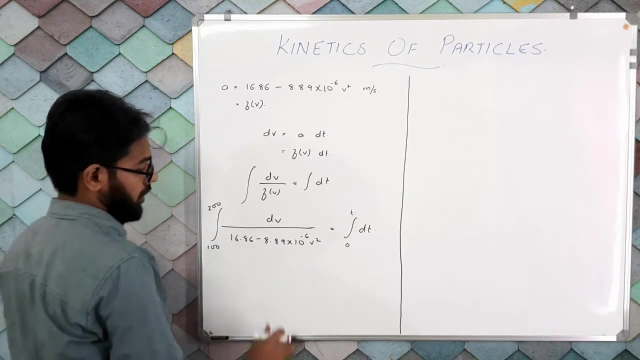 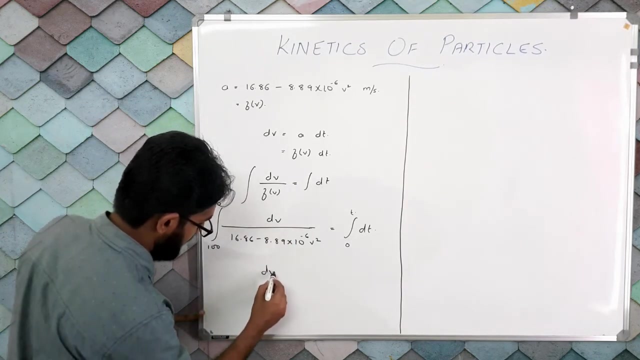 Now the limits are from 100 meter per second to 200 meter per second, Their time from 0 to 0.. Now, if you look at this corresponding integration, you can express this equation in the following format: dv divided by a square minus x square. 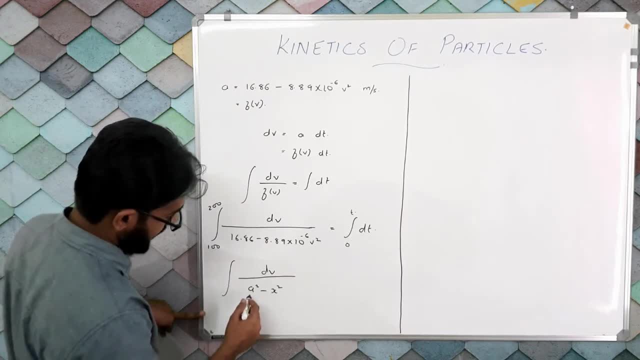 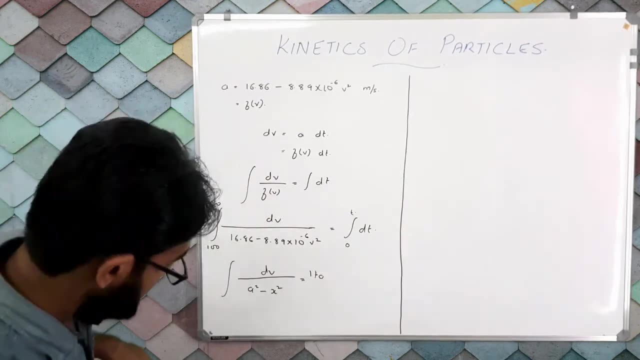 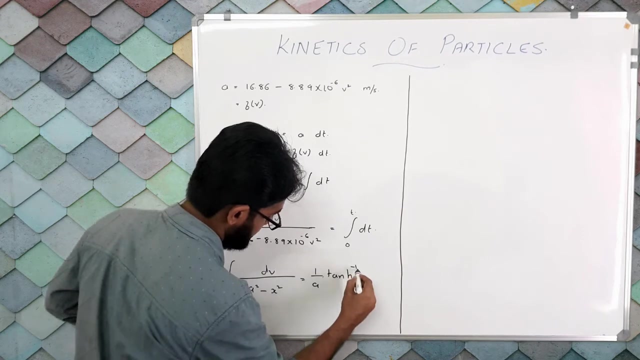 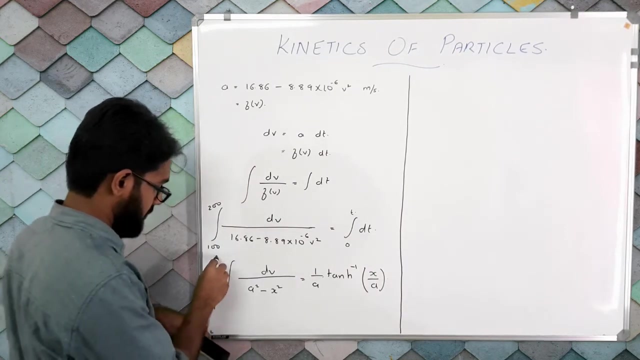 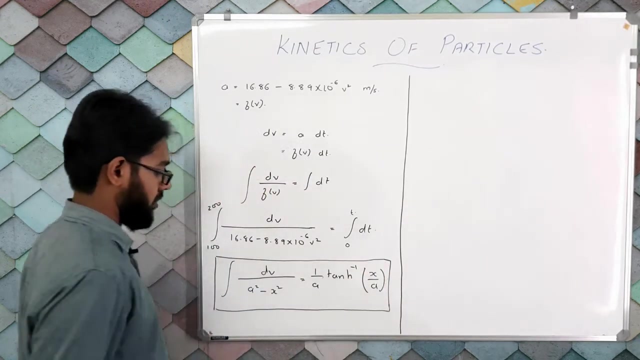 Now, integral of dv divided by a square minus x square is equal to 1 by 2.. This is going to be 1 by a tan h inverse x by a. So integral dv divided by a square minus x square is equal to 1 by a tan h inverse x by a. 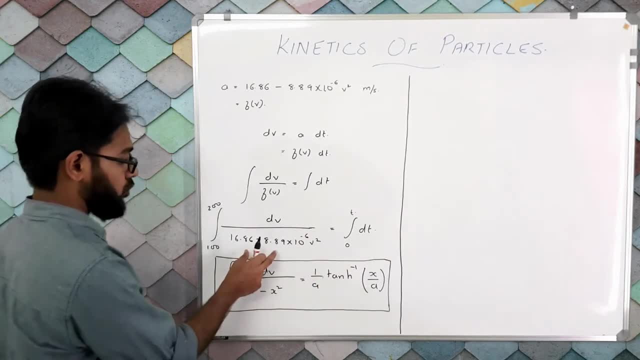 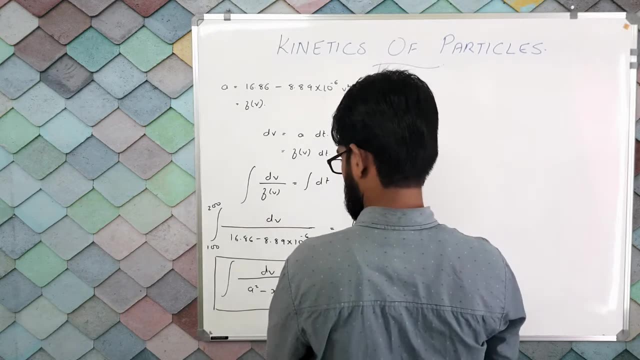 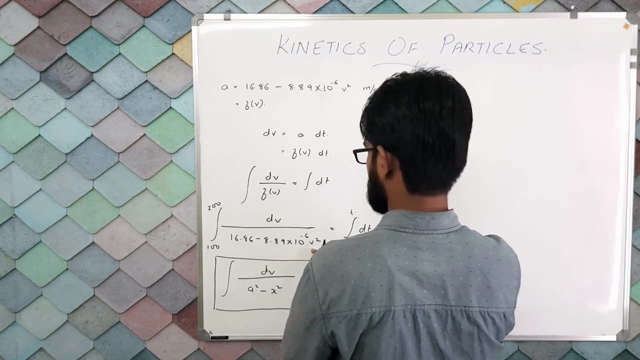 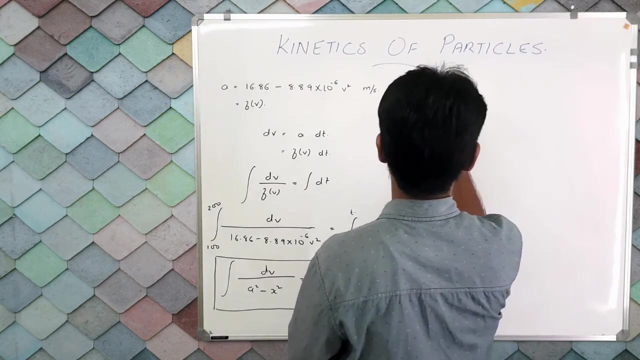 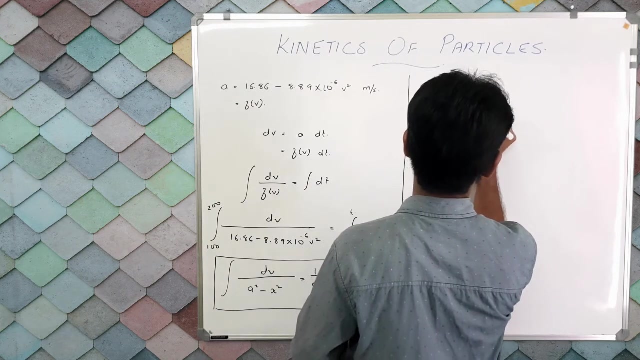 So I express this corresponding integration to this corresponding interaction for this expression in this format. So for that what I do, I take 8.89, 10 raised to minus 6 outside, So this corresponding term will give me T. T equals 1 by 8.89 into 10 raised to minus 6. 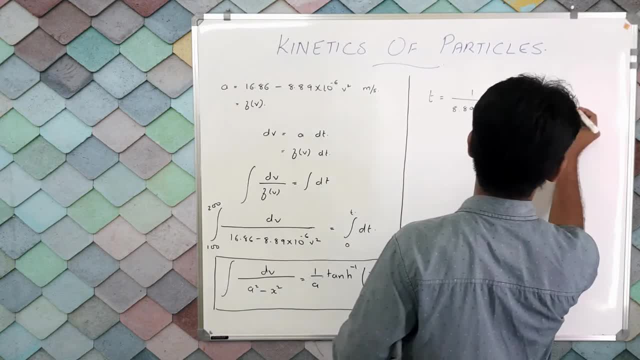 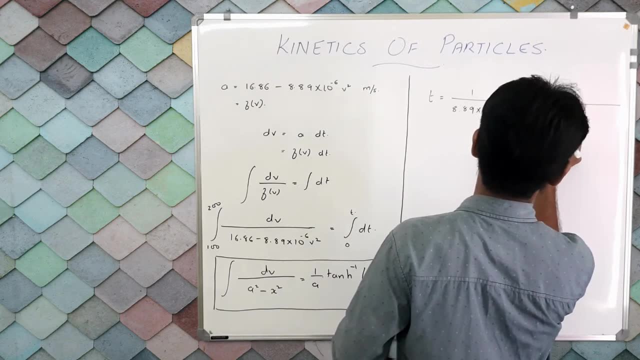 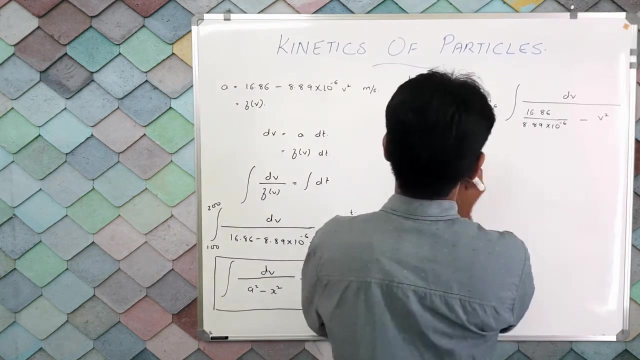 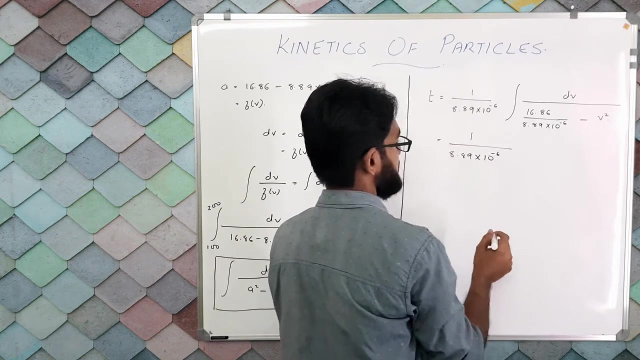 integral dv divided by 16.86, divided by 8.89 into 10, raised to minus 6 minus v square, This will turn out to be 1 divided by 8.89 into 10, raised to minus 6.. This will turn out to be dv divided by: